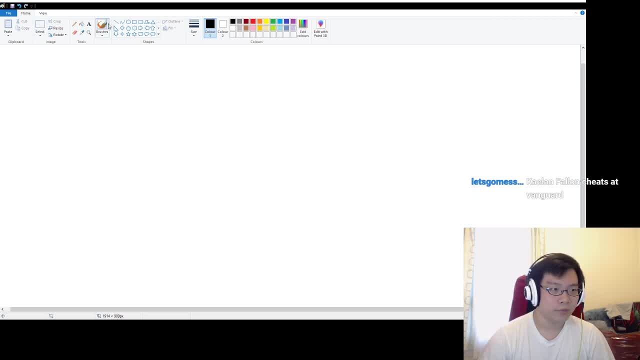 So let me just clean up, All right. So when we get to basic statistics, right, you think of like flipping a coin or rolling a dice, And flipping a coin, as you're aware, is 50-50.. That's for a coin, really badly drawn coin, whatever. 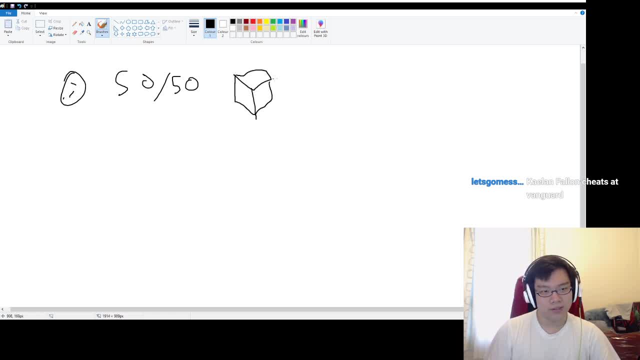 And then you know dice Badly drawn. Badly drawn dice, That's you know, one in six to roll any given number. So to do multiple probabilities at once, there's two ways you can go about it. One is for compound probabilities or one is for 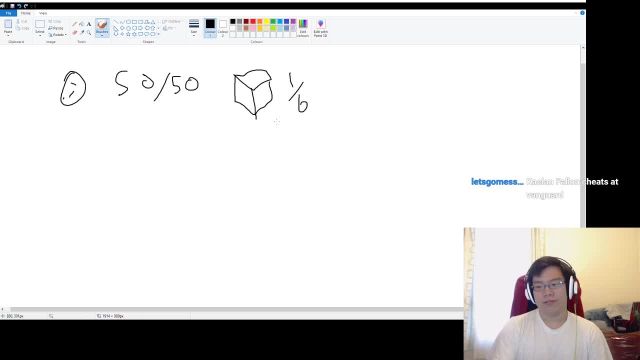 There's a specific word- I don't remember what it was, but it's like you can either have this and that, or you can have this or that. So to illustrate what I mean real quick, this is a really core concept that I'm just going over, just in case you don't know this. 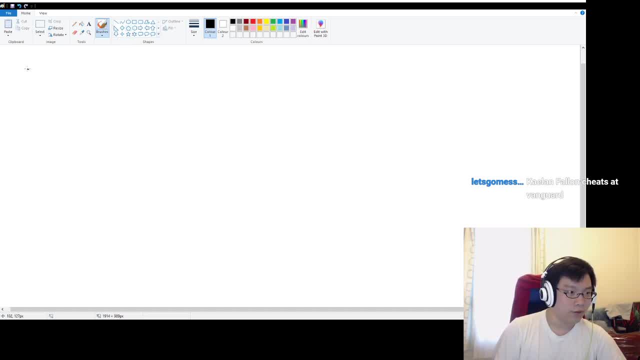 But let me just draw another dice here real quick, One slightly less bad than the previous one. All right, That's a horrible dice Anyway. so the chance of rolling any given number on a dice is one, six, right? So let's say that you want to roll a one and then a two. 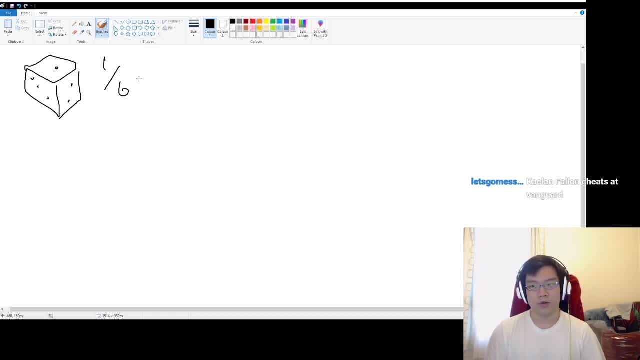 Well, you want to roll one six, followed by another chance of one in six chance. So when you say the word and in probability that means to multiply, So to get any two specific numbers is one six times one six, which is one thirty six. 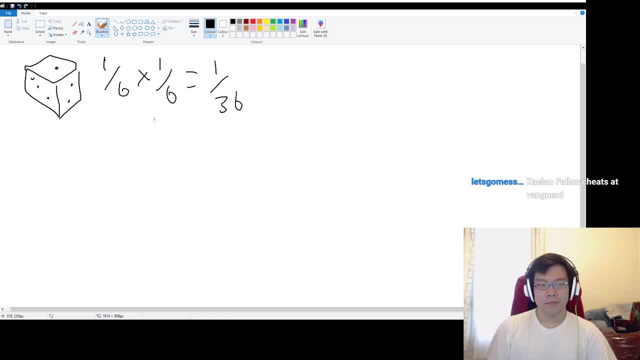 which is some number. It's really low. But then to say that you want to roll a one or a two, so you roll one dice and it can be either of those numbers an, or refers to a plus. So in this case one six plus one six is two sixths, which is a third. 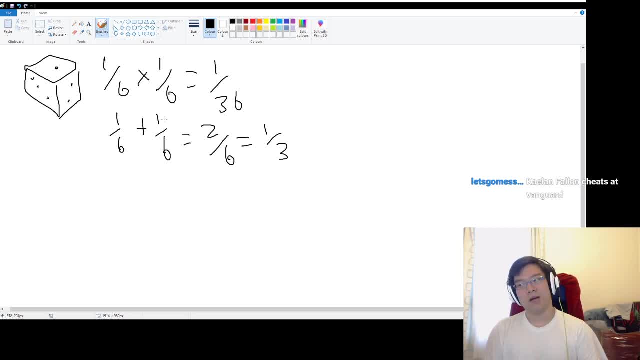 Which makes sense, right, Because one and two combined, put together, make up a third of the dice. So that's the, The absolute, absolute basics that we need to understand. And so the next. So moving on to the actual being card game specific when it comes to card games, 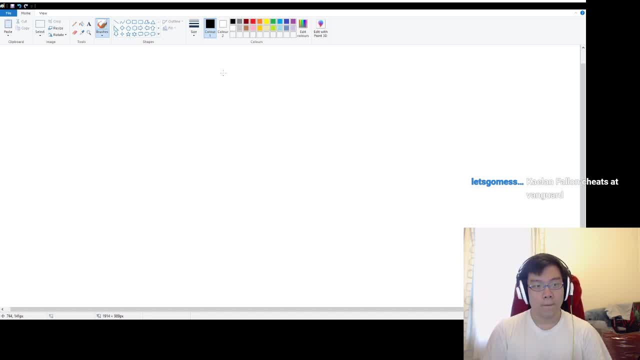 you think of drawing cards off the top of your deck or whatever. This is what we call compound probability, where you have lots of probabilities that stack up one after the other. So, for example, you know if you are drive checking right. 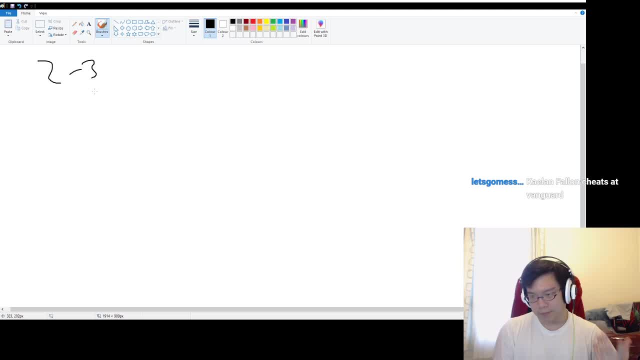 So during a drive check, you look at two to three cards off the top of your deck, depending on whatever your Vanguard is, And you have, you know, some number of cards in your deck. Let's just call it 30 to make numbers easier. 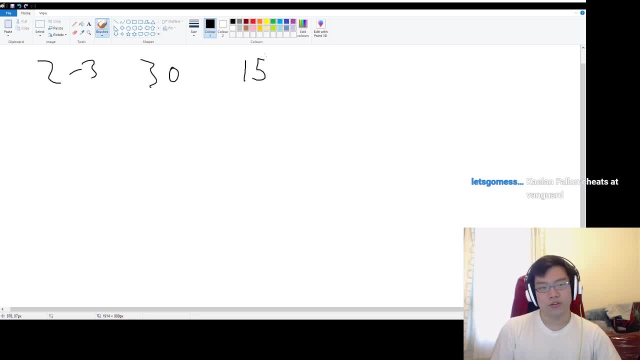 And in those 30 cards. you know there are 15 triggers left in your 30 cards because you are really well stacked and you didn't hit any triggers earlier on. It's so even though 15 divided by 30 is half. 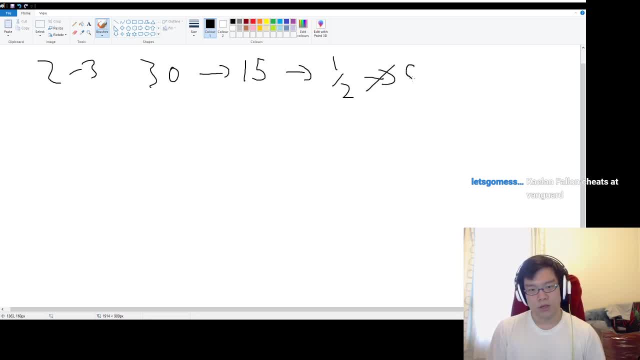 So half of your deck is triggers. That does not mean that you have a 50% chance of drive checking a trigger And that is because each individual card is its own probability checker. And that is because each individual card is its own probability checker. 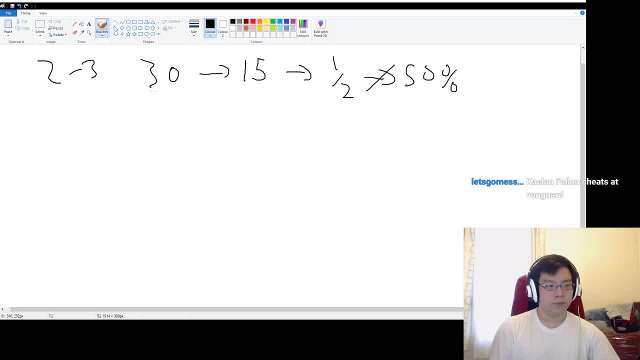 And that is because each individual card is its own probability checker, Kind of, as it were. so what I mean by that is, you know you, drawing cards off the top of the deck is not like. you know, drive checking three times is not the same as rolling a dice three times in a row. 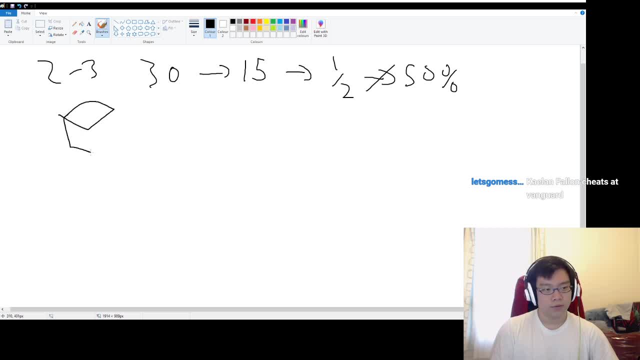 Like the chance of rolling. So when you roll a dice, I'm getting really late at this. So the chance of getting any number on the dice is one-sixth, and it's always one-six, one in six. Whatever happens beforehand does not affect the probability of what happens afterwards. 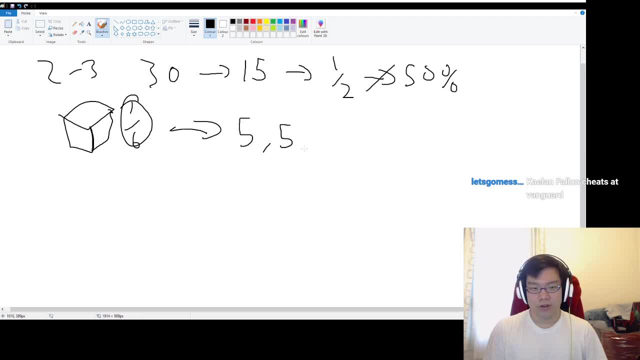 So, like you know, if you roll a five and then you're on another five, five and then you roll another five on your dice, you are still equally likely to roll the fourth five. as you are to roll a one, a two or any other number, It's always one. 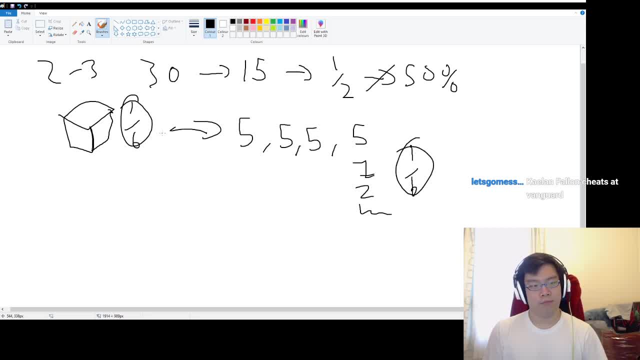 in six. That's because the dice roll is an independent probability, Whereas, compared to Vanguard, you can think of drawing cards at the top of your deck, like reaching to a bag of marbles, right? Let me just quickly illustrate that now. So here we have our bag. 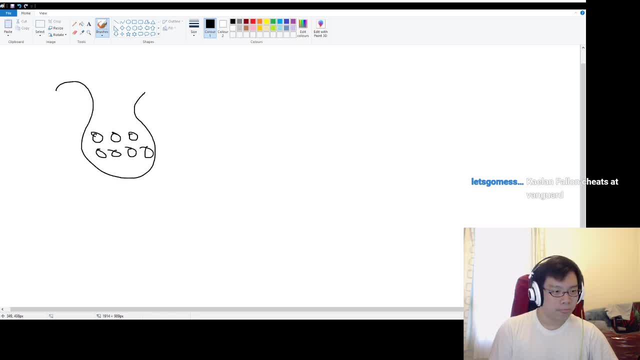 It's full of marbles. So I've drawn 10 marbles here right And we could assume that half of them are black and half of them are white. I'm using black and white because I can't be bothered to change the colour, So when half of them are black and half of them are, 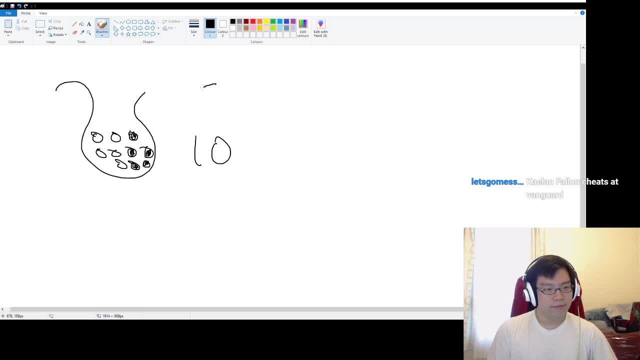 white. we have 10 marbles in the bag, five of which are white, Which means that when you reach your hand into that bag and pull out a random marble, it is a 5 out of 10, half 50% chance. 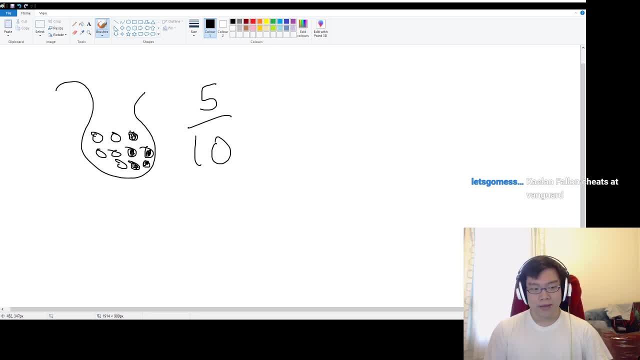 of drawing a white marble. However, once you take that marble and you take it out of the bag- let me just switch the eraser- So if we get rid of this marble from the bag because you've taken it out, the chance of drawing a black marble from the bag is now no longer. 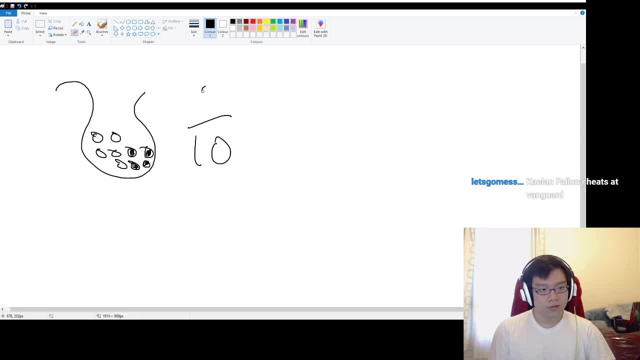 five in 10.. It is now four in nine. So you see that this is what we call conditional probability, where the outcome of one or the outcome of any given trial affects the outcome of your further trials. It's kind of like you know. 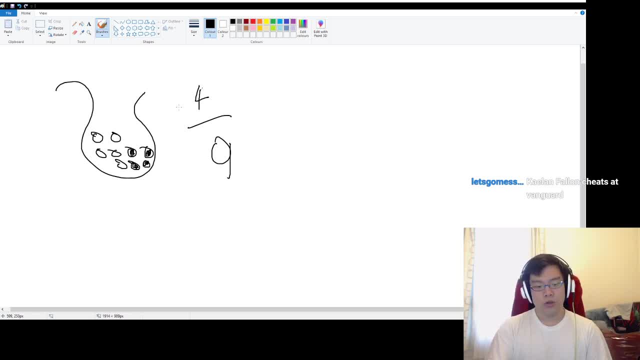 consequences, as it were. So because drawing a card, when you draw a card off the top of your deck, it's a conditional probability because it tells you what the rest of the deck looks like. But I'll be very clear now. This is not how it behaves in real life, Like 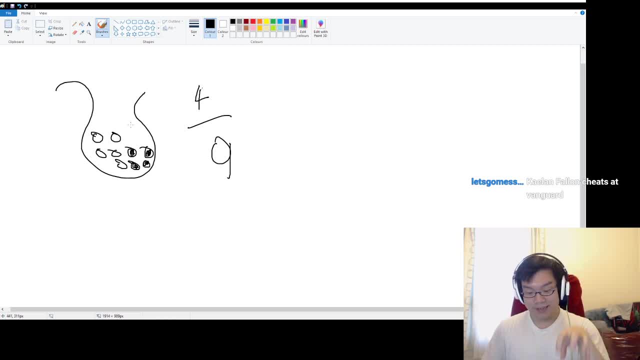 once you shuffle your deck and you put it on the table, your deck is in a fixed order and drawing a card will not magically make the next card a trigger or not a trigger, based on what you draw. So the conditional probability for Vanguard is a very abstract term because 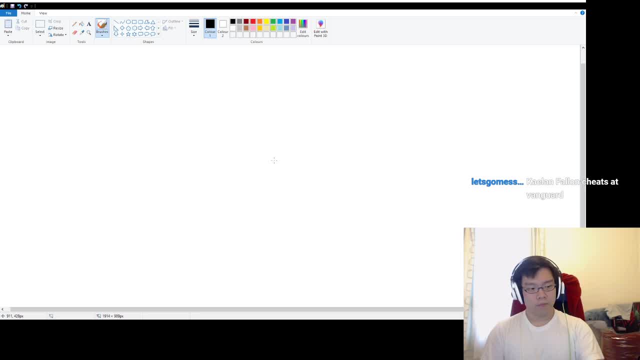 the conditional probability is how we calculate what happens. But it's not what happens is the wrong way of thinking about it. How do I describe this? it's more the way when you shuffle your deck. you set your deck into this very 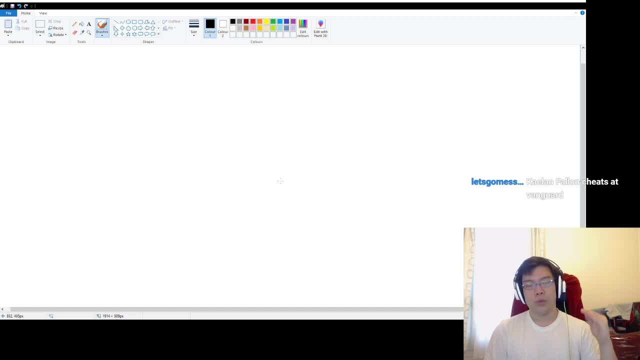 particular arrangement of cards, and conditional probability is how we determine what that arrangement is. So that actually brings me on to the next topic really easily. So the first core concept we need to understand is permutations and combinations. So this isn't really statistics per se. I'm not very good at drawing straight. 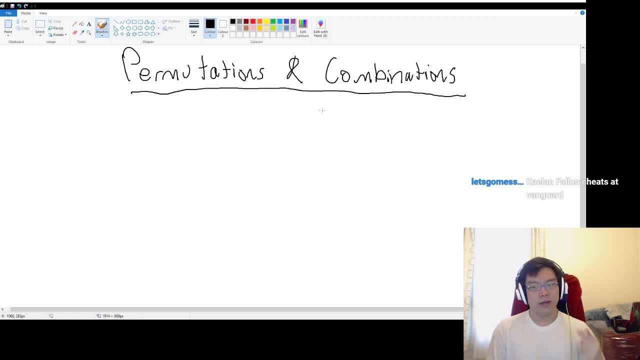 lines. So this isn't so much statistics as it is, set and number theory, but it's going to be relevant for when we actually get into statistics. So a permutation. so actually we'll start with combination first. So theoretically, a combination is what it sounds like. it's a combination of numbers, you know you. 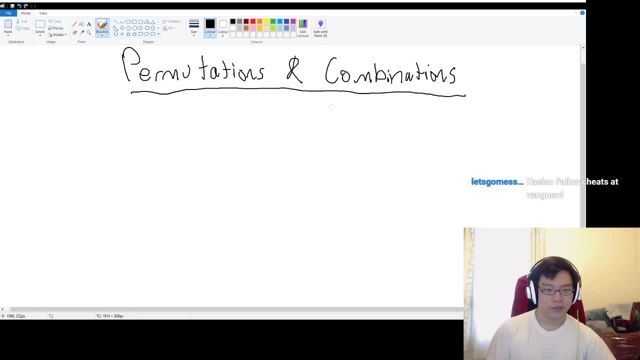 have your combination lock, you have a combination of cards, whatever It's basically. how many ways are there of selecting stuff? So let's say that we have five numbers. We have one, two, three, four and five, right? So five numbers. and I ask you how many ways? 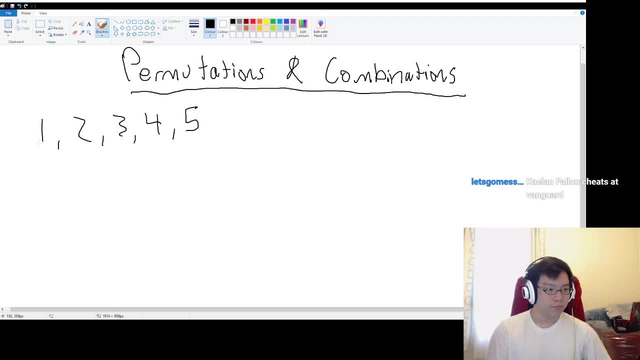 are there of choosing three numbers from those five. Well, we've got one, two, three. we've got two, three, four. we've got three, four, five. we've got one, three, four. one, three, five. It goes. you know, you can do this by hand, we're not going to do it like. 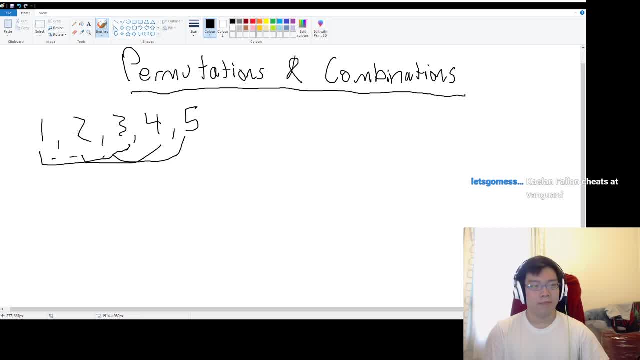 I'm not going to do anything by hand here, I'm just going to explain the theory behind it. but basically you know a com-, so one, two, three. so choosing three numbers from five, you would say, is five, c, three, and that's how many ways you can get combinations of three from. 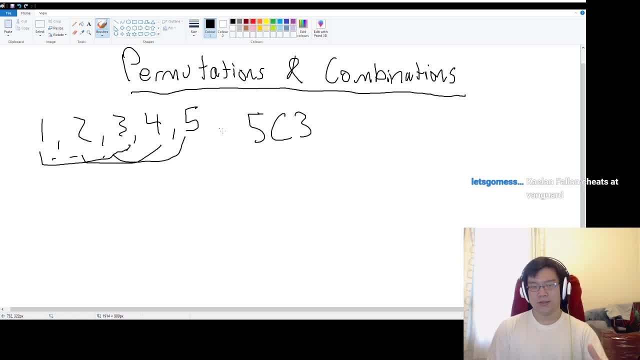 five, And a permutation is basically another step beyond that. so a permutation is basically a combination, but the order matters. So, for example, you know, if you're saying: oh, let's pick three numbers from one, two, three, four, five, you've got. 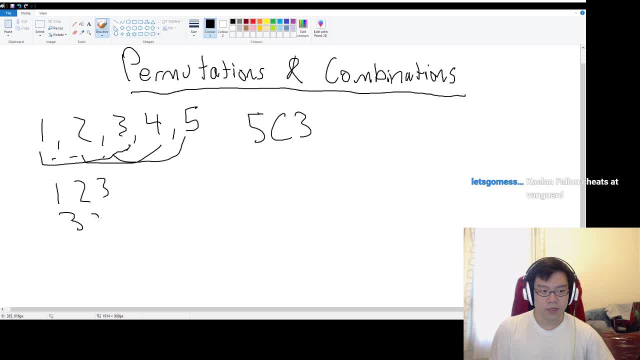 1,, 2, 3,, but you also have 3,, 2, 1,, and you also have 1,, 3, 2.. So you can see that each of these three contain the same three numbers, but in a different order. So all three of these are the. 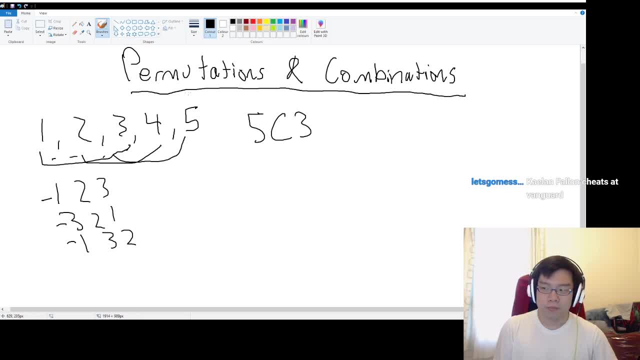 same combination, but they are different permutations of that combination. And to determine permutations you would do 5p3. And that basically says how many ways are there of arranging sets of three from five. So how do we calculate this? Well, it gets a little bit. 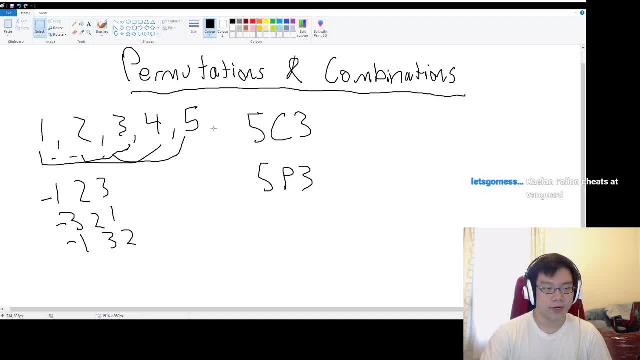 complex, but this is so. this is where we're actually starting some real maths. This is where it gets complex. Let me just get rid of all this for a second and redraw 1,, 2,, 3,, 4, and 5.. 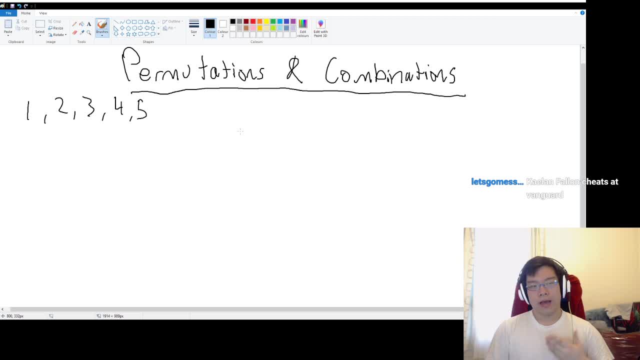 So let's say that we want all five numbers. How many ways are there of arranging all five numbers? Well, for the first number, we can choose any of these five. So we have five options in the first digit slot. Let me just draw these: 2, 3, 4, 5.. So let's say that we pick 5 as the first. 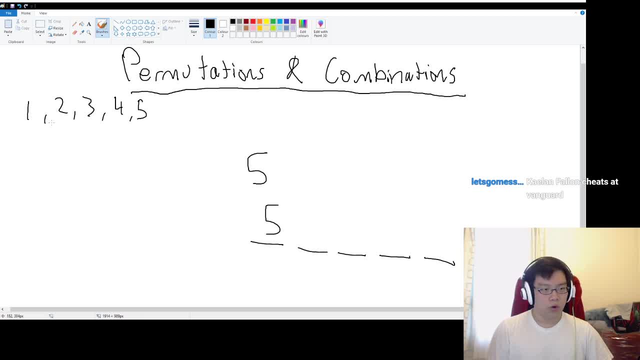 number right. So then we're left with four numbers. We've got 1,, 2,, 3, and 4 left, which means that in the fourth slot we can choose any of these five. So let's say that we pick. 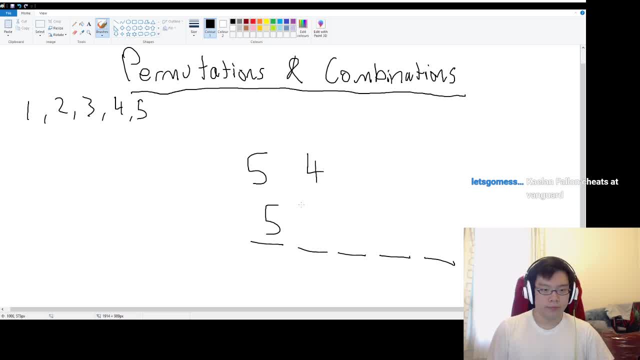 any one of 4 numbers. So let's say that we chose 3.. So we can't use 5 and 3 anymore. So in the third number we're left with 1,, 2, and 4.. So we have three options left for that number. So let's. 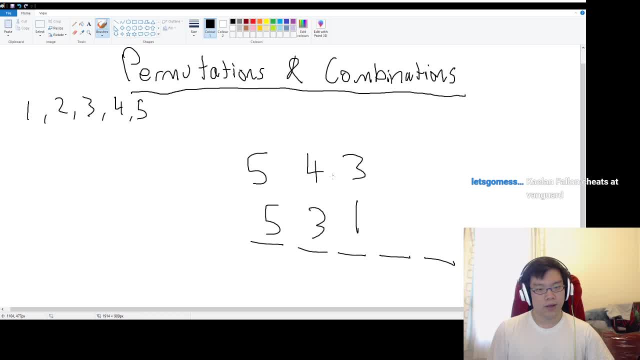 say we choose 1.. Second slot: we've got 2 left, which is 2 and 4.. So we've got two options. We'll choose the 2. And in the last slot, the 4, is the only one we don't have left, which is the 4.. 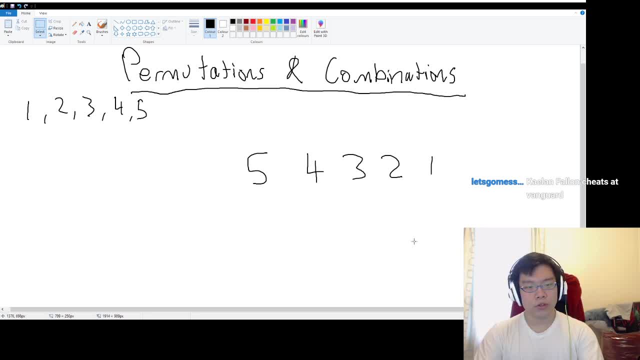 So let me just get rid of that real quick Now. assuming that we were choosing these at random and each of them were equally likely, it stands to reason that to choose any single number out of five numbers, you have a 1 in 5 chance. And then, when we take one of those numbers away, 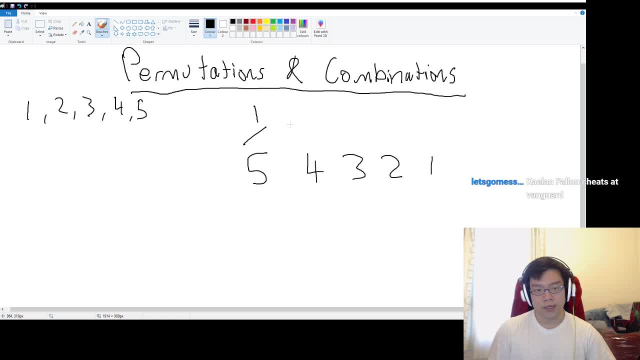 we're only left with four potential options, all of which are still equally likely. We're left with a 1 in 4 chance. So you multiply them, and you multiply them, and you multiply them, and you multiply them. So, before we talk about chance again, 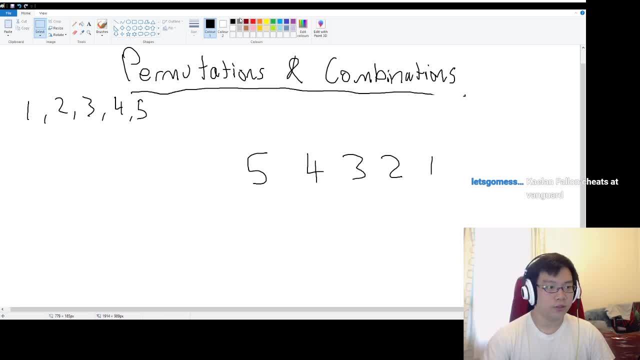 let's go over the fact that you had five options at the first stage, then four options at the fourth stage, and so on and so forth. So the number of options you can get is just times, times, times, times, And there's actually a thing where you can call this. So anytime that you take a number, 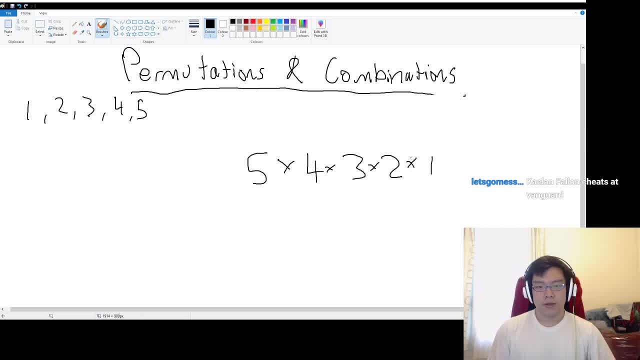 and you multiply by all the other numbers after it, going down in sequence, it's called factorial And we represent that with an exclamation mark. So that's five factorial. Okay, This is actually has a lot of applications beyond just statistics, But this is the most. 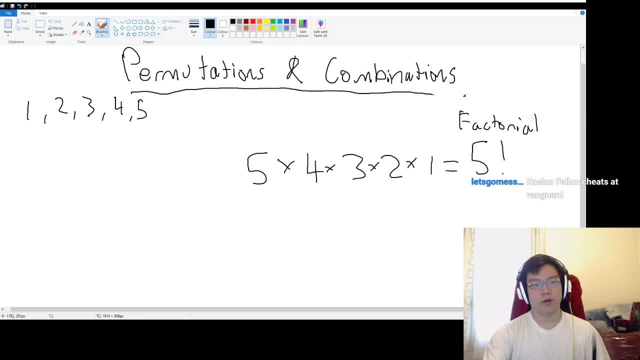 basic application you can think of it for. So now that we know how to represent, or how many ways there are of selecting stuff, we can then expand that further and think of a deck of cards, right? Well, five factorial is 120.. That is correct. So a deck of cards? well, let's keep it easy in terms. 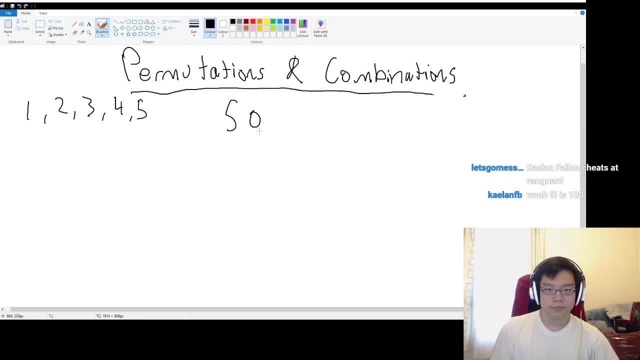 of numbers. So a deck of cards in Vanguard is 50 cards, right? So how many ways are there of arranging 50 cards? Well, it's 50 factorial, which is a really large number that I'm sure someone's going to work on in their calculator. 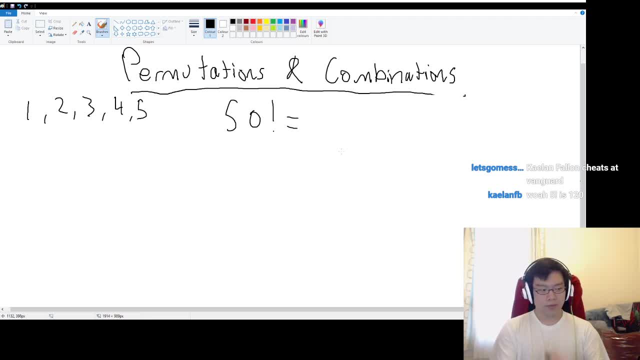 but I'm going to do it right now. But it's basically some really large number, which means that anytime you shop a deck of 50 cards, right? So at the moment the deck is in one. all the cards in this deck are arranged in a very particular order. I can give you the first three. 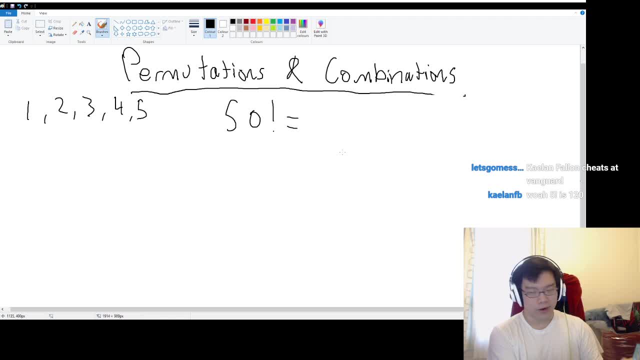 cards are: Morgan row G, unflip crit and grade one booster. right, I can shuffle, shuffle this right now, Recently, you know not, it's not a perfect randomization, but it's a decent randomization. And we look at the top three cards now. top three cards is now: grade one booster draw trigger PG. 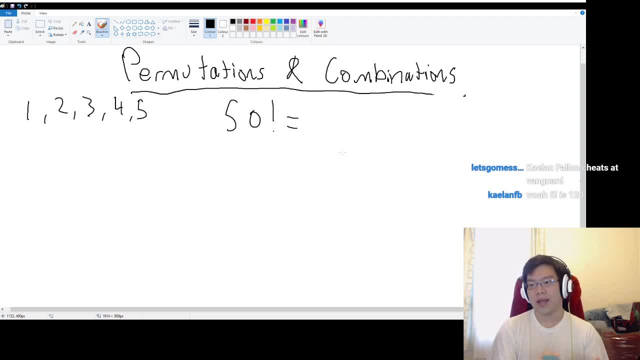 So obviously this will apply for the entire deck, But every time you shuffle the deck you're changing the order that the cards appear in, And which specific cards don't matter. like you know, for example, if you have four heel triggers, it doesn't matter which one of those four heel. 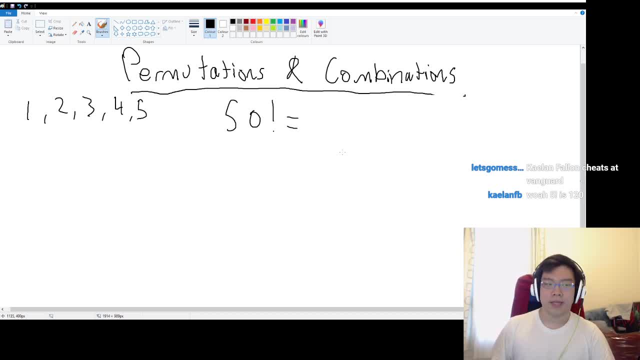 triggers is where, because heel triggers are all the same. It's like having, it's like even the seamless of five numbers we had. instead of having one, two, four, five, it was one, two, two, two, five. So we have three twos there. you can go: two, one, two. 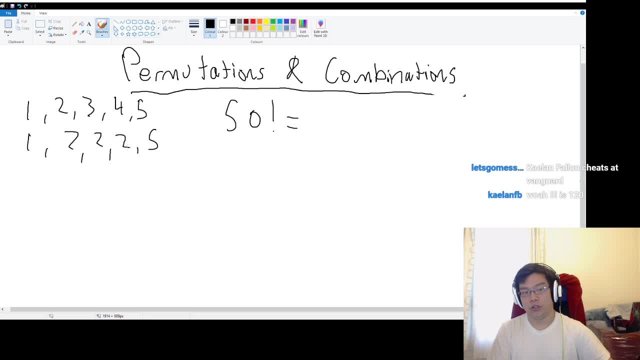 five, two, And it doesn't matter which two is where, because it's still a two. So in this case, we know that there are 50 factorial ways of arranging cards. Therefore, when you finish shuffling your deck and put your cards down for your opponent to cut, you have- let's turn this into an arrow- you. 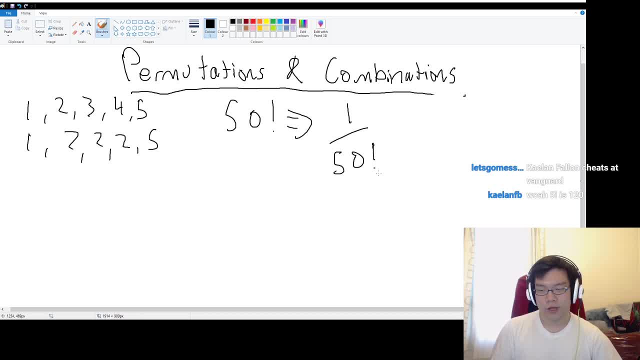 have a one over 50 factorial chance of your deck being in any specific given state. So that's looking at the whole deck. But then how do we look at some cards? Yeah, so yes, if you hadn't started it would be. 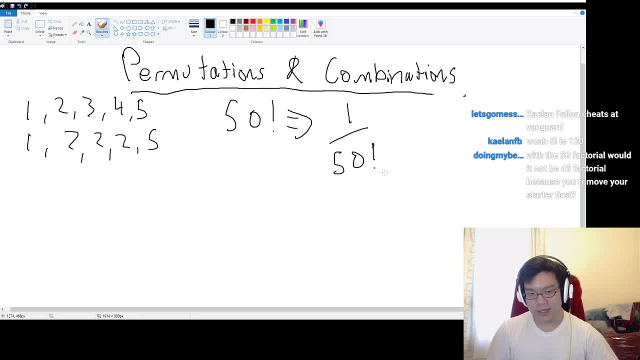 four in factorial. I'm just using 50 as an example to make the number nice, round and easy. But yeah, and when it comes to practical application, it doesn't really matter what the number is. I'm just describing you. In a normal deck of playing cards it will be 53 factorial, for example, or 52 if you. 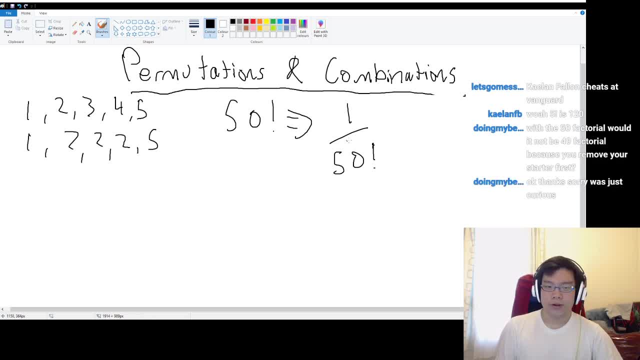 want to take away the joker. So we know that there is this particular chance of your deck being in a given state at any moment in time, Even if you're shuffling in the middle of a game. you know that there's 34 cards in your deck And there are that many orders that your deck can be in. Now, if we 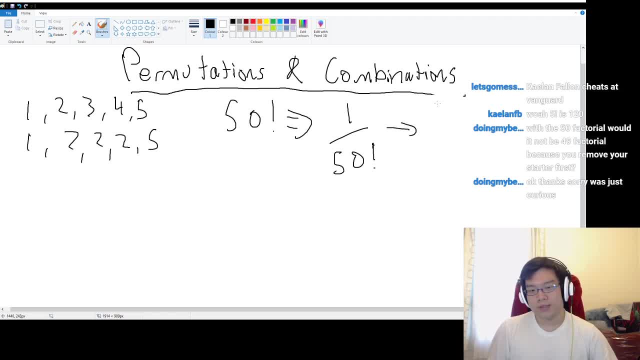 flip the top card and it's a trigger. you know that there's a 16 out of 50 chance of the top card of your deck being a trigger, But, like we said before, the deck state is set in certain ways. So 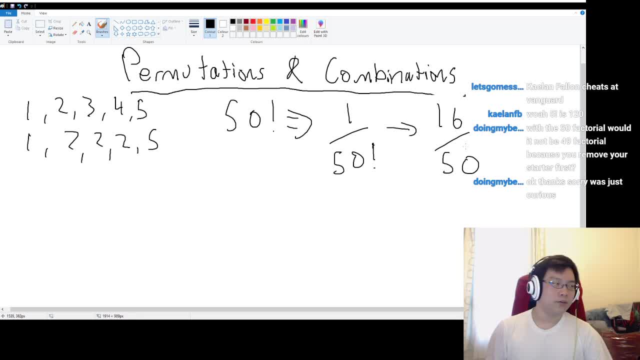 even though you. how do I describe this? Okay, let me quickly calculate what 50 factorial is. 50 factorial, That's 300 million or whatever. right, It's three to the power 64. It's some gigantic number, But basically you have a 16 out of 50. 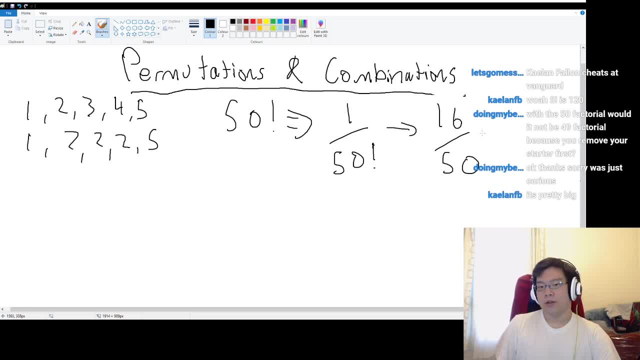 chance of your deck having a trigger on the top. That doesn't mean that you don't know what that card is until you flip it. it means that there is a 16 and 50 chance of that. you chose one of these many billion combinations where the top card was a trigger. so, to go back to the five, 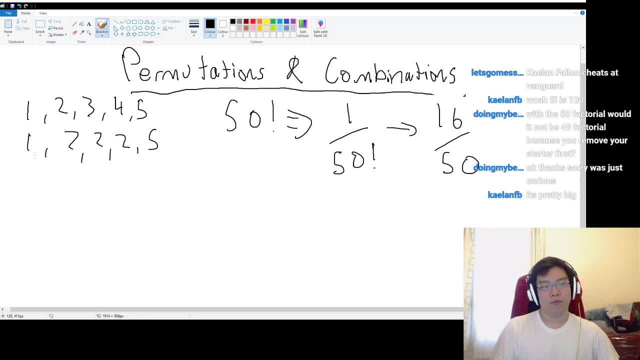 numbers example: right if you count the one as the trigger. so we only have one in five cards is a trigger. right, there are you can go: 1, 2, 2, 2, 5, or 1, 2, 5, 2, 2, or 1, 2, 2, 5, 2 or 1, 5, 2, 2, 2. so we said because 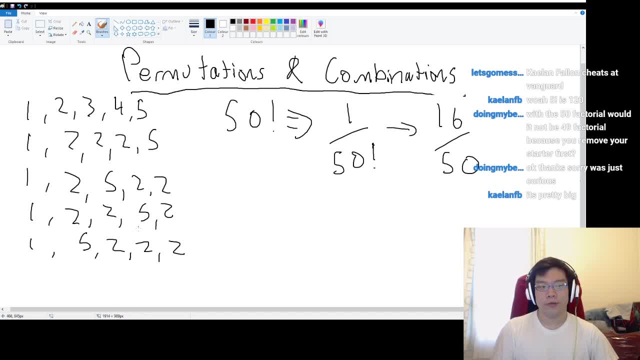 these three twos are all the same. there's only four states. your deck could be in where the one is on top any other. you know you can swap these two twos around. you swap those two twos around around, but in reality they're the same combination or permutation, as it were. 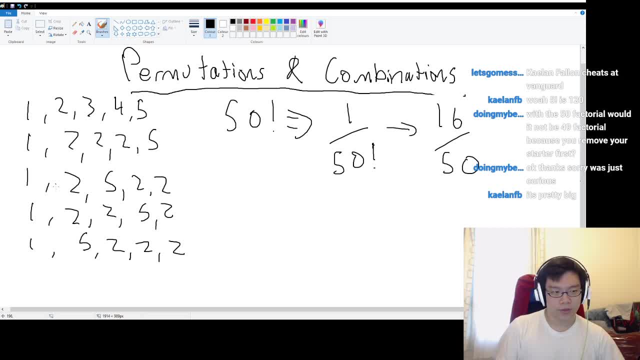 because these are all the same combination. so there are four permutations- whether that could be on top and then. so these four are the subset of the very, many, many permutations there are of one, two, two, two, five. so by knowing that this is the biggest number, you have to work with you. 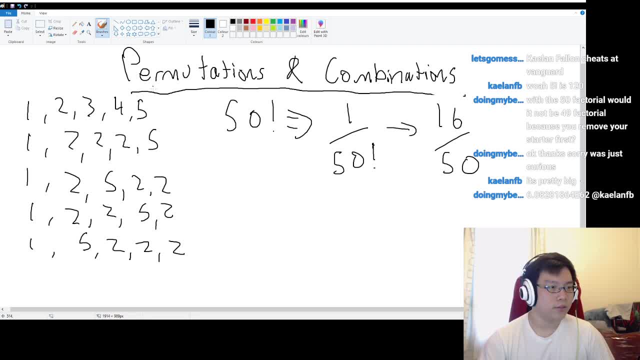 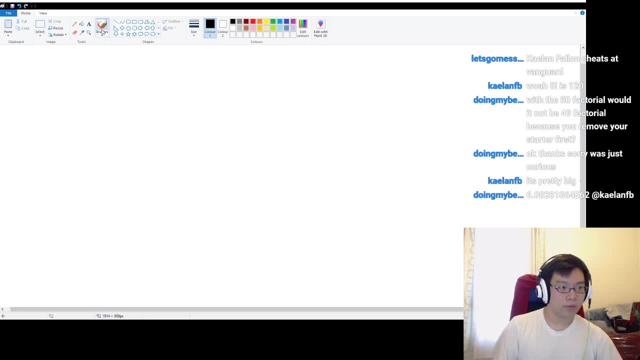 can then interpolate and cut it down. so let me just clean up for a second, just make it easier. all right, so if we're looking at the top four cards, right, so, the first top card being it. so let's go back to 50 card deck. so we have 50 card. 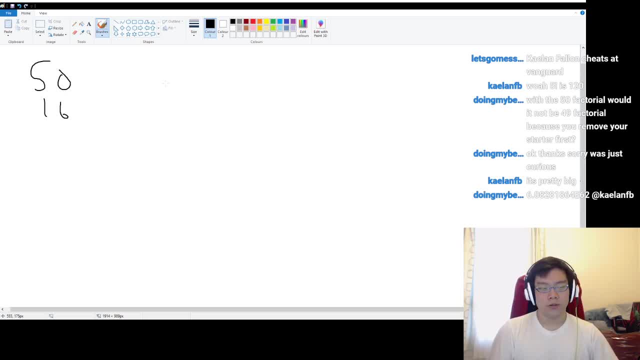 deck. 16 triggers the chance of, in fact, you know, let's assume it's not even a deck, let's assume it's a bag of marbles, to keep it really truly random, the top the first choice being what we want- a success, as we'll call it- is 16 out of 50. 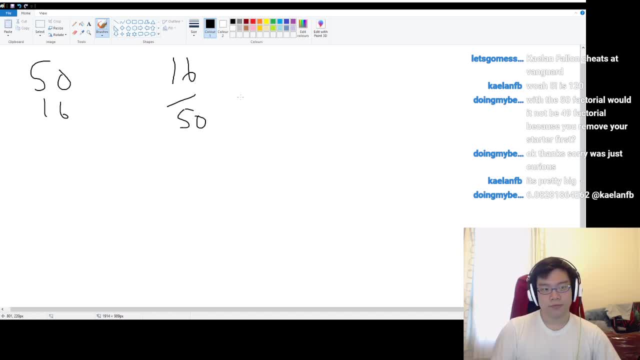 you know that's what we want. a success, as we'll call it, is 16 out of 50. now, if it's success, then the chance of having a next one also be a success becomes 15 out of 49, because we've taken away a success from the pool. if this is, 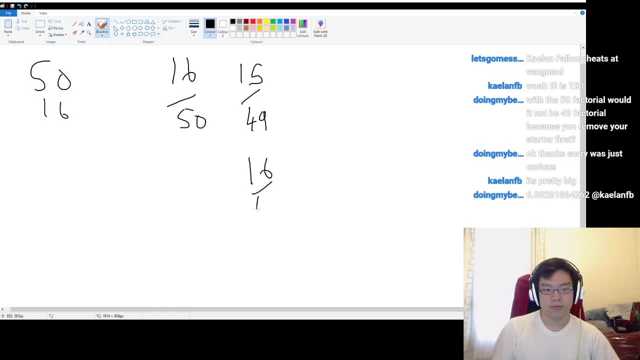 not a success. instead it becomes 16 by 49, because we've taken a failure away but we haven't taken a success away. but for now let me just get this and let's look at only successes. so if we keep going and we keep hitting successes, we get to 14 by 48, and so on. 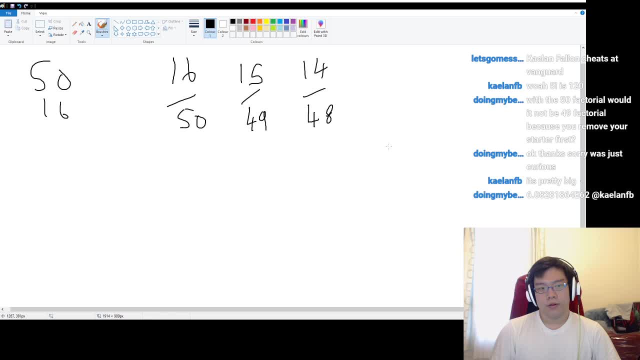 and so forth. now you'll notice that these are both going down. if we just look at the bottom side for a second out, let's ignore probability, let's look at just the top side- you've got 50, 49, 48 and 47, so on, so forth. now, if we follow- 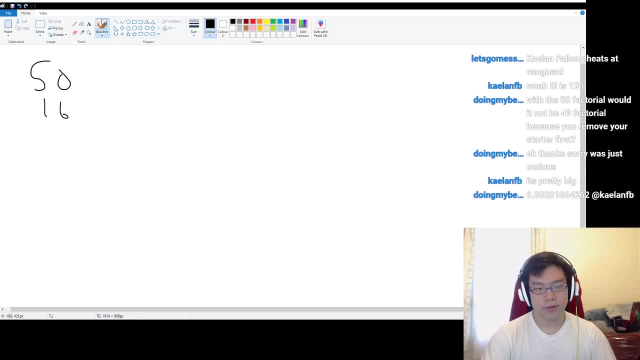 that trend. let me just go before that. you'll remember that it looks like a lot like 50 factorial, which is the number of arrangements we have now. let's say that we only want to take the first three items. so how many ways are there of arranging the top three cards of a? 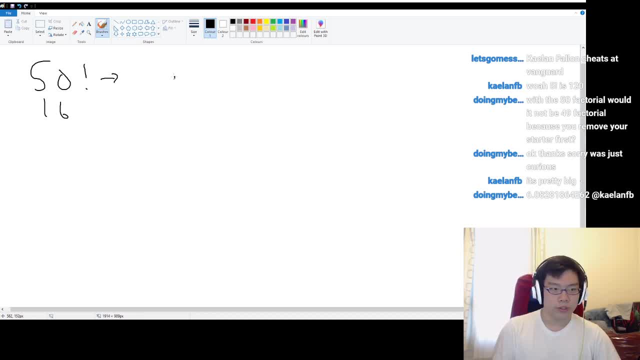 deck, for example. well, again, we're still going to go down, which is 50 choices at the first card, then 49 choices at the second card, then 48 choices at the so on and so forth card. then we just want to stop there. so this is, you know some. 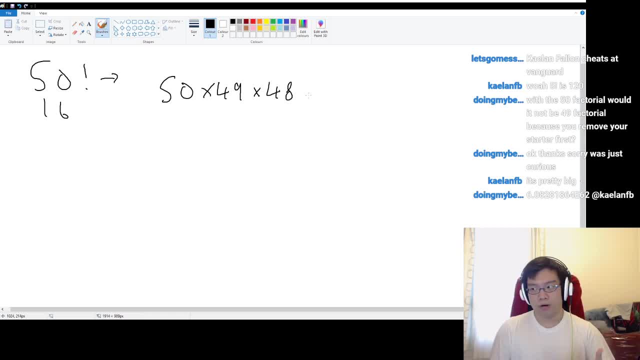 number you can calculate very easily yourself and that's how many arrangements there are of choosing three from the top five, from 50 or whatever. but we can expand this further because if you think about right, if you just write, let me just continue all the way down to times 3, times 2, times 1, so it's. 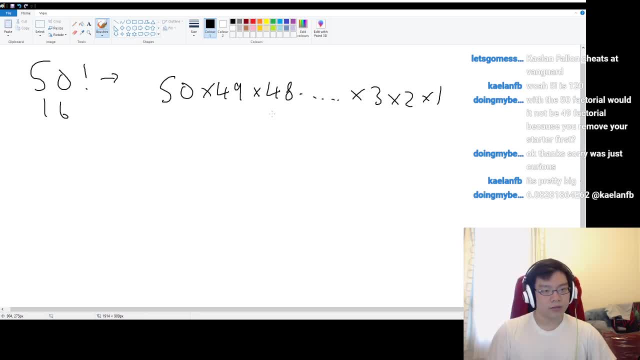 not all the way into middle here, right? if I write 48 times 47 times, 3 times 2 times 1, this is 48 factorial, right? this is 50 factorial. so if we only wanted to look at the first two, how many ways are there? 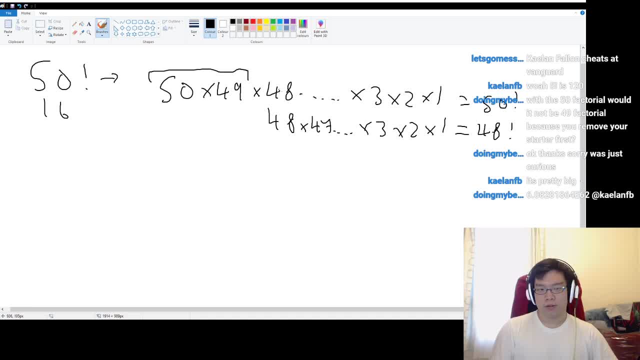 of ranging the top two cards, we can see that the rest of all these will cancel out and, as it so happens, 50 minus 2 equals 48. so what we've accidentally discovered here is the deeper permutation equivalent equation, so factorial, shows you the total number of ways of arranging entire. 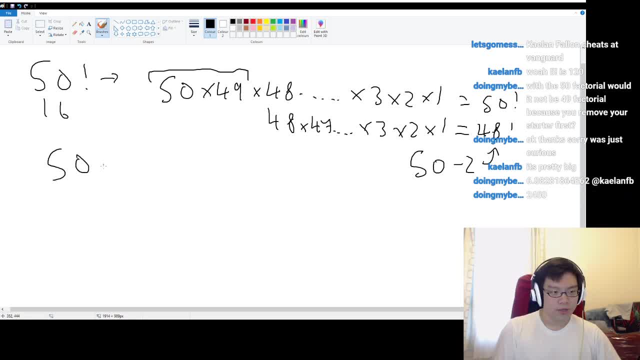 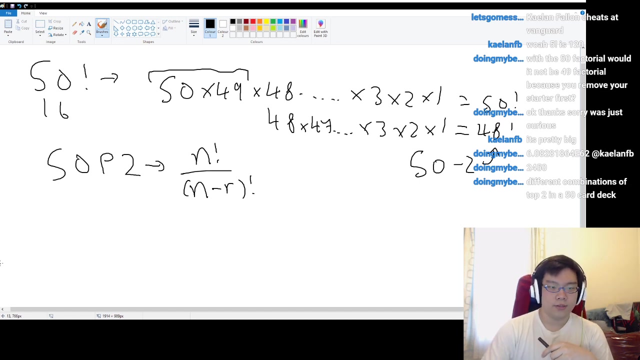 set, but 50 P 2 is number of ways of arranging 2 out of 50 and the formula for that is n factorial divided by n minus R factorial, and that is the permutation equation. so this is good, so this is going to be. this is going to be important later down the line when we talk about the next topic, which is the. 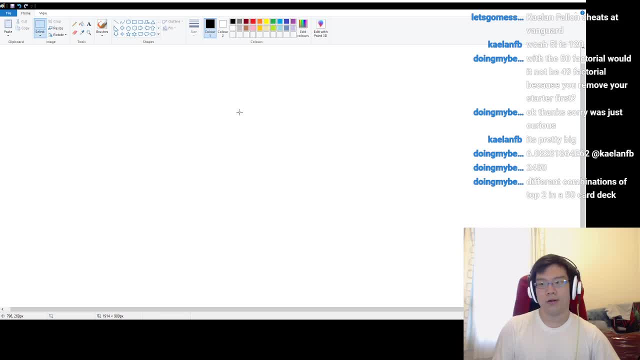 hypergeometric distribution. so this is where we're going to get into some really complicated stuff. now this is where this is the meat of the stuff. let me just write this down: hypergeometric distribution and this is exactly. it's not how we determine what's. 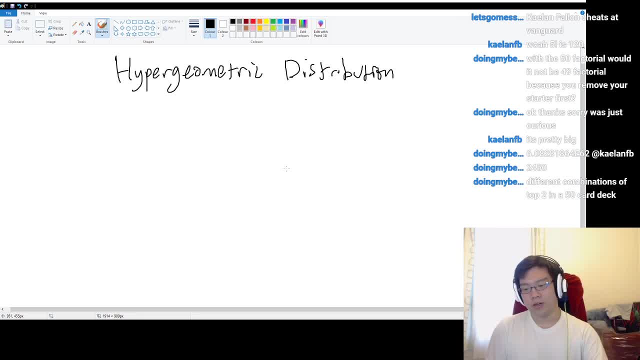 in the deck, like because, I just said, flipping the top part of your deck does not give you information about the rest of the deck. it gives you information about the states that the entire deck could have been in. but the hyper geometric distribution basically states that for a population that contains some 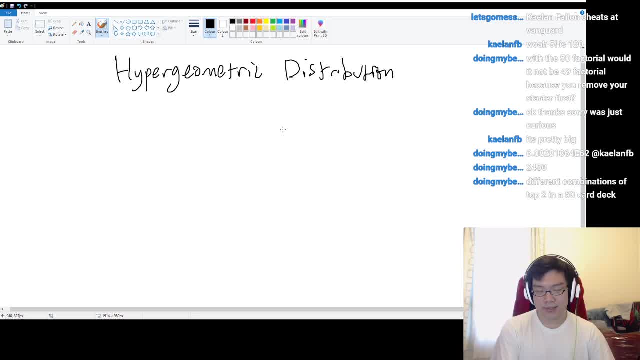 number of successors, with the probability X of that given success. how do we know what's the probability of getting X number of successors? and let me just pull out my notes real quick. there's a whole thing's something that depends. can calculate for this. So the notation is for an individual calculation. so I'm just 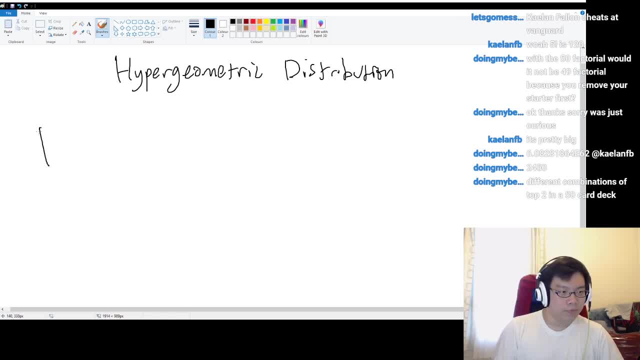 going to write this down first and then explain it. it'll be easier that way. So the probability that your outcome equals some number x is equal to n. big N, x, n minus big X, little n minus little x divided by nn. I forgot to explain combinations. 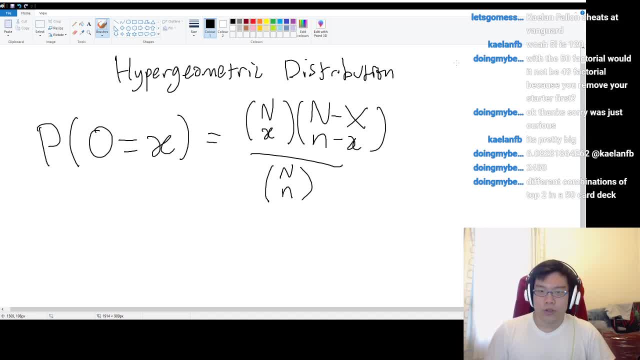 so sorry. let me explain this notation first. So when you see a bracket number on top, number on the bottom bracket, that is for hello, where's my pen? for choose two. Combination is slightly different to permutation. You know what? let me just. let me just rewind and explain that. 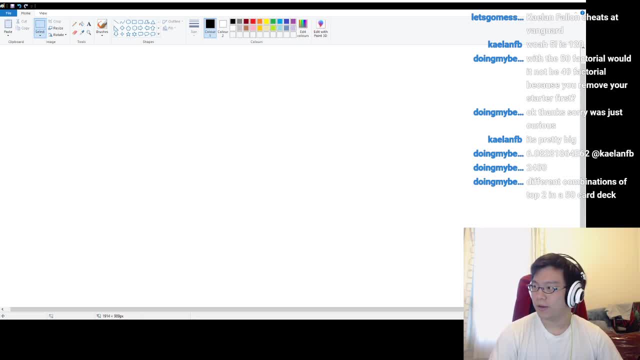 all together All right, so we've learned, all right. that was my bad, I jumped ahead a little bit too much, So we've learned that p, p, which is the number of ways of arranging stuff, is equal to n. 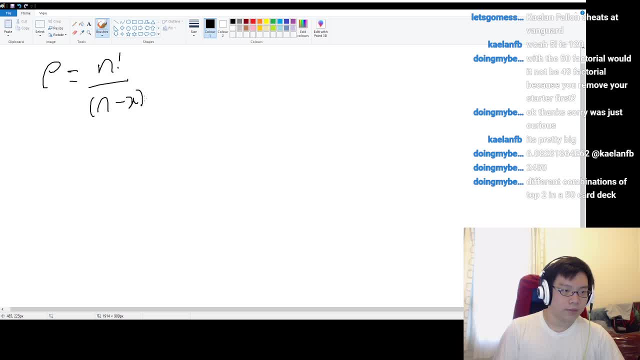 n factorial over n minus x factorial, where n is the total number and x is the target number. So combination, as we've explained, is an expansion of permutation, because permutation cares about the order but combination doesn't. So to get the number of combinations from the 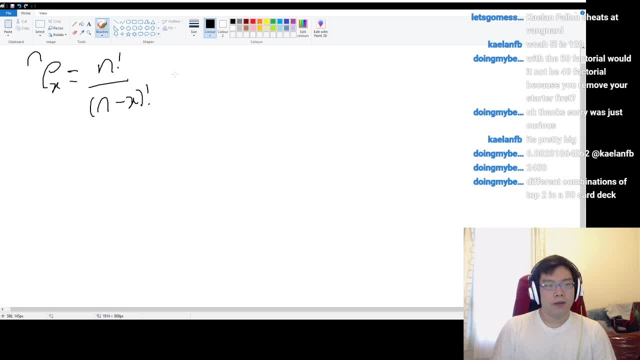 number of permutations is really, really straightforward, because then you just need to divide by the number of ways those things could be arranged. So, for example, back into the ones, you've got 2, 3, 4, 5, right- 3, 4, 5.. If you want to take 3 from them, you've got 1, 2, 3, 3, 2, 1, 1, 3, 2.. 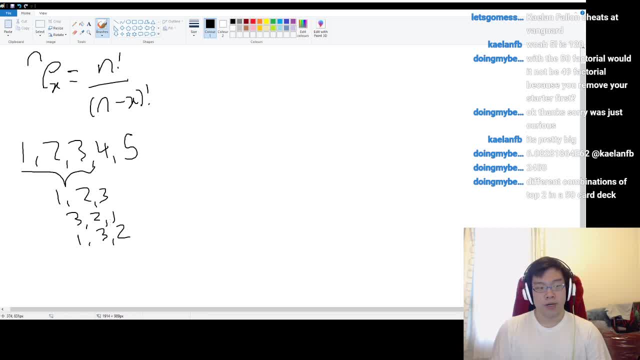 So there are three different ways of arranging three numbers. It's pretty, pretty straightforward. Oh no, there's more than that. actually, 2, 3, 1, 2, 1, 3, I think that's it. yeah, Am I being dumb? Is that it? No, there's 3, 1, 2 as well. 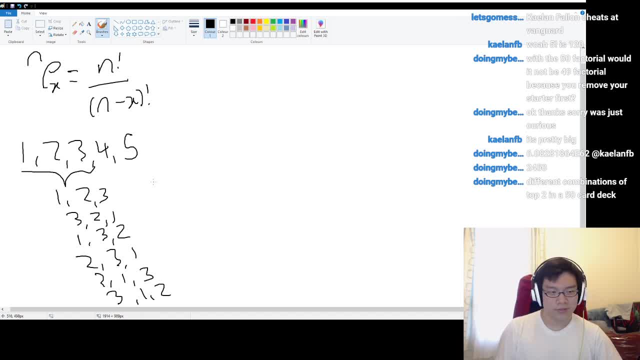 So there are six ways of arranging six numbers? Yeah, I should be right, because obviously, how many ways are they arranging three? Three factorial, which is three times two times one, which is six. So we know there are six ways of arranging three numbers and we know. 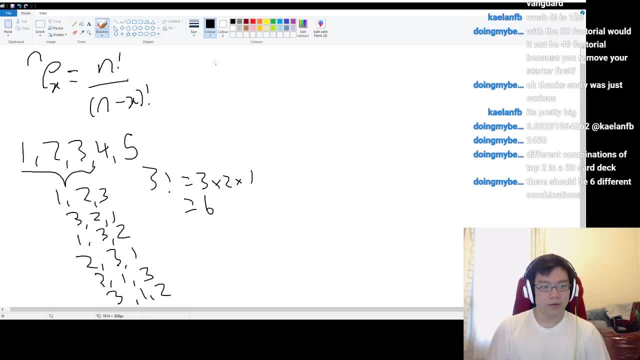 that from npx. if we shove that in, so 5p3 is 5 factorial divided by 2 factorial, because 5 minus 3 is 2. And that's as simple as 5, that's like 5, 5 times 3 times. sorry, 5 times. 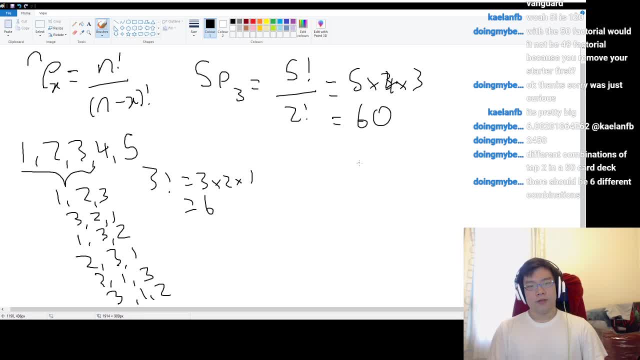 4 times 3, which is 60. So there are 60 arrangements of three numbers within 1 to 5, and that's it. But we know that for every given three, so for every unique combination of three, there are six ways of arranging them. We can then just divide by 6 and be left with 10,. 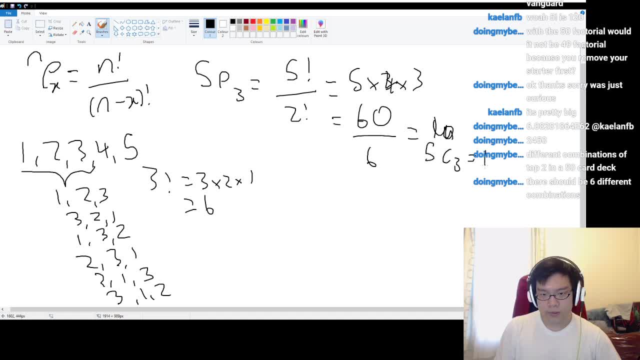 which is sorry. 5c3 equals 10, because we know that there are six duplicates. But notice that we divide it by six times, which is another permutation and which is what we're looking for here. So the combinational calculation is n factorial. 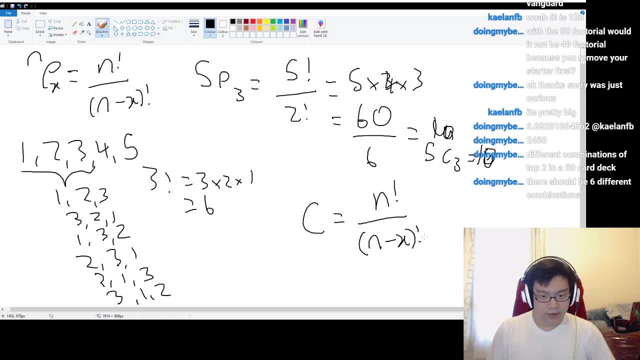 divided by n minus x. factorial multiplied- sorry. further divided by x. factorial for nc3, or ncx. I keep forgetting. you have an undo, I'm so used to doing it on a pen and paper, So that's the other important thing we need to know here, because that's going. 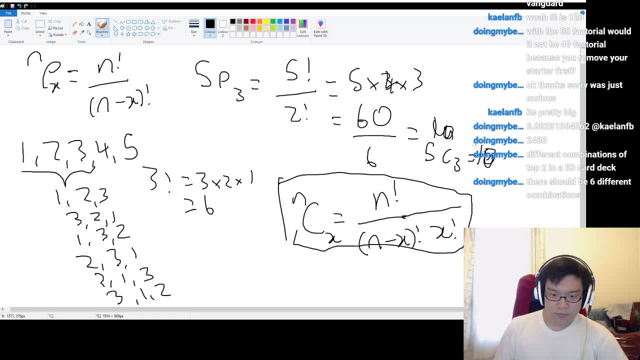 to come up And, as I, the reason I got into this was because that is represented by- and you can kind of see how that makes sense, right? Because you have permutations and you divide the number of possible permutations by them. So you divide by the number of possible. 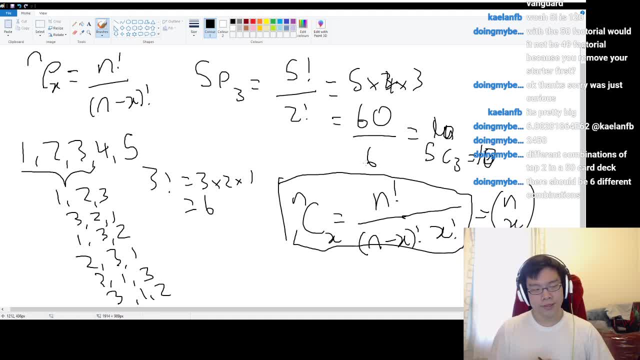 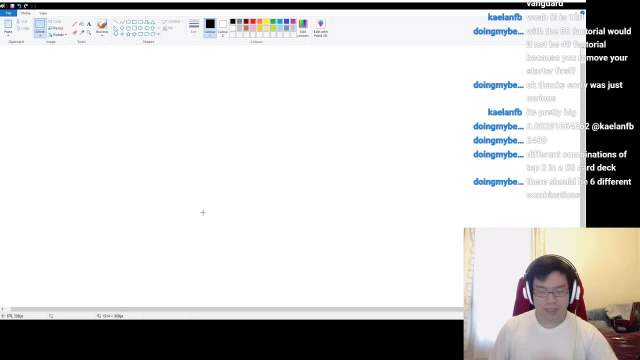 permutations to find out the number of total unique combinations. So that's that. Let me know if I'm like going too fast or if you need me to go back and like re-explain anything, I'm happy to do that. So back to hypergeometric. 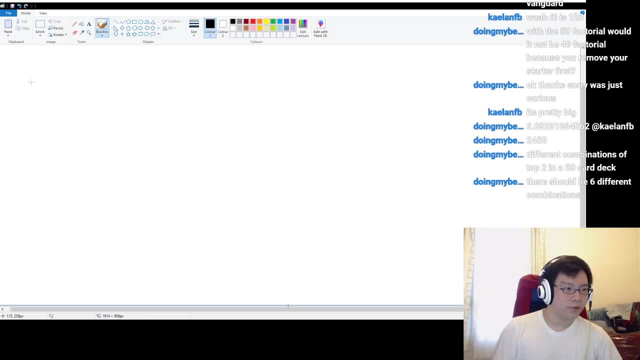 So probably. So the probability that O equals x is equal- to bring my notes back up again because I minimise them, because I'm stupid- is equal to big N over x, big N minus big x, little n minus little x over big N, little n. 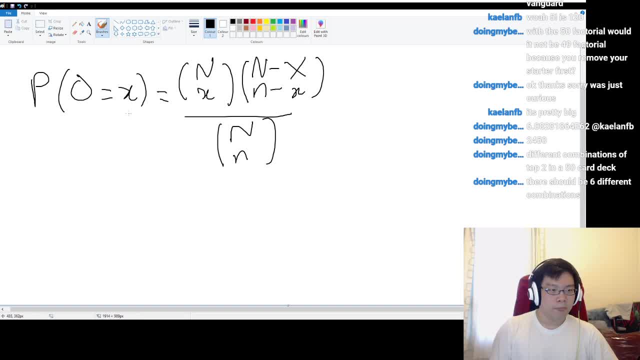 And in this. so I'm going to write that down first and then I'm going to explain it. So, as we said, x is the number of successes we want. Number of successes N is equal to the total population. So in a deck of Vanguard cards that would be 50.. 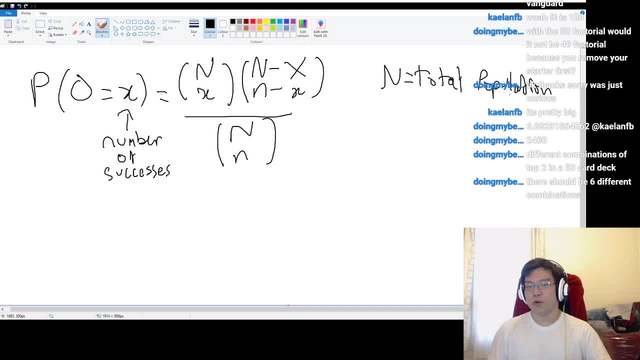 Yeah, I'd say 50.. I'd say 50,, 3 per cent, 50.. 50?, 50 or 40, I don't know what. have you in a starting example, Little x, as we've seen. number of successors. 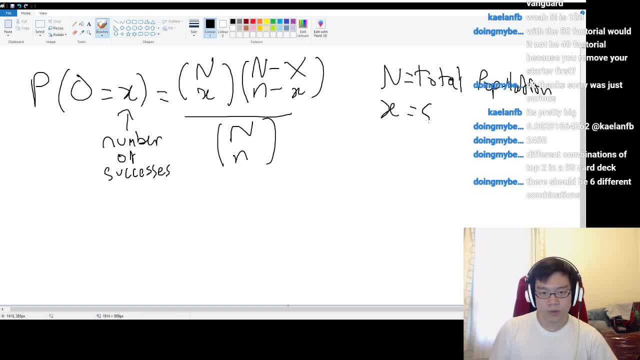 Let me just write that here, so it's all in one place: Equals successors. Then we've got big X, which is the number of successors in the population. So we'll call that population success. So in the case of Vanguard, in a 50-card deck where n is 50 because it's total population, 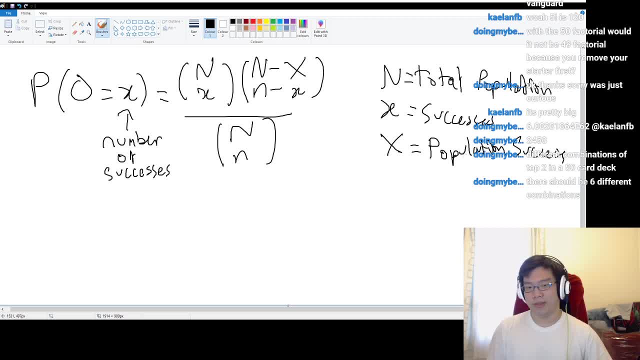 the number of the big X, the population of successors of triggers in the deck, is 16.. So there are 16 total triggers in the deck, of which the little x that we want to find is 2,, 3, or whatever have you. 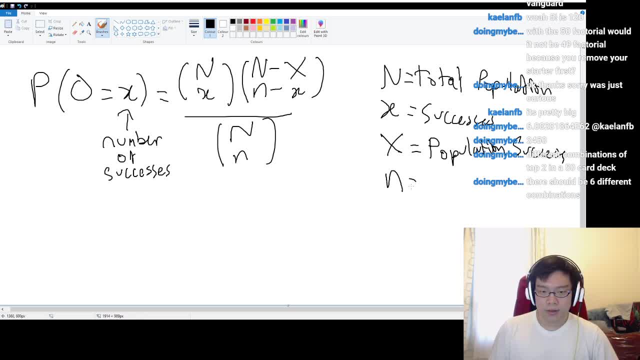 And then little n is number of trials. So how many times are you doing the test? So again to relate to the Vanguard, for example, n would be the number of drive checks. you do So in a 50-card deck with X many drives with X many triggers. 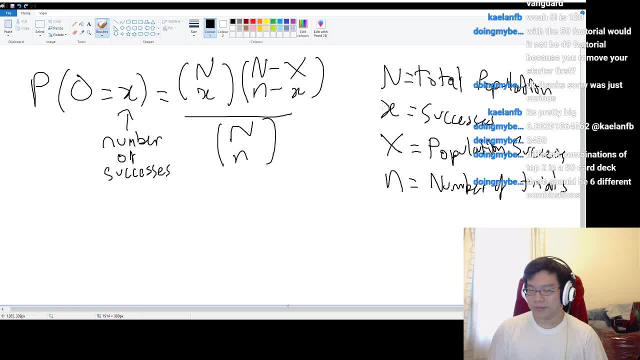 what's the chance of seeing X number of successors? Are you with me so far? This is like the very basic application for it, Or, you know, in like an opening when you start the game: 49-card deck minus a starter opening. hand size of 5.. 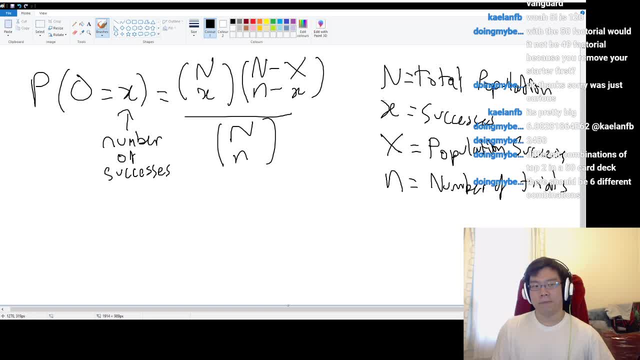 You know there's four domains in the deck. What's the chance of finding one domain? You know what? let's do that right now. So you know that this is. this is represented as C, which I'll calculate separately. So we have a 49-card deck. 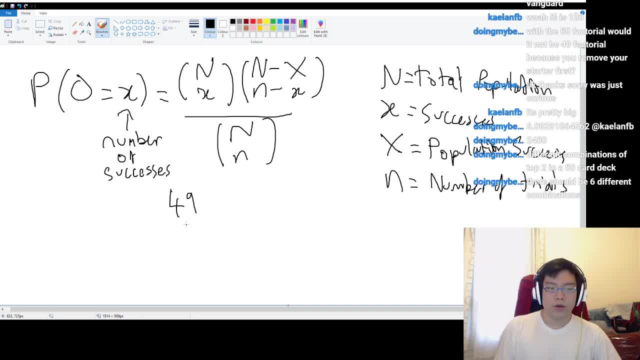 And we want to find- at least we want to find- one domain. So 49, choose 1.. So that's 49.. How many domains are in the deck? Well, we know there's four domains in the deck. How many cards are we looking at? 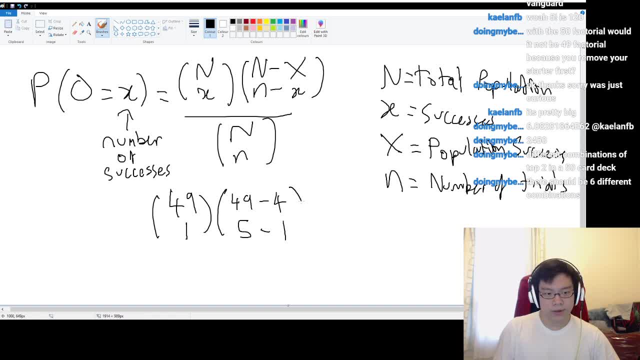 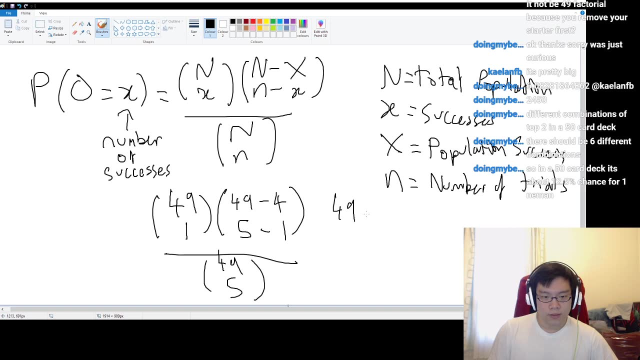 Five card opening hand, minus the one domain you want to find, divided by big N, which is 49,. divided by number of trials, which is 5.. So this is 49C1, which is equal to- I'm just going to calculate this. 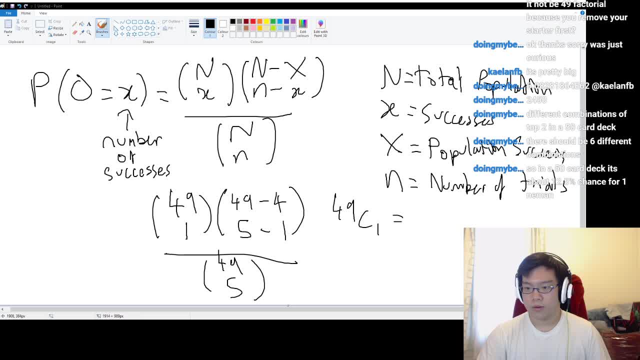 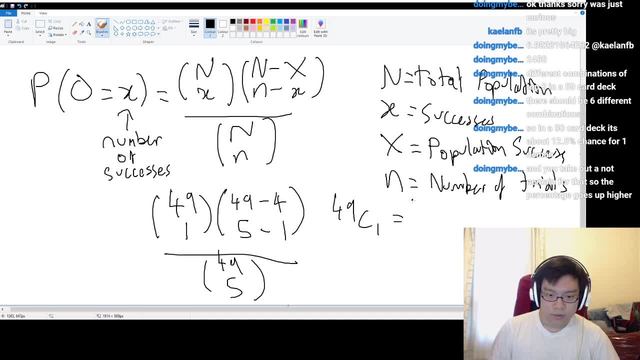 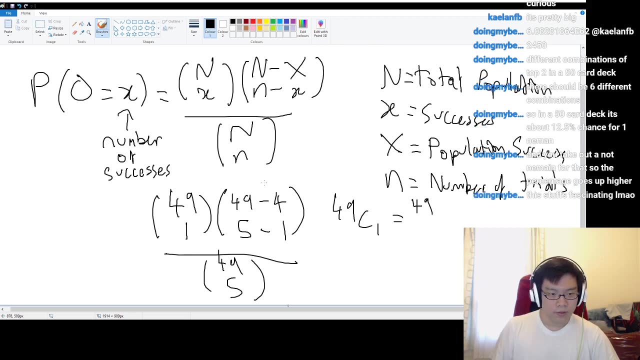 49, choose 1.. It's equal to 49.. I'm running out of space here, especially on my tablet, So 49 minus 4 is 45 and 5 minus 1 is 4.. So we need to do 45, choose 4.. 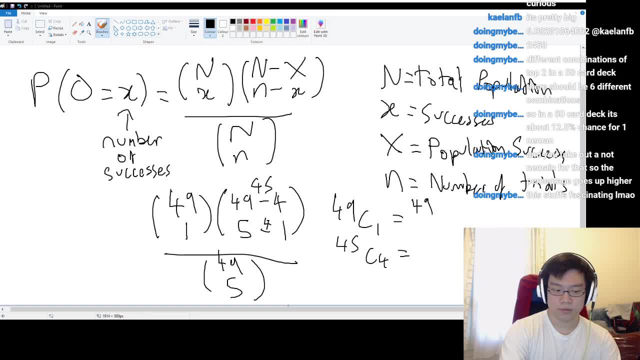 This is going to be a much bigger number. I can feel it. 45 choose 4 equals, come on, Wolfram, 448,995.. And finally, 49 choose 5. Which is 1,906,884.. So you multiply. 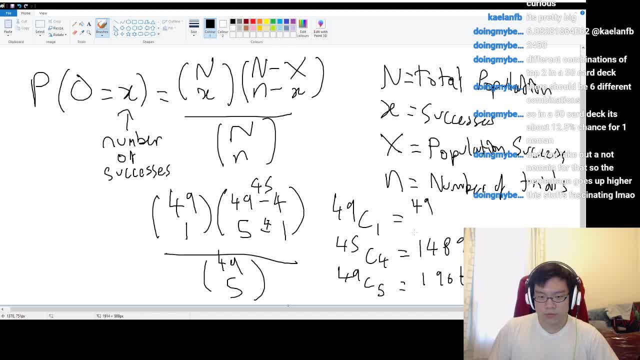 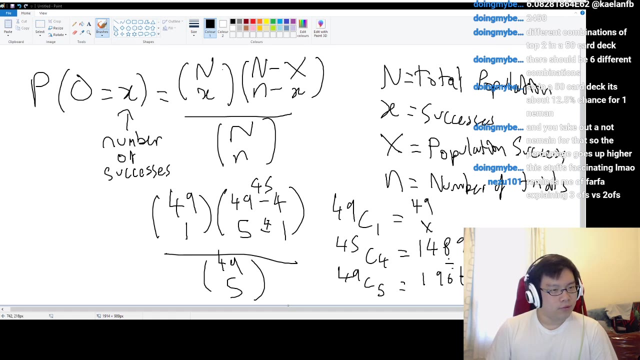 So you multiply. You multiply these two because that's what numbers together in a fraction means. So you've got 49 times that divided by that, which is 49 times 148,905 divided by 1,906,884.. Did I do something wrong here? 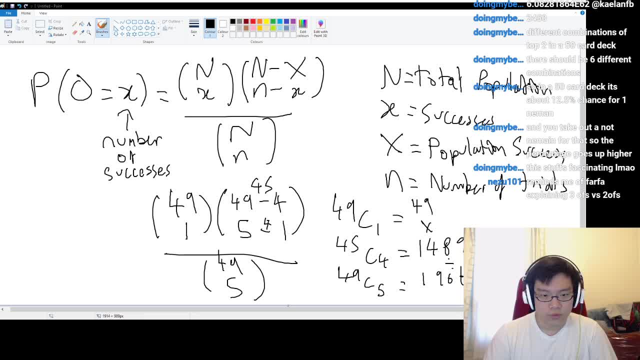 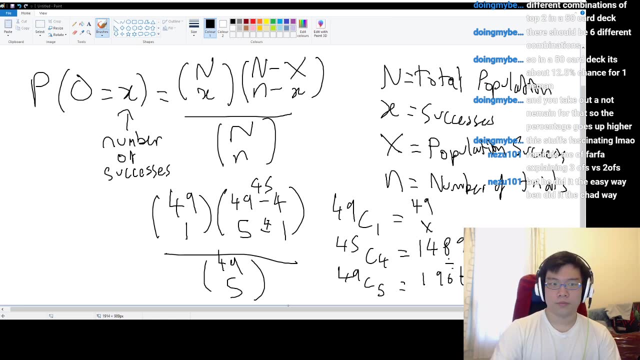 Should be way smaller. What the hell? 49 choose 1, 45. It reminds me of Farfetch'd playing three offs versus two offs, Kind of like that. Have I done the numbers wrong? 49 choose 1.. 45 choose 4. divided by 49, choose 5.. 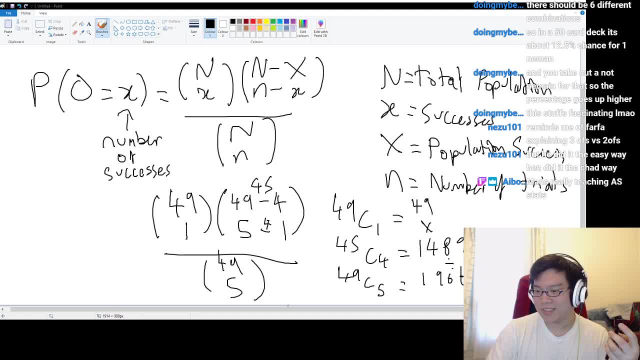 I think I might have written this down wrong. Hang on, Man's really teaching AS stats. Yep, He did these way, he did it the shadow way. Have I written this down wrong? There's a good chance I might have written this down wrong. 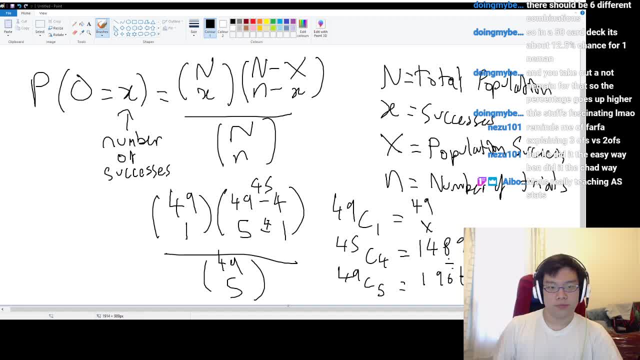 Right, I know shit. See, I've edited everything now. Oh, The next one too. Next, we have probability. is that Existence in the population? I have written that down wrong, Okay, Yeah, Okay, I've done a little bit of a steep in here, but that's fine. 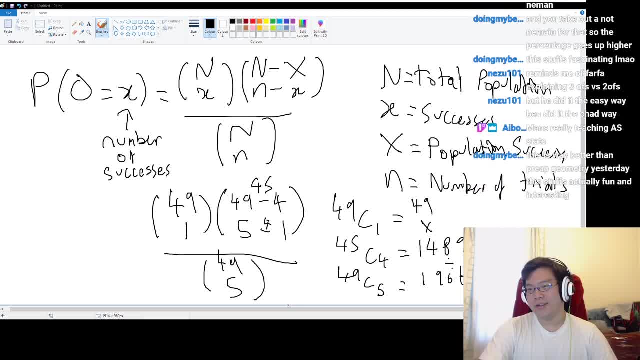 Nothing We can't, Nothing can't fix. that's why, very fortunately, I had something else prepared, which is, instead of doing so, instead of doing this by hand and making a mistake like I did, there's a website which someone's built- a literal website- to engineer this all for you, so let me just bring that up on the screen. 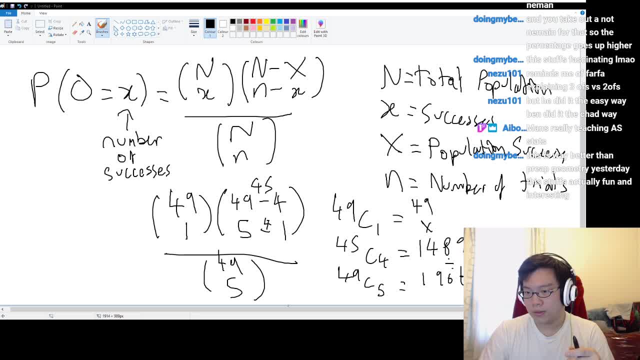 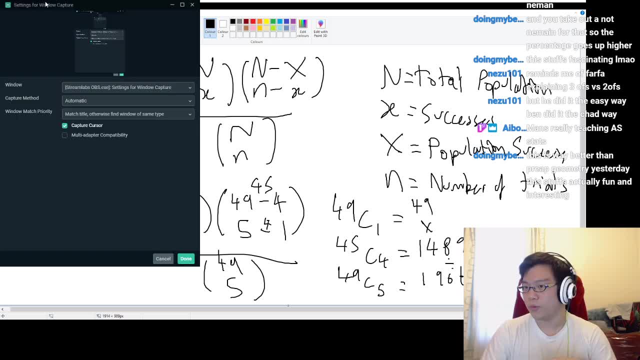 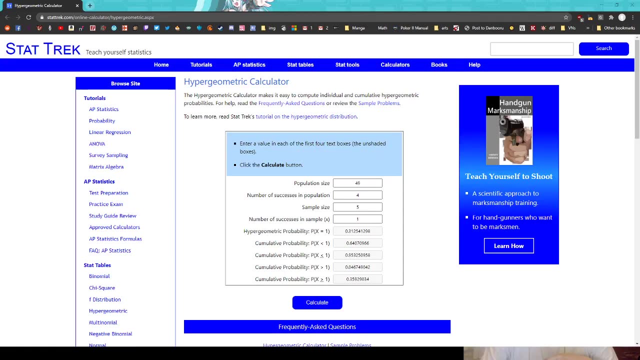 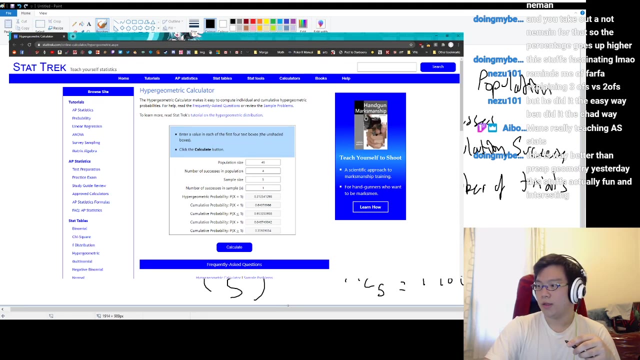 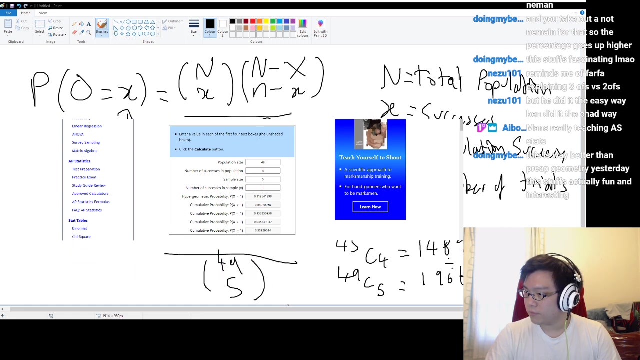 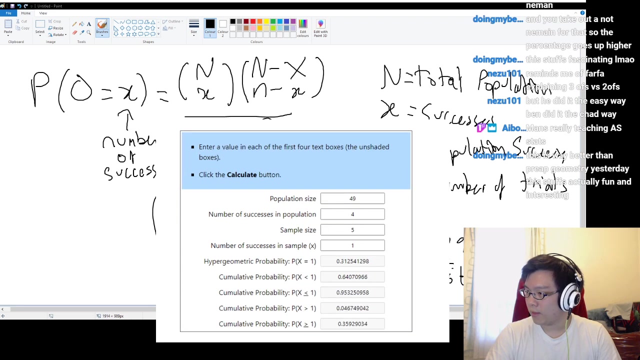 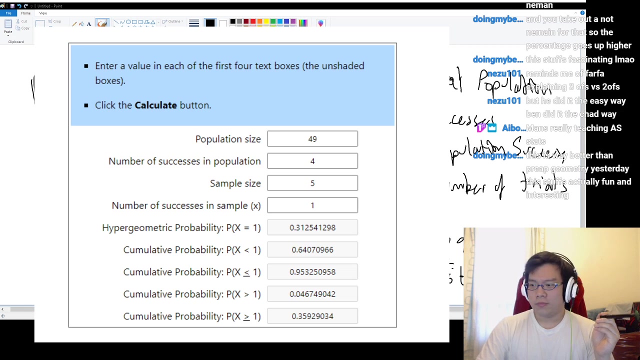 real quick, any sauce. why is always default to that here? all right, so the website: this is what it looks like and you make that a bit bigger, you come on. yeah, so this is what it looks like. the website is called stat-trekcom. let me put a link in the chat right about. 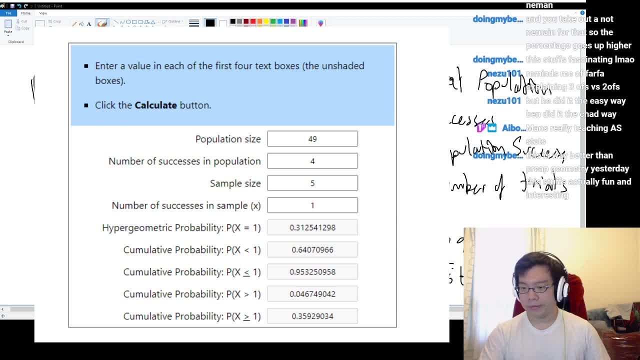 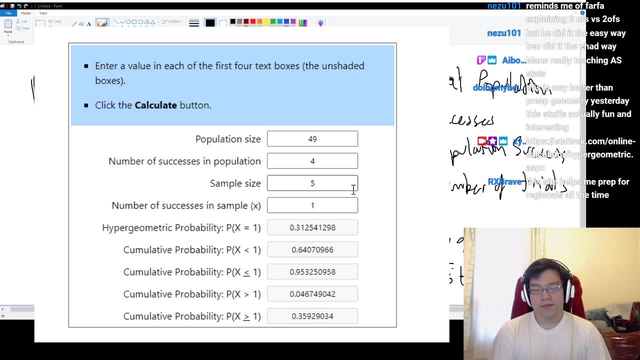 now you'll see it here. so that's the link. you see, here they've. they do it for you like it's pretty straightforward, like especially their maths is not wrong. Does that help me share the regionals time? Yeah, it's, because it's what it's. 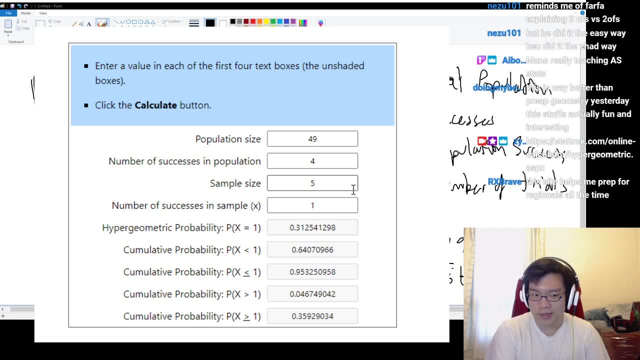 used for. So you can see. you input the population size. so 49 card deck: number of success in population 4, and the sample size of 5,. number of success in the sample 1 is equal to. that's what you did. we forgot to minus the 1, but that's yeah. 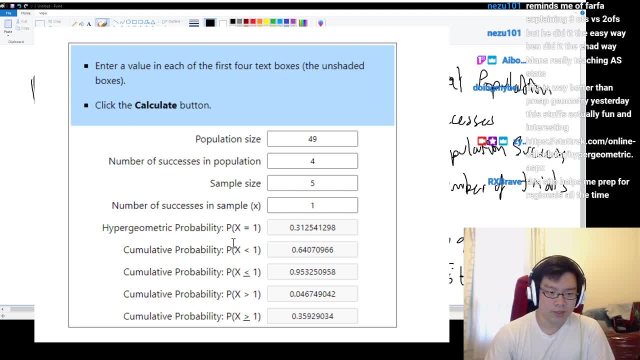 we forgot to count for the 1 anyway. You can see that the exact probability of being 1 is 3ish percent, and then you have the probability of it being less than 1 is 1 minus that. Again, basic statistics. you should all know that. 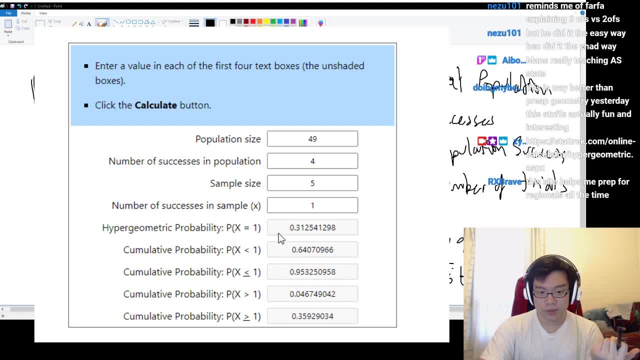 Probability that it's less than or equal to 1 is these two put together. The probability that x is more than 1 is the difference. So cumulative probability is where it gets really interesting, because that's what we're interested in, because obviously you don't care about opening just the one. 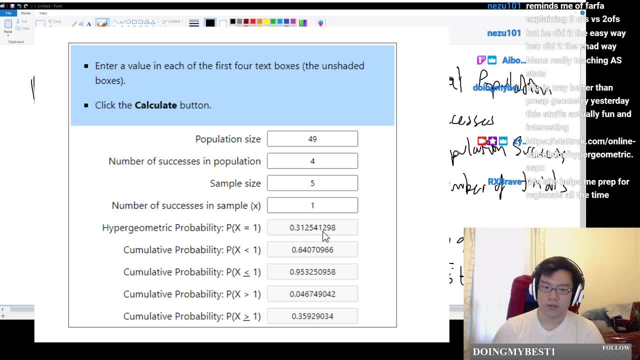 domain. you want to find the possibility of opening multiple domains, because multiples is a subset of the one success rate. So you this number will always be higher than that number, but it's usually this number that you're interested in. So let me just get rid of that and go back to something. 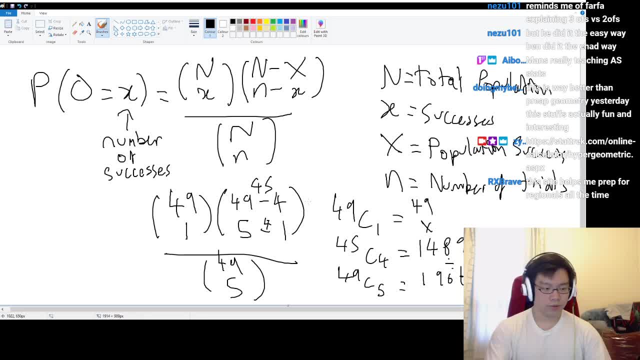 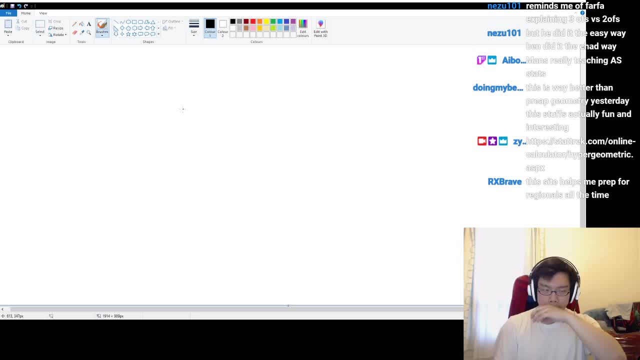 else. So you just get rid of all of this. So we know now how to calculate the chance of for a single. so you know, for a single series of tests, as in for a regular linear sequence of trials and so on and so forth, we know what the chances are of finding. 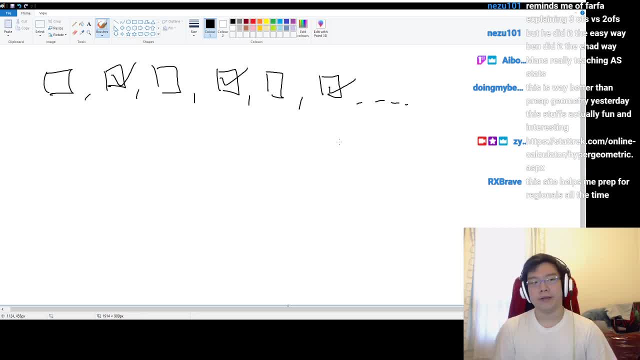 X number of successors, wherever they may be, And that's usually good enough, you know, for things like drive checking, finding a, you know, finding one-step card and opening hand. That's pretty much all you need to know. It's basically case of: it's a. it's an exemplification of thinking of «what if I open you? 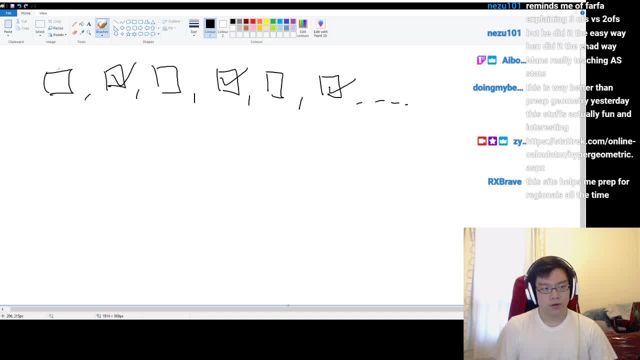 know, sum things up, even if we add another expressing one and you add the other, and so then what do you do»? Okay, see you in a while, Bye, Bye. if we look at drawing an opening hand of five cards right in vanguard now, 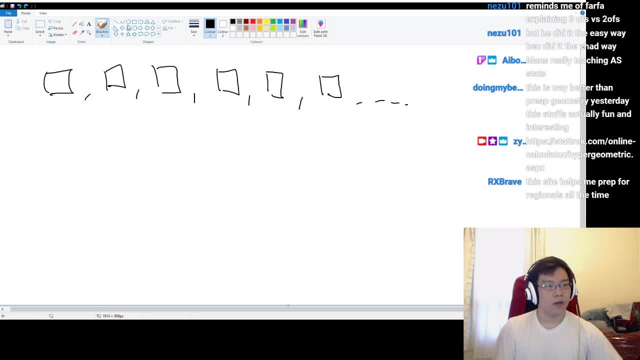 you know, card one, let me just get rid of this. so five card opening hand. it could be, this could be in the main, and then four other garbage cards, or this in the main and other garbage cards. this could be in the main, or this could be in, or that. 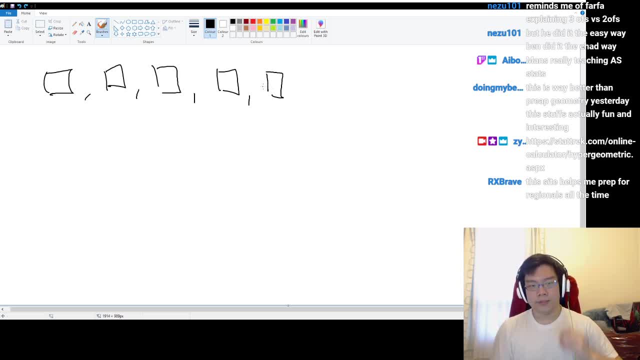 could be in the main, and each one of those is a separate probability to happen, because the chance of not opening the main here is obviously 45 out of 49. so for the main to be here we then have 4 out of 48, and then we'll go back to. 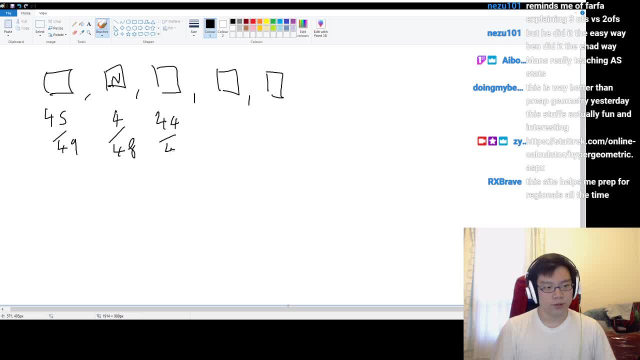 44 out of 47, because we already drew a non-success here, or rather because we've drawn in the main. it becomes the number doesn't change. and another one is 43 out of 46 and then 42 out of 45. so this is different to if the main was the fourth card, because there it would be. 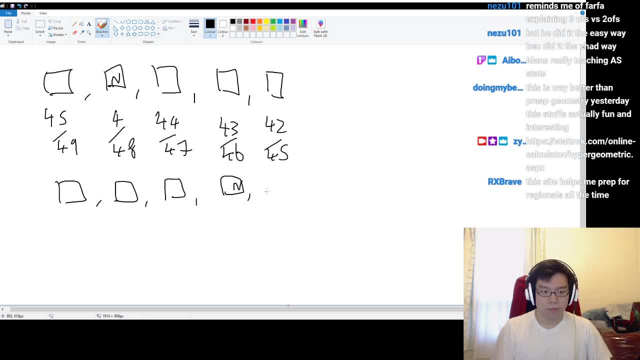 main, it would be 45, 49 and these are all multiplied because it's: and so 45 by 44 over 48, by 43 over 47, multiplied by the 4 here for the domain, over 46, multiplied by 42 over 45.. 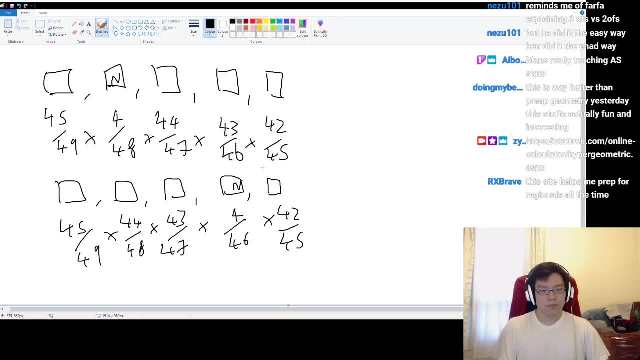 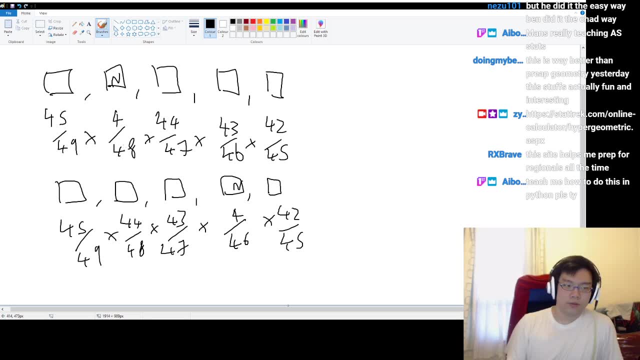 So you see that the middle, this last probability, and the first one are both the same number, but everything in between is different. So because these and these are two very different fractions, the results will actually be slightly different. And then what the hypergeometric distribution does, is it? 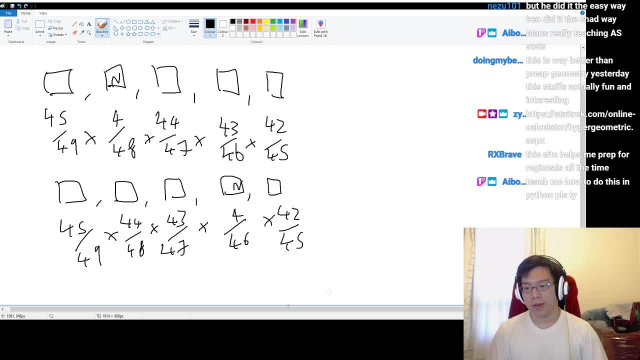 takes all of these different possibilities and just adds them all up at the end, And it just so happens that that form is represented by nx- n minus x, n minus x over nx. Teach you how to do this in Python. It's pretty straightforward, you. 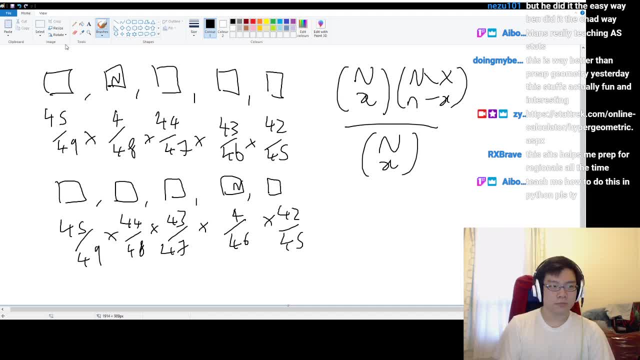 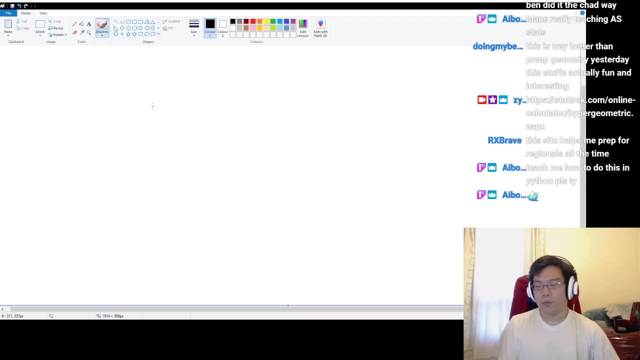 could probably figure out yourself. Python's not hard, So. So that is the basically the basic calculation. Obviously, like you'll do your one minuses or whatever accordingly, So let me just select the n. So now we you know. let me quickly go about how we do cumulative, before we talk. 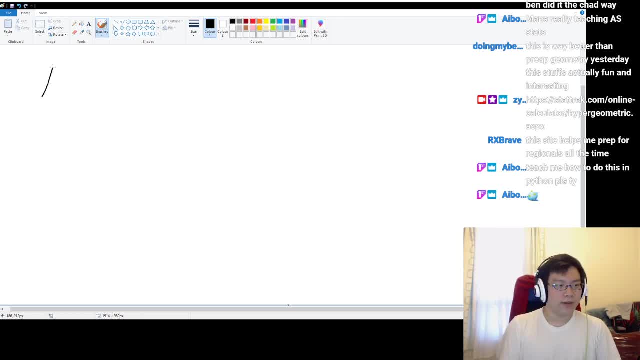 about the next subject. So let's say that you want to find at least two in the main right. You want to be greedy, you want to write one of your domains and then have another one to use superior type write chain with, and you don't always any of. 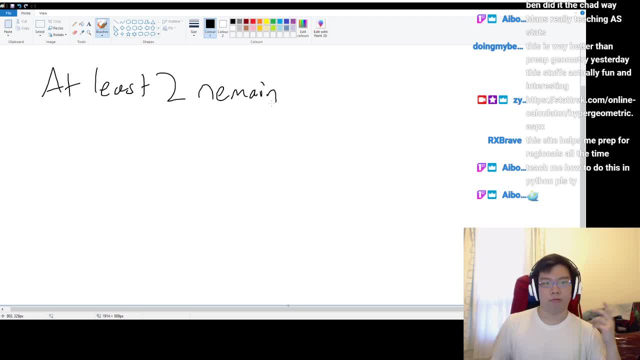 your other grade ones, even though brand one is already good. right, how you don't been riding the bank for whatever reason? because you on the 13 capability, so they're at least two- means that you don't see 0 and you don't see one, so rather you can get. 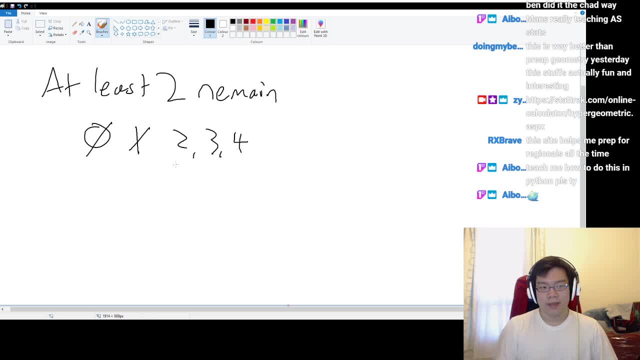 coming for this is 23 and four domain. it's easier to cap the properties of seeing exactly zero, exactly one, adding together and taking them away from the success. so 1 minus the probability of 0 and 1, right. so in that case you're plugging the formula, which is: I should. 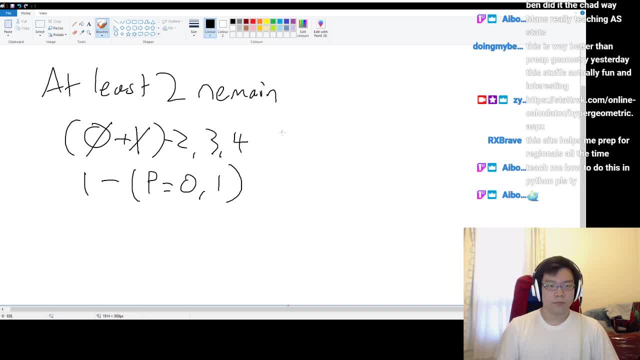 I really should memorize this, but I'm too lazy to do that- which is so. that's 1 minus P 0, which will represent like this, plus P 1, which will represent like that, which is 1 minus 49: 0 by 45: 5 divided by 49: 5. 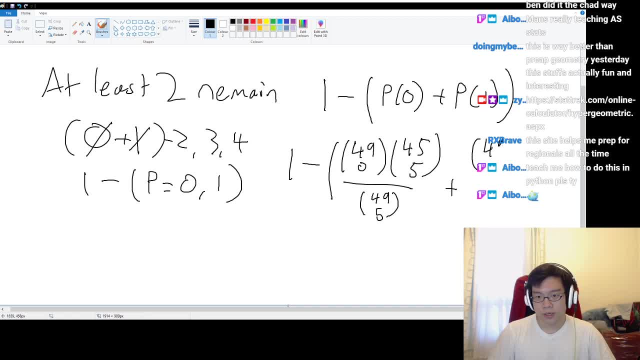 plus 49, 1, 45, 4 divided by 49, 5. now, and as you may know from very basic maths, when two fractions have the same bottom number, you can just add them up so that becomes 1 minus 49, 0, 45, 5. 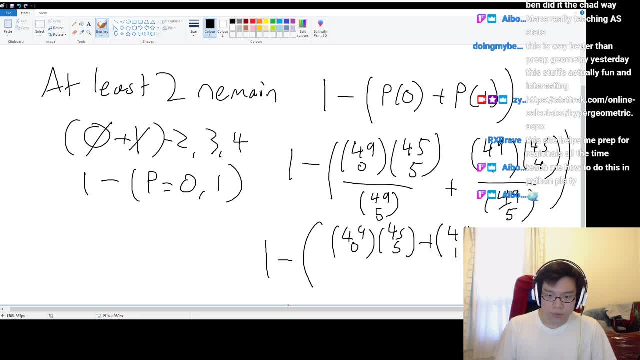 plus 49 0, 45, 4, divided by 49: 5 plus 49 1 45, 4. all divided by bad at straight lines, 49, 5. and then let me move some stuff around. I really wish I knew what Khan Academy uses. it'd be quite. 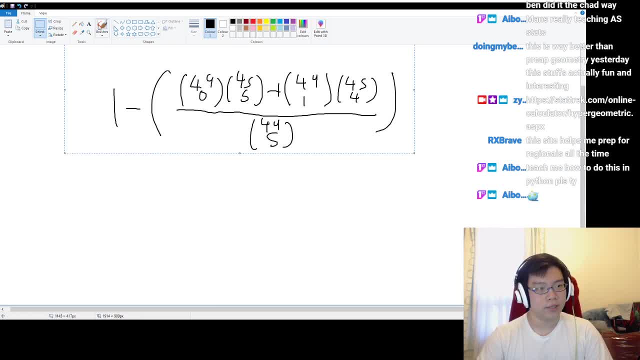 nice to get my hands on that. let's move that up there and keep going. so we know that 49 choose 0. we can calculate that. let's quickly ask Wolfram what the answer is. so 49 choose 0, that is 1. so you know that's 1 times 45 choose 5. 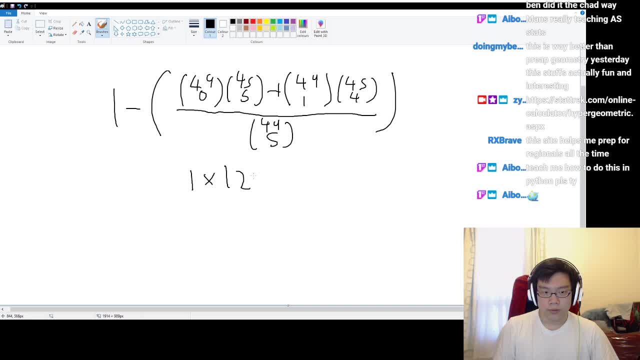 is 1, 2, 2, 1, 7, 5, 9 plus. you know that 49 choose 1 is 49. we did that earlier times. 45 choose 4. we did that earlier as well, but I don't know what the number was. 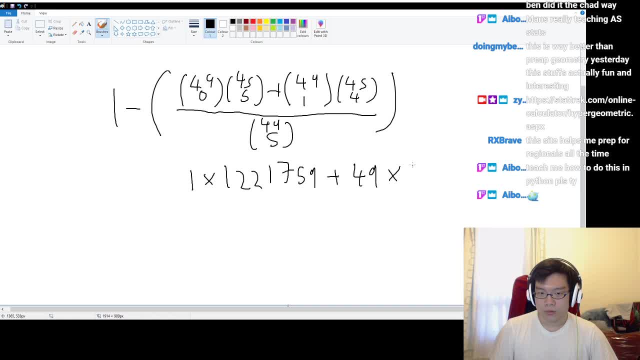 because I had six digits, that was 1, 4, 8, 9, 9, 5. we divide the entire thing by 49, choose 5, which is 4. these are my very famousρού randomina: 5, and then it Highway. 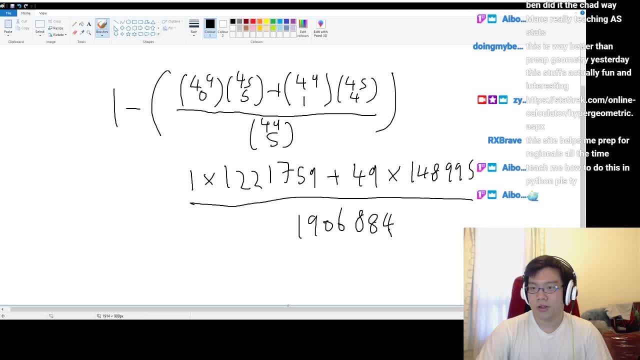 9 0, 2, 4. we can figure 4, 9, 0, 2 and 1 0, 6, 8 and 8, 4, 7, 8, 3, R, 9, 9, 0, 6, 8, 8, 4 and then just. 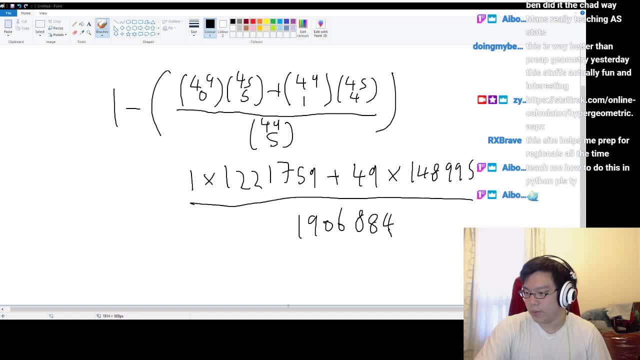 calculate that. or, instead of doing it by hand, we can go to our good friend the. I close the website, didn't I? I did close the website- are hyper geometric calculator, which let me put back up on the screen when I wasn't doing alchemy. I'm just going to. 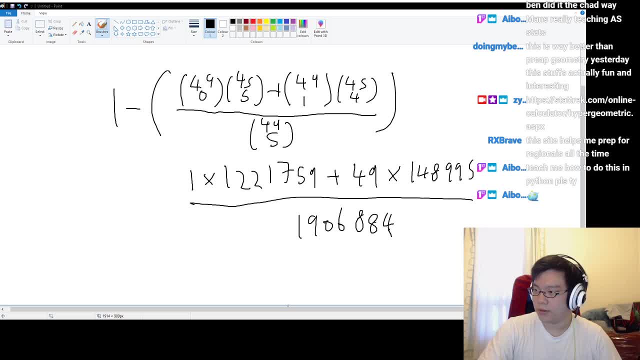 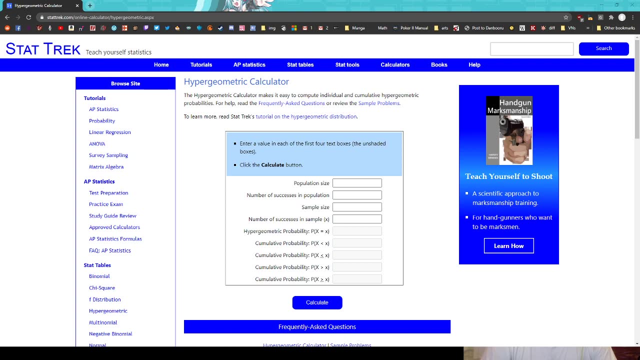 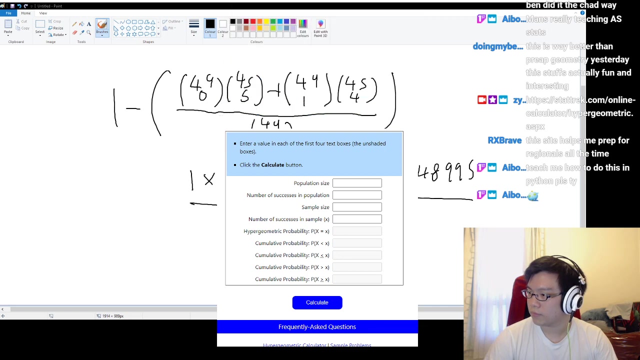 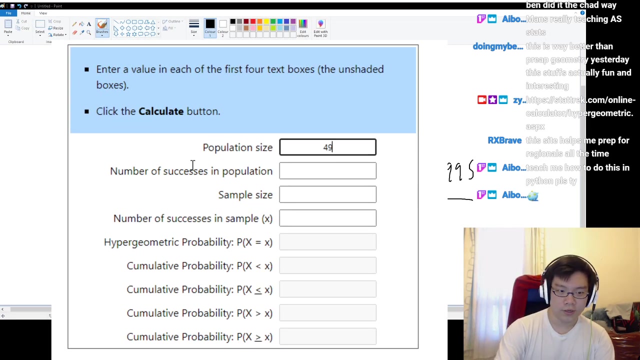 I wish OBS would just play nice. So add that and I want you to point to this page and I'm going to need to resize this again. So population size of 49, number of successors: 4, sample size: 5, successors. 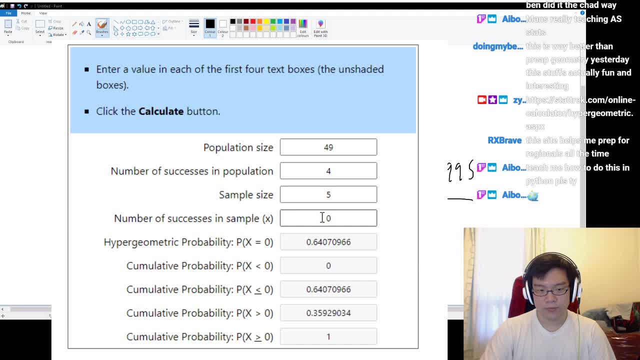 So first we want to find the probability of x equals 0,, which is 64%, then the probability of x equals 1,, which is 31%, So 64 plus 31.. Okay, 60, which is 0.64 plus 0.31, is equal to 0.95. 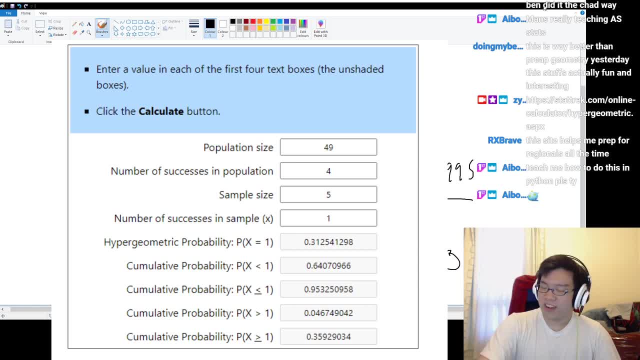 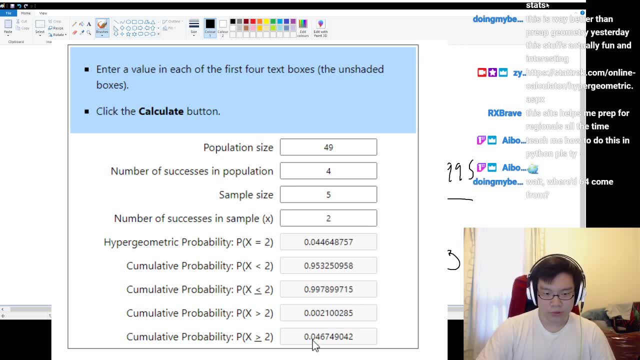 So 1 minus 0.95 should be 0.05.. So you have a 5% chance to open two domains in the top five cards of your deck. If it's just a 2, the probability that x is greater than or equal to 2 is about 0.5.. 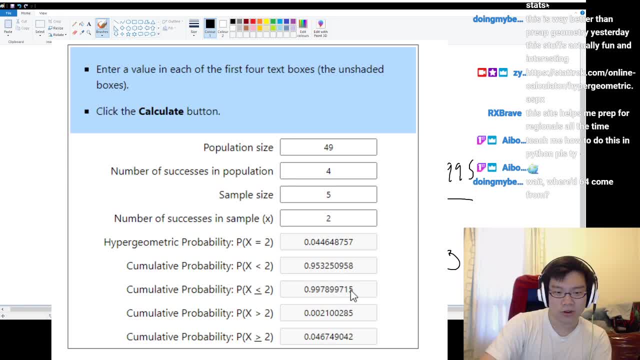 Now, the reason this is a little bit lower is because there's a lot of rounding errors that we need to account for. all right, If I, if you go back to- oh, nice, Okay, If I go back to here and type 49,, 4,, 5, 1, you'll see that probably x equals 1 is actually. 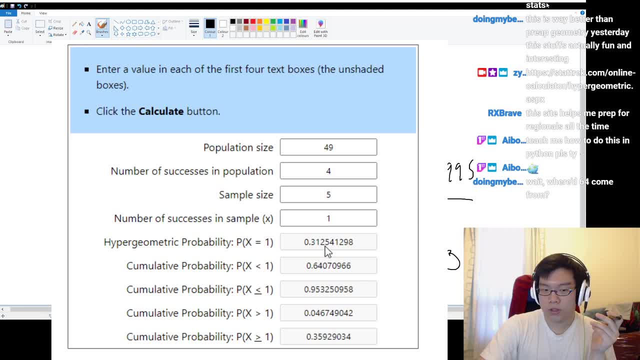 close to like 0.32, because it's like 0.03125, which this rounds up and the probability that x equals 0, 0.641 and that these all add up a little bit more where 64 come from. 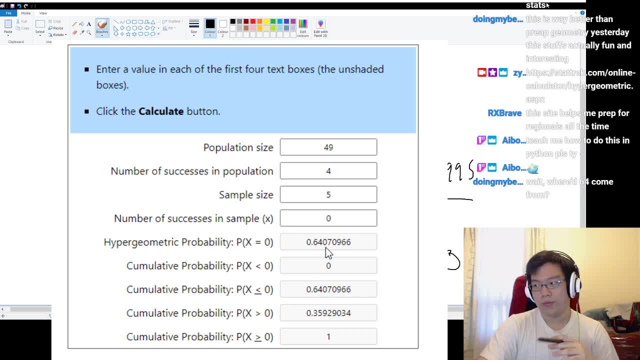 So a probability is always between 0 and 1.. That's the basic statistics, So the prob. Okay. So if you want to say 0 and 1, you need to multiply this number by 100 to get the percentage, Because 50-50 is half right. 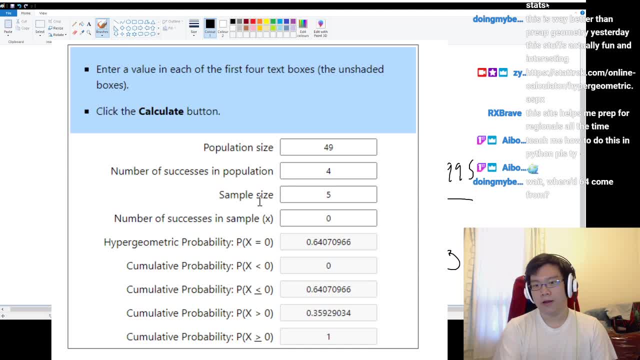 So if you half a chance to flip heads versus half a chance to flip tails, half is 0.5 numerically, but it's also 50% statistically out of 100%. So this number- any decimal you get in probability- usually needs to be multiplied by 100 to convert. 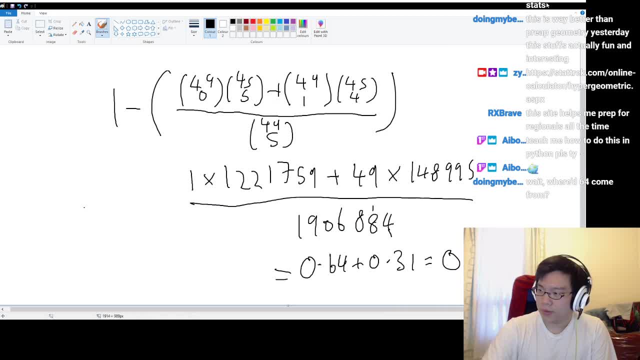 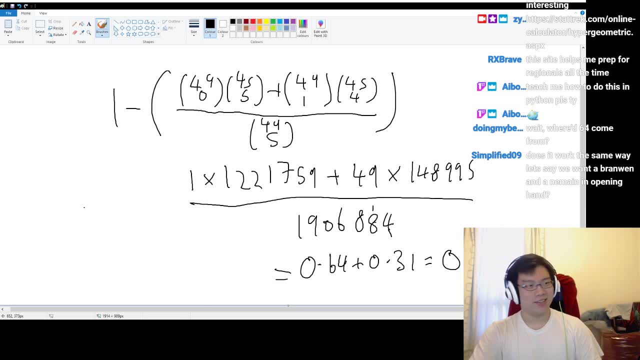 to percentage form. So that's that, Okay, Okay, Okay, Okay, Okay. Does it work the same way? Let's see, We want a brown one and a main and an opening hand. Aha, This is the topic I was about to get to next. 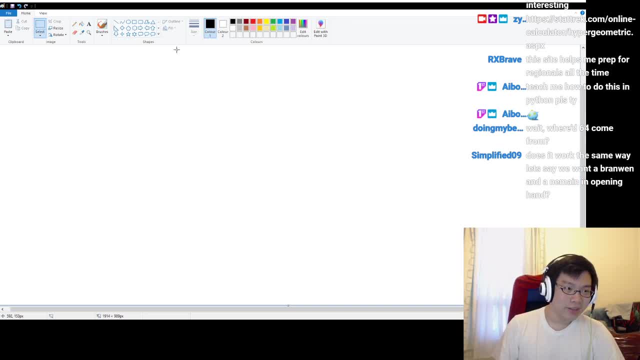 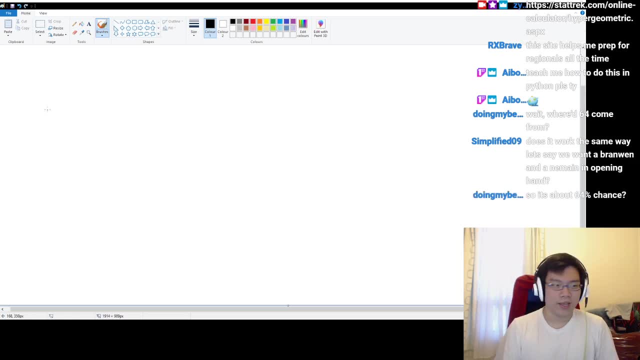 I'm glad you asked that, because it does not work the same way, because Let's go back to the bag of Marbles example here. So that, Yeah, It's about, excuse me, No 64% chance to open no domains in your top five. 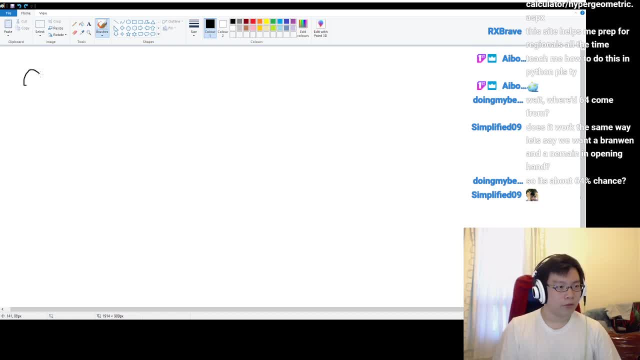 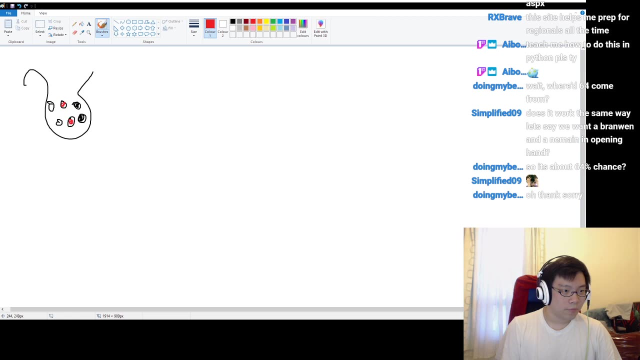 Hello, What happened? Right, So you've got our bag of Marbles. Okay, Cool, Cool This time. two of them are black, two of them are white, and now I have to change color. Two of them are red. 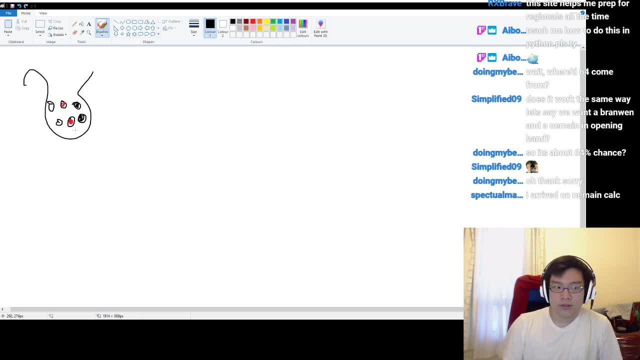 The reason we can't do it straightforward like this is because the chance of pulling There are now three outcomes. So if you think about it, before, right, With just two colors, we had like a tree right. So the first chance you had chance of failure, chance of success, and then after each individual. 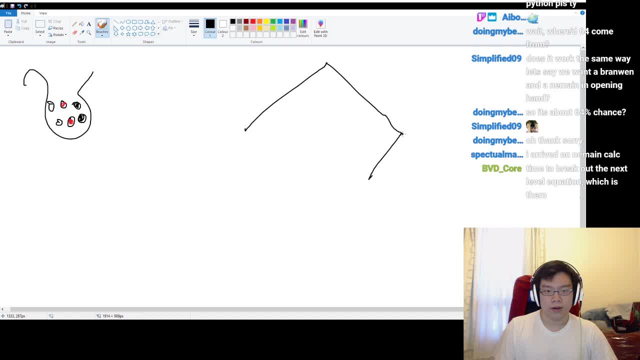 failure, success would have been another failure, and another success Here would have been another failure and another success. So, because we have two decisions at each time, there's less calculations to do, So let's say that it's, Let's go back to having half black, half white. 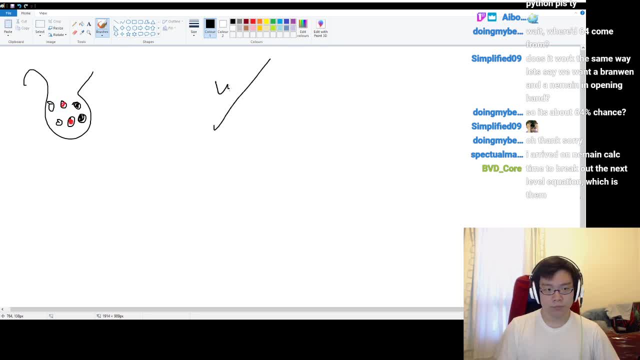 There are only two branches. when you pull out any given ball, You either pull out a white ball- Sorry, got hiccups- Or a black ball. But now that we introduce red, there's now a third option, which is red. 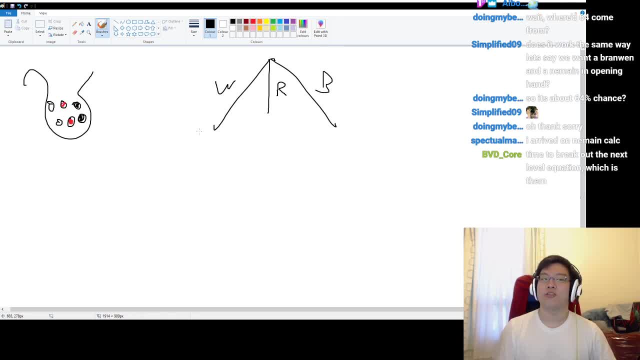 And then each time, each of these three branches then has three branches off of them, being white, red black, white red black, white red black. So you can see how the complexity scales. Okay, It scales massively. 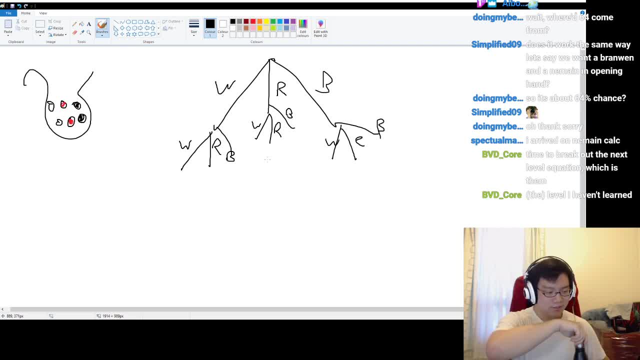 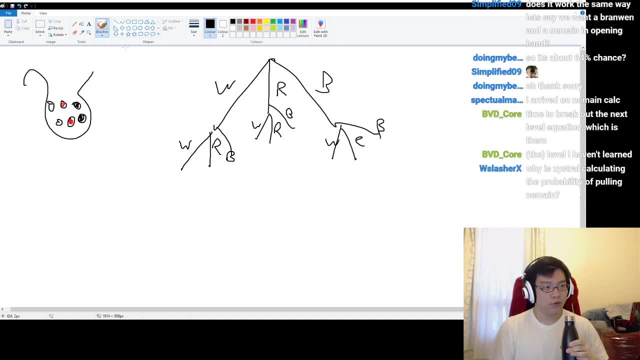 But fortunately, thanks to the hypergeometric calculation, there is a way around it. Now I never formally learnt the distribution for it myself or the derivation for it myself, So I can't tell you why this is what it is. I can just tell you that this is how it is. 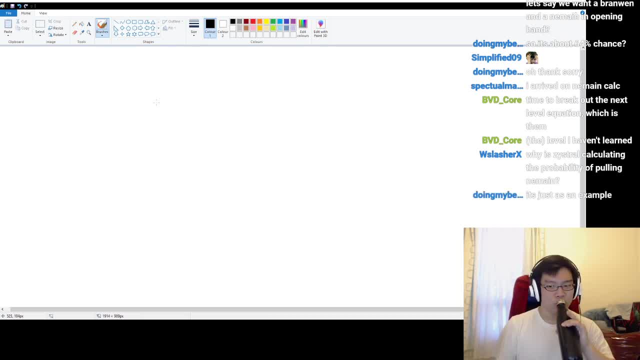 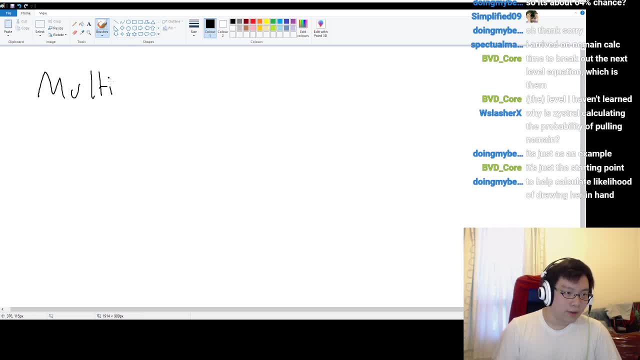 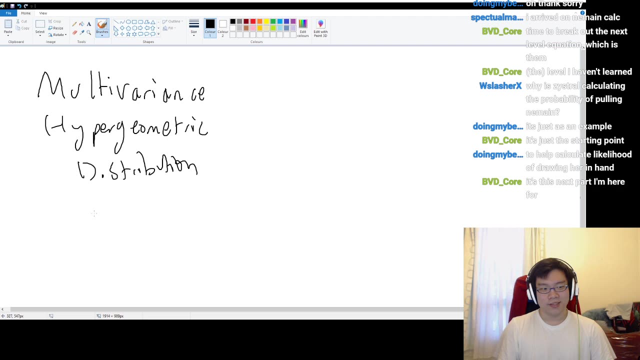 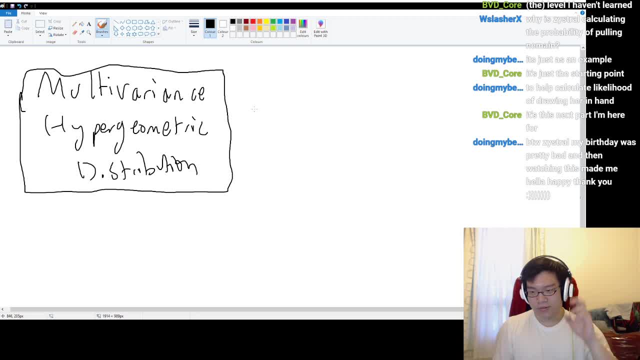 taught this. I had to learn this on my own, so I'm just going to show you what it kind of is. Thank you for the kind words. hopefully you'll learn something. So the probability of having x1, sorry, so little. x is the number of successes and big. 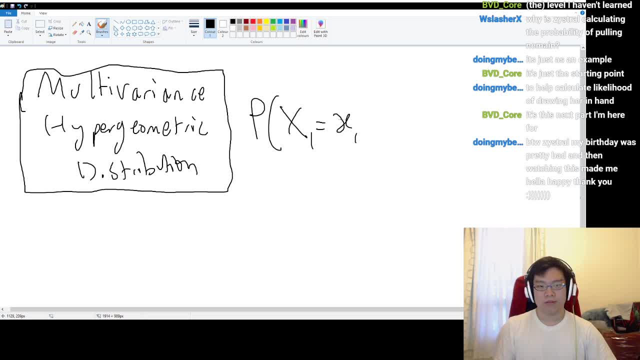 x is the actual target of having this number of these successes, and then x2, x2 and so on and so forth is equal to. let me pull up my notes again. I had this written down and I can't remember it because I didn't study properly. 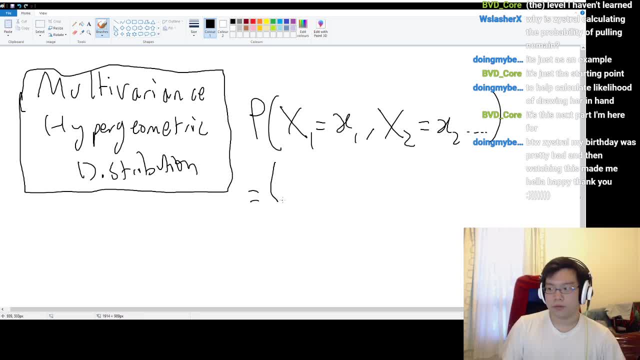 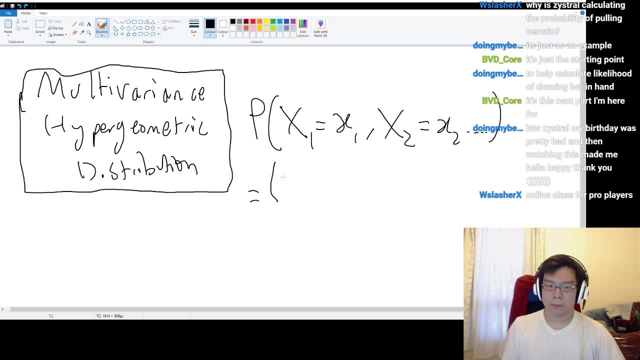 This can't be true. This can be described as: that's not meant to be, x that's meant to be. it's going to be really hard to explain. oh yeah, that is correct. so x1 multiplied by x2 multiplied. 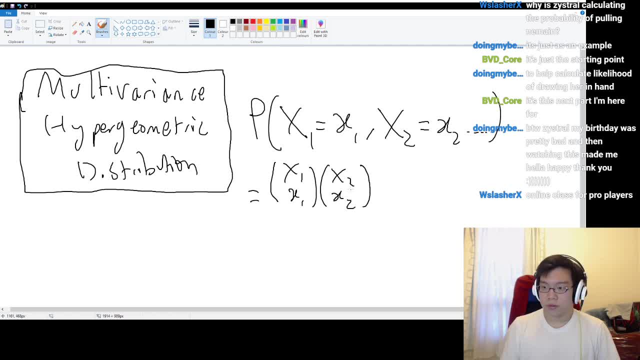 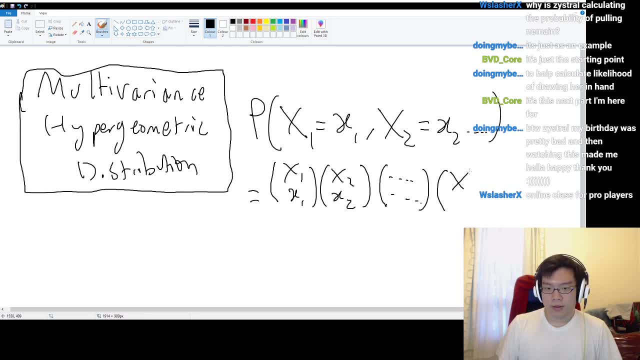 and then finally multiplied by X, big X minus X, 1 X 2, so on and so forth. and this is that's not meant to be X. is it that's meant to be? that meant to be an X? no, what number is that meant to be? it's meant to be N minus X, 1 X 2, and so on. and 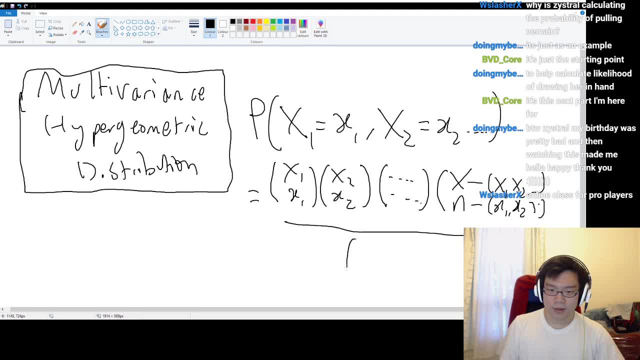 so forth. that then gets all divided by big N over little n. this is all. it looks a lot more complex than it seems. so sorry, yeah, it looks more complex than it is. it seems more complex than it is. it's actually a lot easier than you think, so. 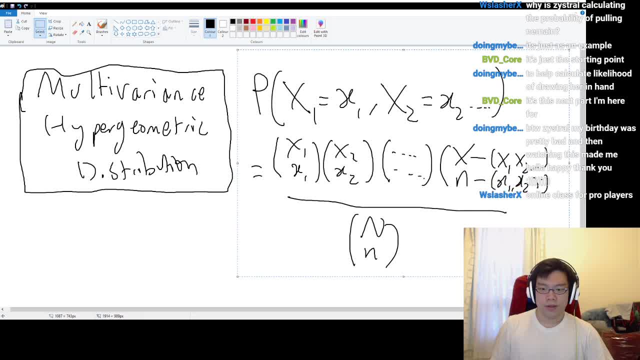 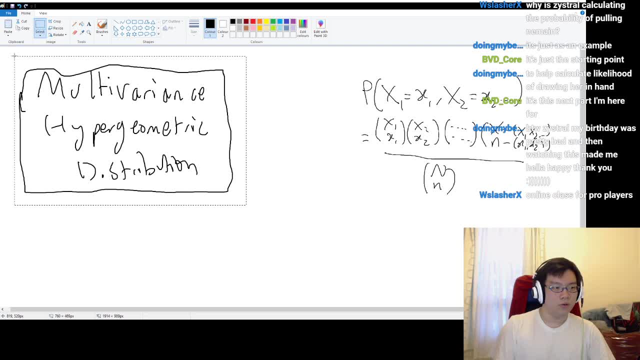 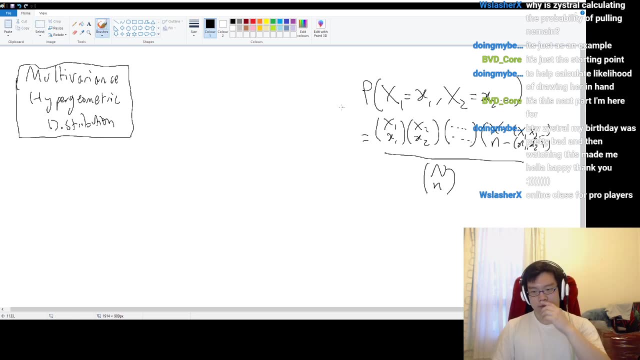 let me move this up here for a bit and make it smaller, just to get out of the way and make this a little bit smaller as well. get out of the way and we'll plug some numbers into it, just things that works. so in this example, let's say: 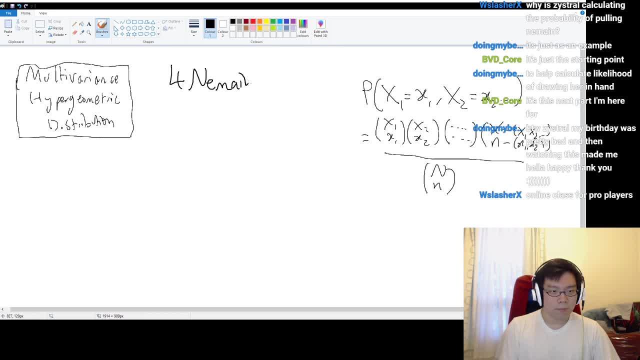 that you play four domains and I don't know what's a good number. 13 other grade ones, right. so for 17 greater ones total, that's not a ridiculous number of Shadow Paladin and 17 total great ones. so you want to open at least one of. 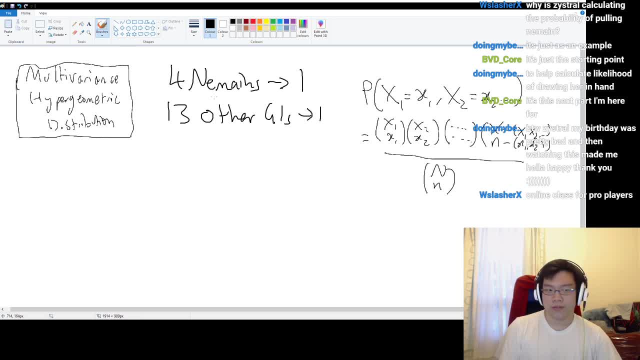 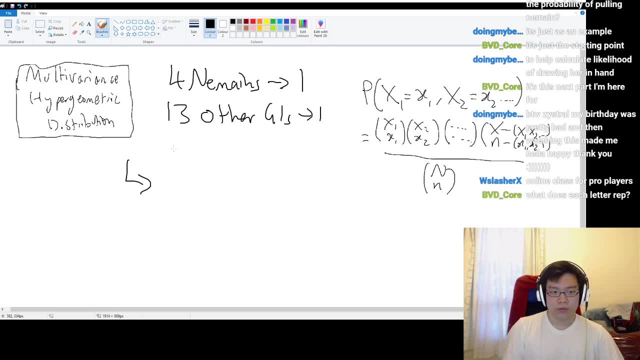 these and at least one of these, so that you don't have to ride the domain that you pull. it's fine. so here this would be calculated with- or no, let's call it exactly one. just make it really easy. so what does each 0, so the big X, refers to the number of successes for that item in. 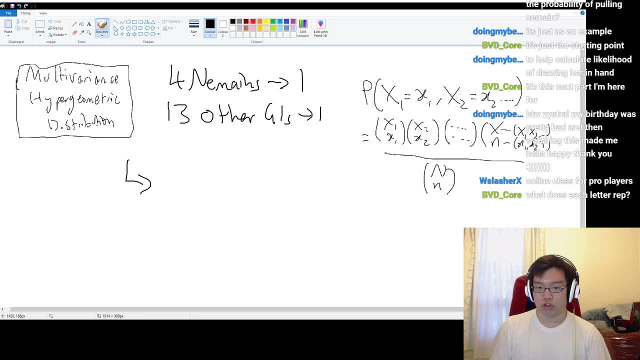 the little x refers to the number of that item you want to see in your trials. big N is the total population and little n is the number of trials that you run. so here it would be. you've got four domains. I want to see one of them and 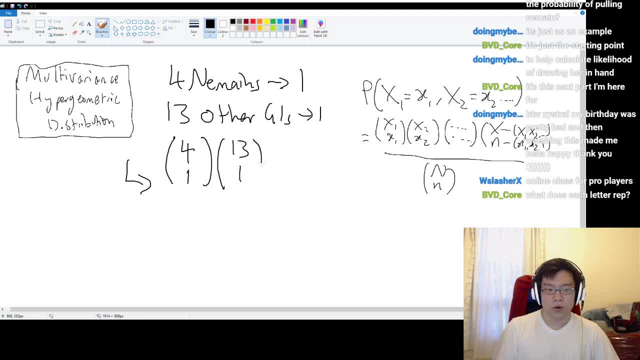 then we've got 13 other grade ones- I want to see one of them- and then we have 49 minus 13 minus four. so that's forty nine minus seventeen. is 37, 37, it's not 37, is it? it's not? am I being dumb? it's thirty-two. yeah, yeah, whoops. 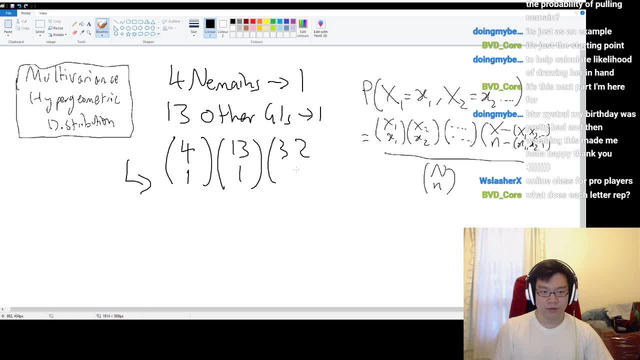 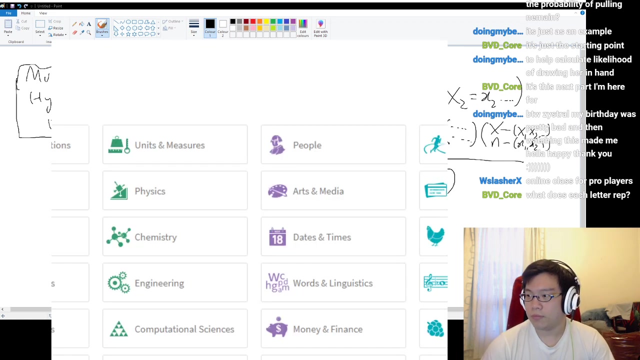 and then the remaining number of cards we can draw on opening hand of five is three, and then that gets divided by 49 over over five, and that is was my cursive on that is: let's go to Wolfram alpha. let me bring this back onto the screen from alpha. don't need to rescale this on. I. 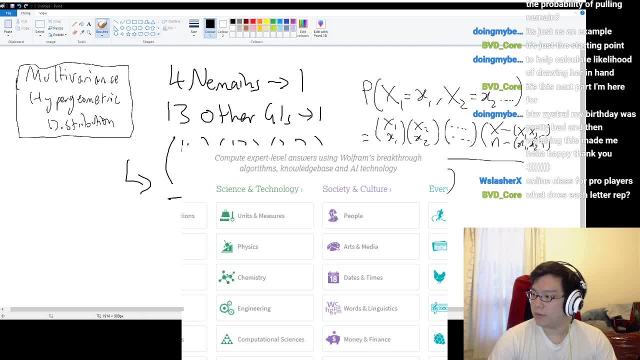 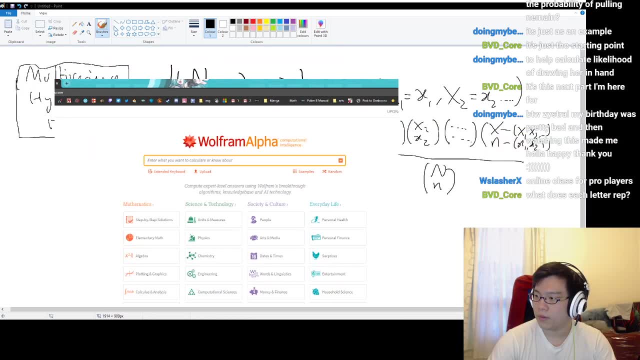 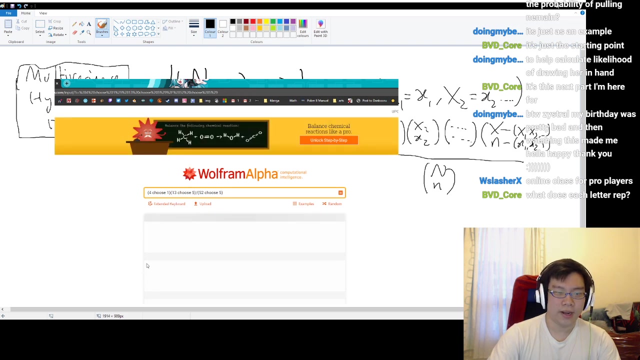 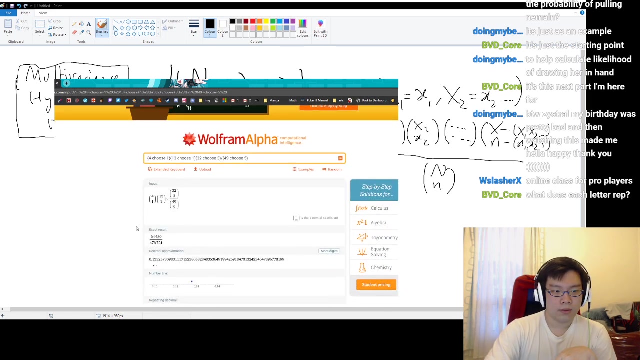 yep, small, scale that way, scale that way, scale that way. all right, so what's our calculation? our calculation was: four choose one, four choose one, multiply. I decided this earlier. it's kind of four choose one, thirteen choose one, and then 32 choose three, divided by 49, choose five, and that is this decimal. 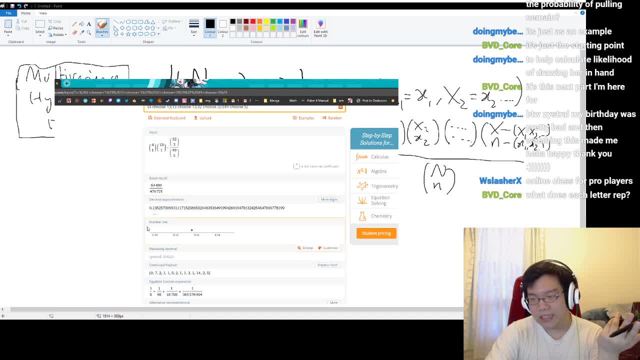 which is equal to multiply by 100, is around 13 and a half percent to open a grade one and in the main in your opening five cards. now this doesn't account for things like mulligan. obviously we're in the top five cards here, but you don't have to worry about it. 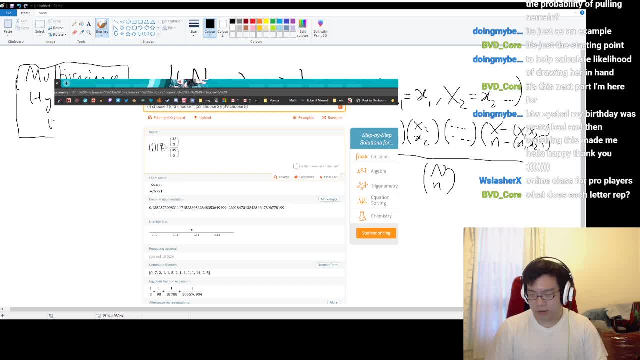 because you don't have to worry about it. you don't have to worry about it because you don't have to worry about it. you don't have to worry about it. you can see how the calculator is created. right, you have four domains. you can see one, 13 other grade ones want to see one, and then the other three. 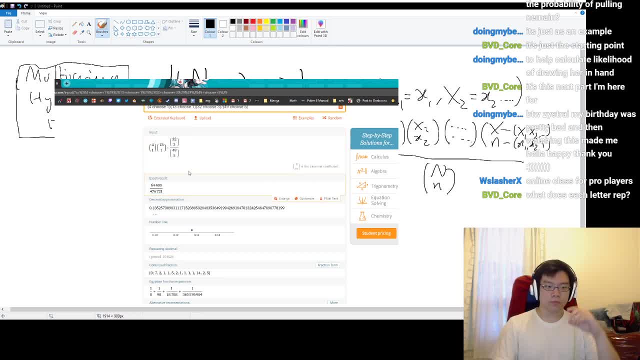 cards you want to be, does of the rest great and that's pretty much it. so you know the chance of that's it, the chance of opening grade one and the main is 13%. but of course, like I said before, we want cumulative because you want to have at. 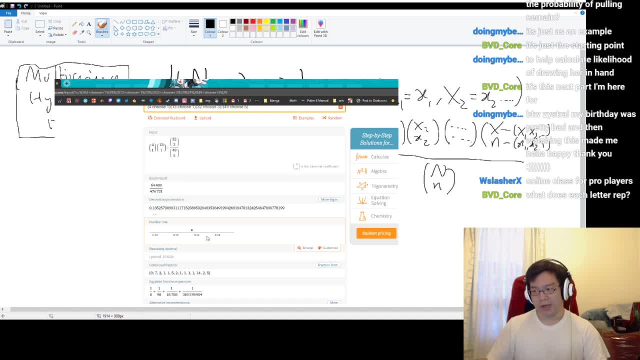 least like ideally. you wanna have your grade one in the main Luad and then two other cards. that's a whole nother thing. but what if you only care about opening the main in grade one? so yeah, see, at least right. so you want one, minus the chance of opening none. so what you actually want is: 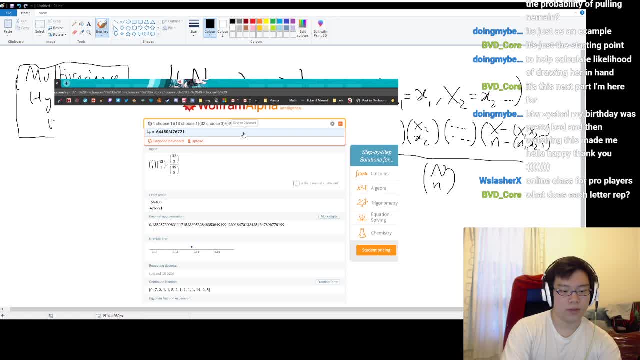 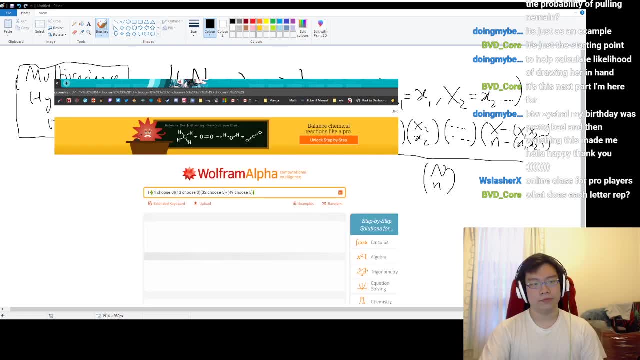 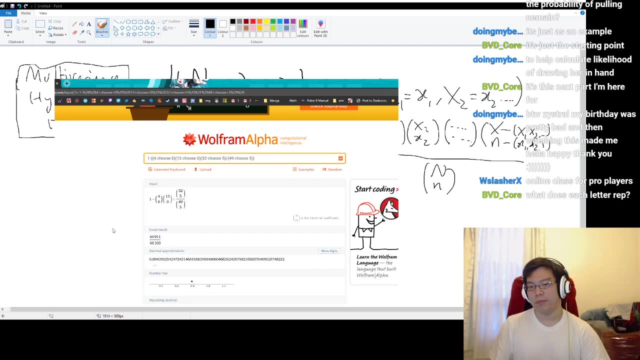 one minus all of this and instead of seeing fortune one, it's four to zero, thirteen to zero, and this choose five, so it's actually an 80 or well, this is actually a slight of approximation. it's actually a bit lower than this, but you are just, you're- over 80 percent favored to find a grade one and, in the main, in 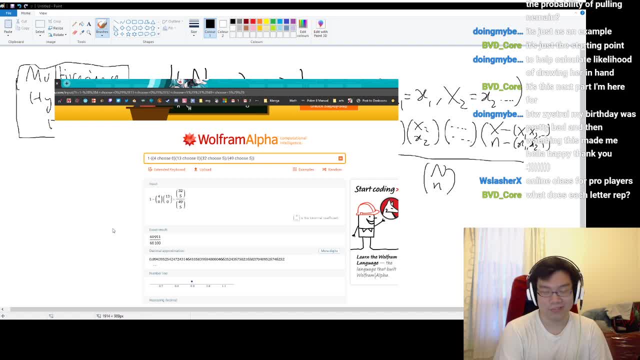 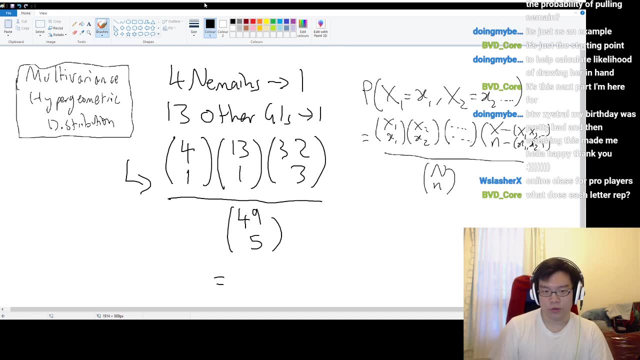 your opening five cards. the chance is really high. it's really hard to break with Luad who would have guessed. but yeah, that's not. that's the application of the numbers. so, to recap, open it again. so multivariate distribution. you take the number of you, of the total number of your first success in the population. 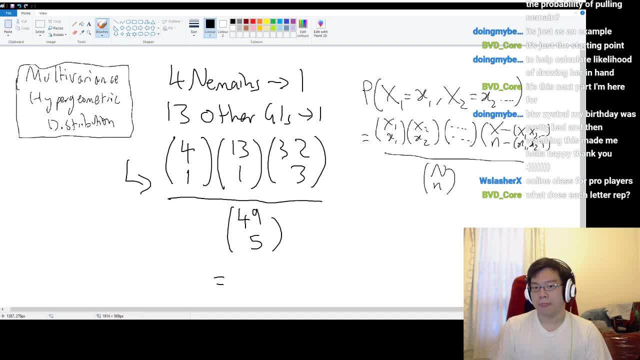 choose it by the number of successes of that you want to see, and then the number of assessors of the second population numbers is of those you want to see, and until you reach the success of the chaff, the other cards, as it were. Do you have a calculator for this or do you need to use Wolfram? 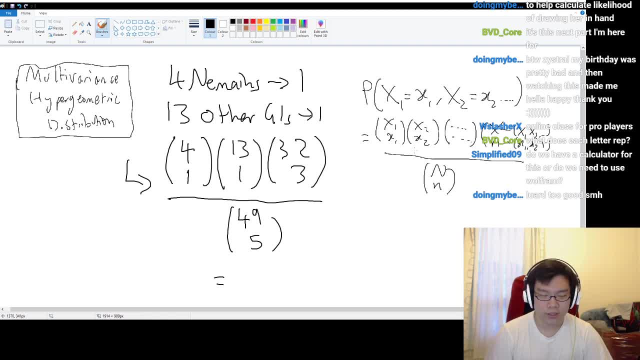 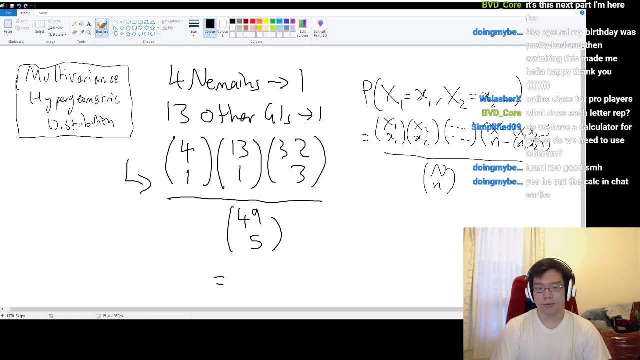 You have to use Wolfram. unfortunately, The stat track link I above only does individual- What's the word? Only does single variable calculations. But, as you've seen, it's not too hard, Depending on how many things you're dealing with. 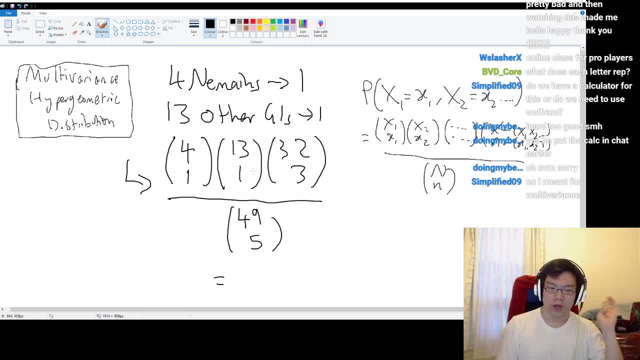 if you want to see 1,, 2,, 3, and 4 cards in the top 8 or whatever, it becomes a lot more complex to do. But once you understand how choosers work, you can just punch it in really easily and calculate it yourself. 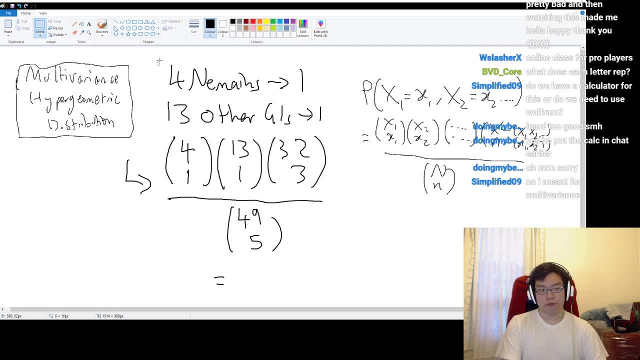 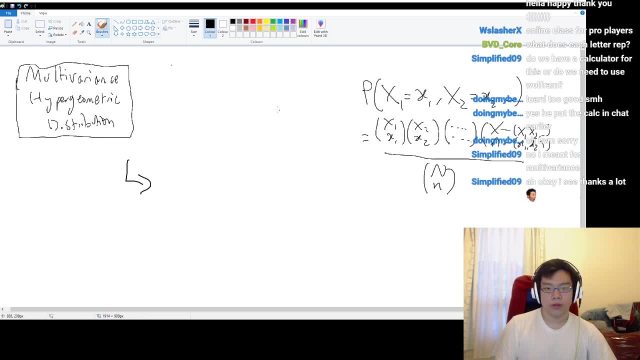 It also helps with things like If you want to find 3 of something or you want to have 3 variables, it's only 1 extra calculation. So that's 4 of a grade 1, 4 of a grade 2,. 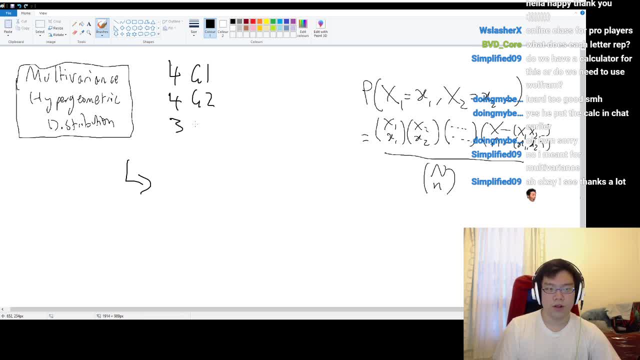 and 4 of Let's make it funnier, Let's make it spicy. You have 3 copies of some grade 3, and you want to see 1 each of these in your opening hand. You would just do 4, choose 1.. 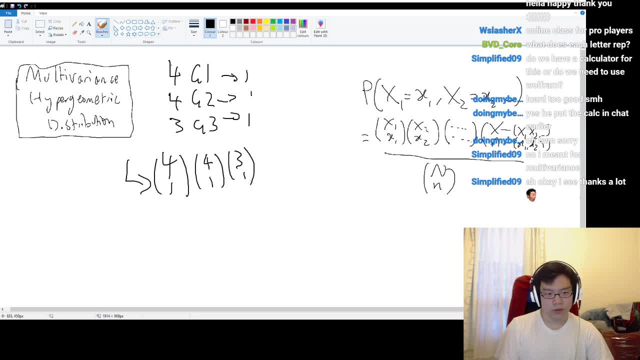 4 choose 1.. 3 choose 1.. And then The other cards is what? So that's 8,, 11,, 38- choose 2.. All divided by 49: choose 5.. So now that's the formula and how to use it. 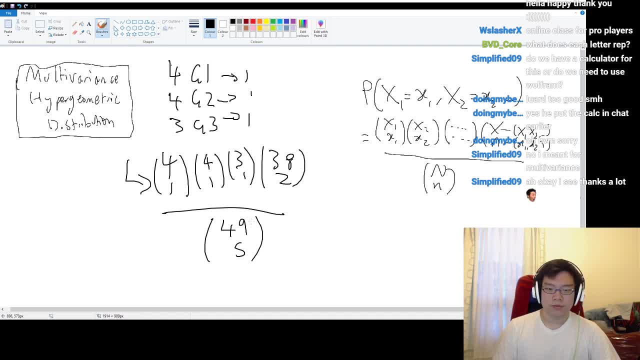 I want to break down a little bit to show you how interesting this really is. You have So this down here. this combination is 49 choose 5, which is how many different 5 card hands can you draw in a 49 card deck, right? 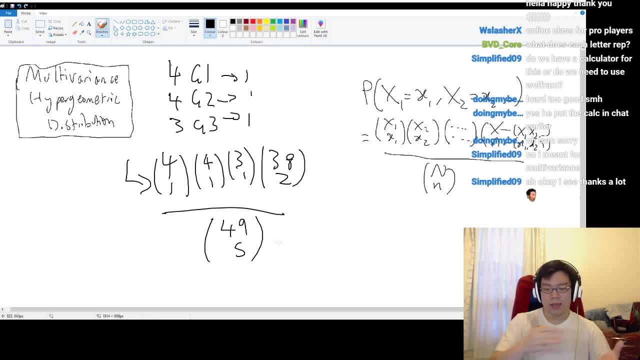 And that kind of makes sense, because That's like saying: here's all the deck states we can have, and now I want to see the ones with the top 5 cards. the order doesn't matter combination, but the actual cards in them does. 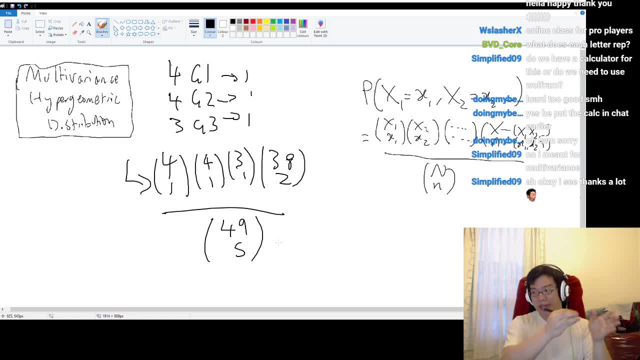 That's So out of all the various possible, infinite, almost infinite number of deck states, you can shuffle a deck. into which unique 5 cards can you make out of those? But you still need to count for the original 49 cards there. 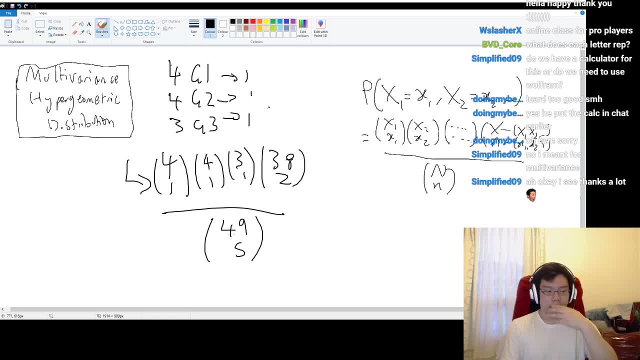 because That's how likely you are to have been into that deck state in the first place. right Like, Let's use some really simple numbers. Let's pretend there were only 1 million possible deck states, which is a lot. 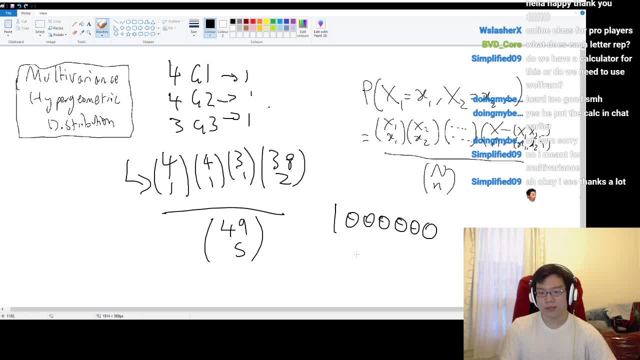 but it's an easy number to think about. So we have 1 million possible deck states and you want to see. So the chance of you being in any given deck state is obviously 1 in 1 million and you want to filter them down to find deck states that match a specific chance. 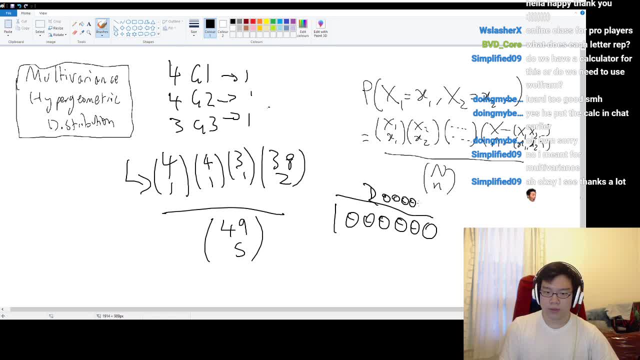 So let's say that 200,000 of those match that 1 million deck state. So now you're looking at just those 200,000, which is where this calculation comes from- and you're playing around that, but all of that still comes down to within this original out of 100 million. to begin with. 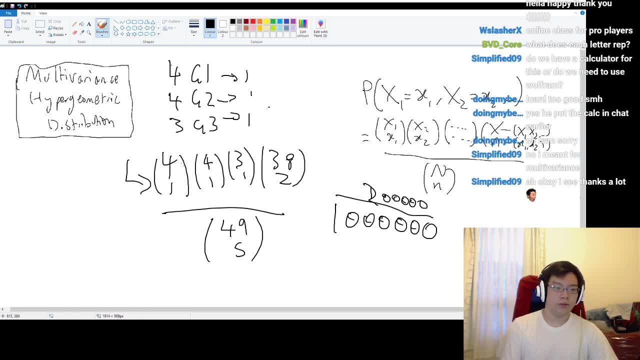 sorry, out of 1 million to begin with. And so these calculations are just saying you know which What? Where can this grade 1 exist? Where can the grade 2 exist? Can it be in the first card, second card, third card, so on and so forth. 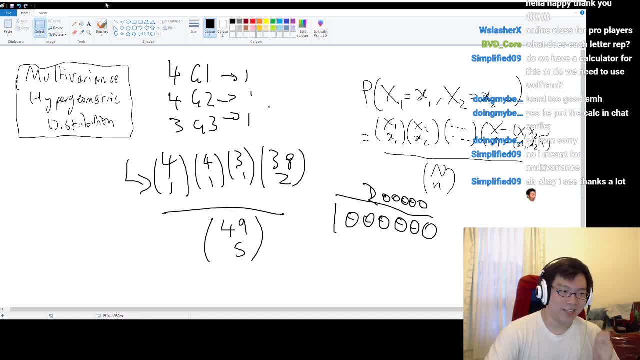 So That is is multivariate hypergeometric distribution, and this is probably the most useful thing when it comes to, Even for things like Weiss. what's the probability of having my grade level 1 character, my level 1 climax, combo climax, and so on and so forth. 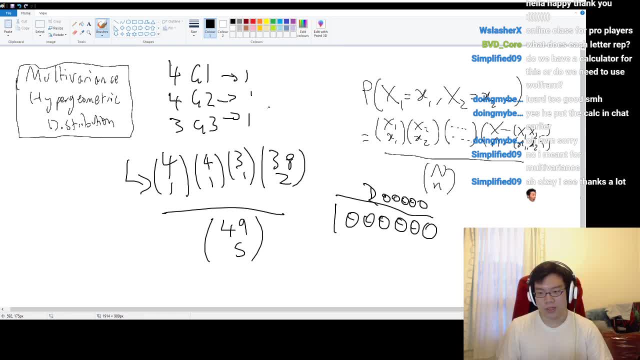 In Buddyfight, what's the chance of opening this and this, whatever combinations you need, Even in Magic, like what's the chance of opening X number of lands and X number of non-lands? It's really really easy to apply in many different ways. 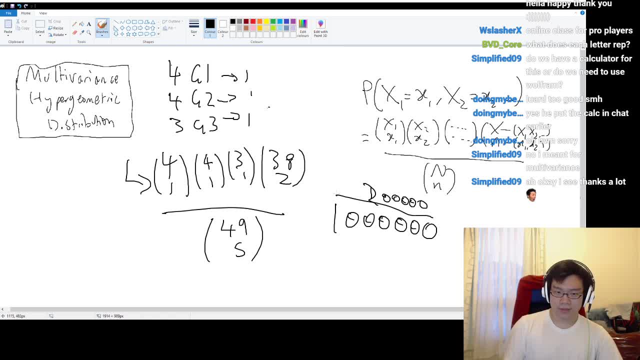 So Sorry about that. That is the basics of it. Let me just have a look at my notes. I think I've covered everything, Yeah, So The important thing to note here is that the reason this calculation becomes so much more complicated- 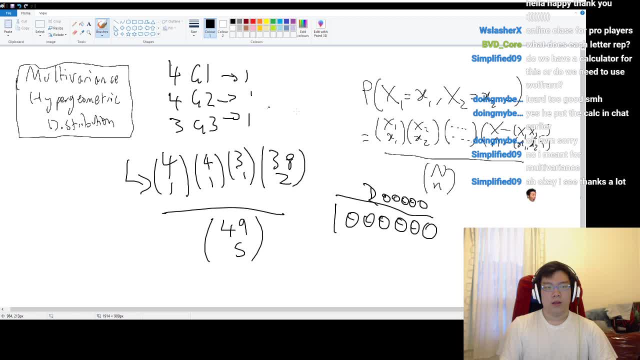 for things like card games is because we're performing- Oh, What's the word? It's conditional Because we're performing trials without replacing the population. It's not strictly conditional in that the result of the previous one affects the result of the next one. 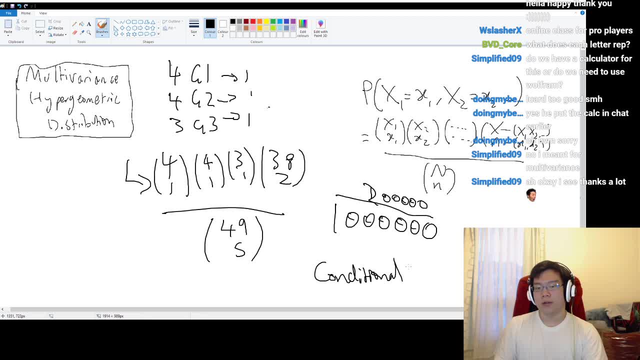 Rather, by looking at the first card, we know that we are in one of. So, Again, let's say that there were only 1 million deck states you could have been in and only 200,000 of which have a trigger on the top card. 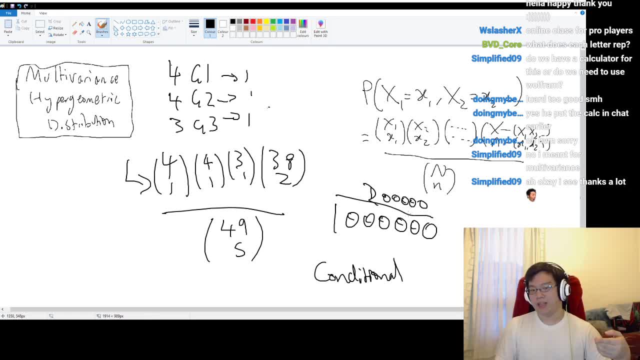 You know that the moment you flip over that top card and it's a trigger, instead of having a million deck states that your deck could be in, you know for a fact that your deck was now in one of 200,000 of those million deck states. 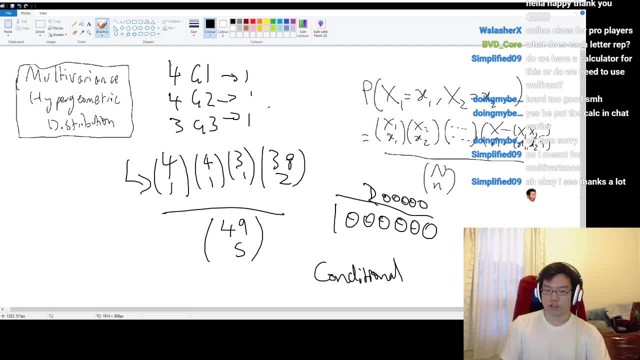 So with the knowledge that you drove check a trigger on the first trigger, the probability of you getting a trigger on the next drive check becomes this number based on this knowledge. But the probability of you getting that second trigger at all still came out of this 1 million. 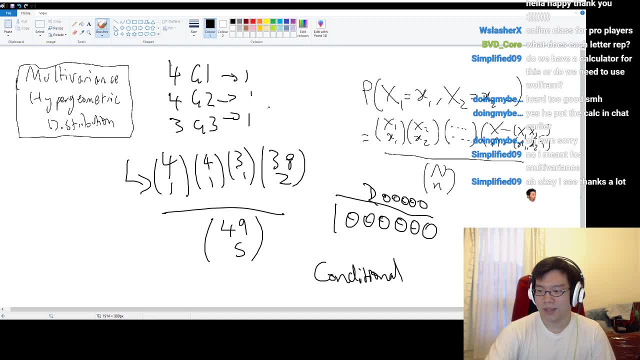 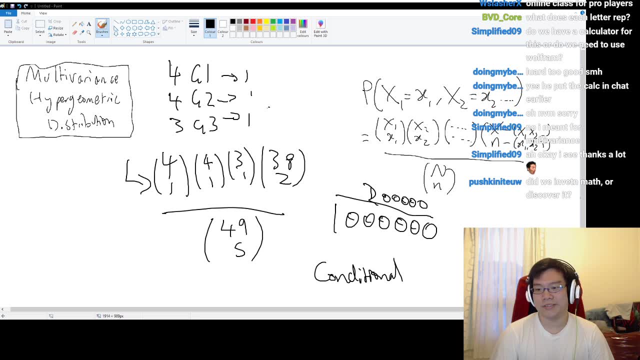 Alright, Now, that's the main thing I want to drive home here, In that it's all conditional. Did we invent math or discover it? I like to believe we discovered it, Although, I mean, this is a wholly separate discussion from another time. 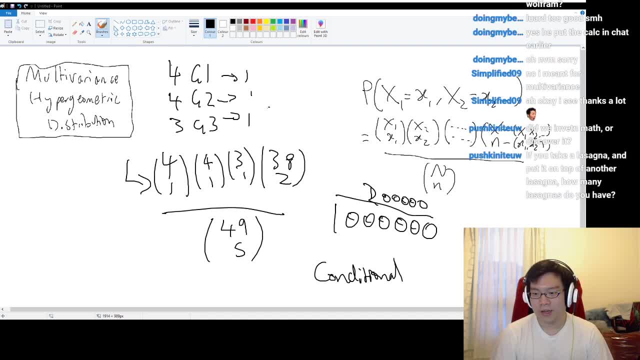 but obviously our entire way of numbers and thinking comes off of the decimal system, because we have 10 fingers on our hands so we can only count 10.. If you take a look at the top of this lasagna, you have x squared lasagnas. 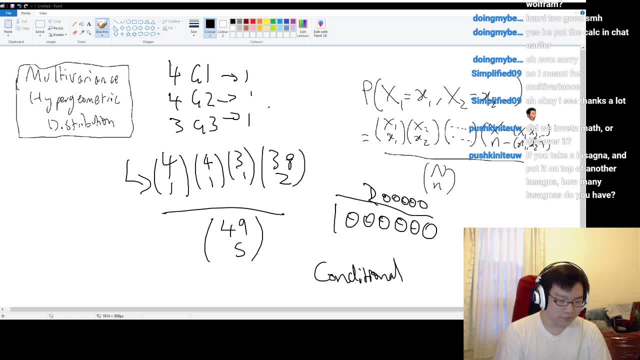 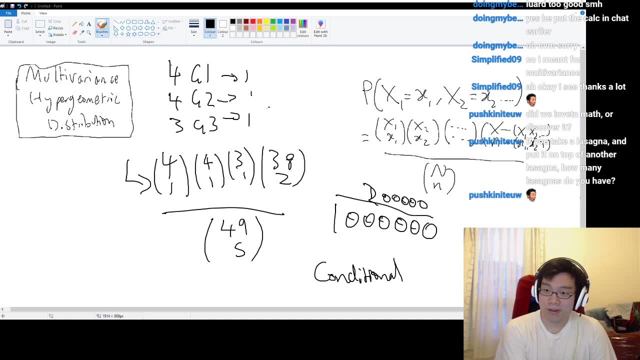 where x is the number of sub-lasagnas within the original number. But yeah, that's kind of the basics. So the reason I wanted to do this on stream rather than making it video is mainly because, yeah, like. 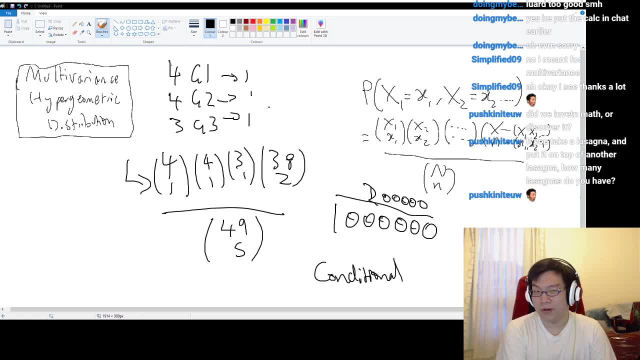 it took a while to plan how to even do the stream and I didn't even follow the plan accurately. you know, I free-formed all of it and made a mistake here and there, and it would've just been a huge amount of time and effort. 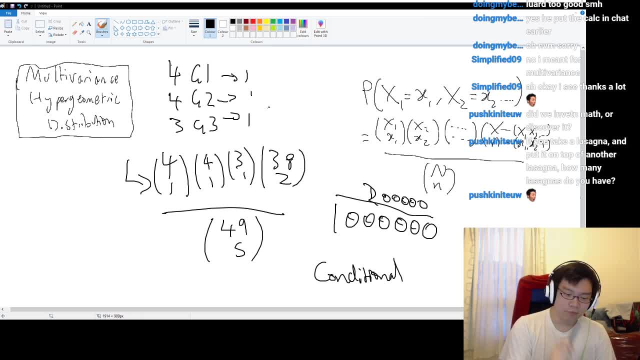 to both record, edit, fix, you know, double-check. I would've wanted to like generate a bunch of images instead of like drawing by freehand in MS Paint. I would've even had to highlight nice graphics and all of that. 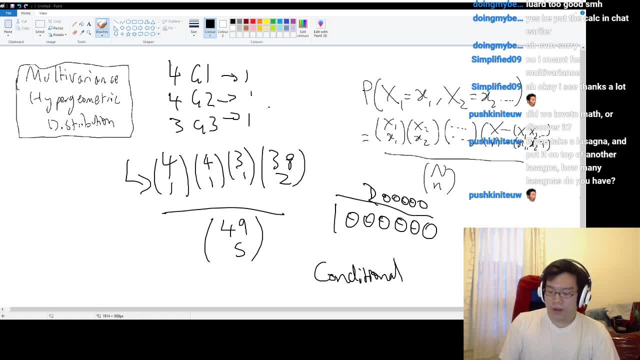 And I just felt that you know as much as I'd like to believe I helped someone today. it wasn't worth that much effort. Like this is Not to blow my own horn, but I think this was really useful for a lot of people. 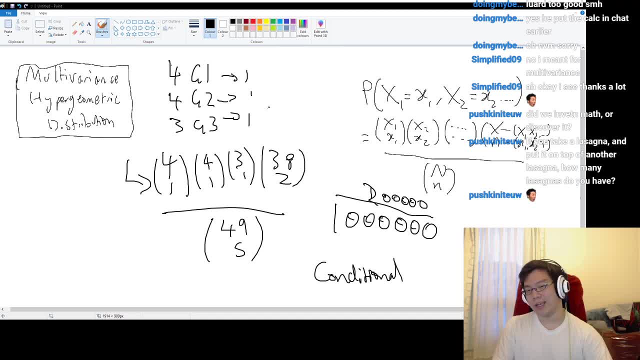 But I'd rather just get it out there as easy as I can, as quickly as I can for people to see. you know, I'd rather put effort into the more complicated things like fight videos and deck profiles and the Link Joker primers and all that stuff. 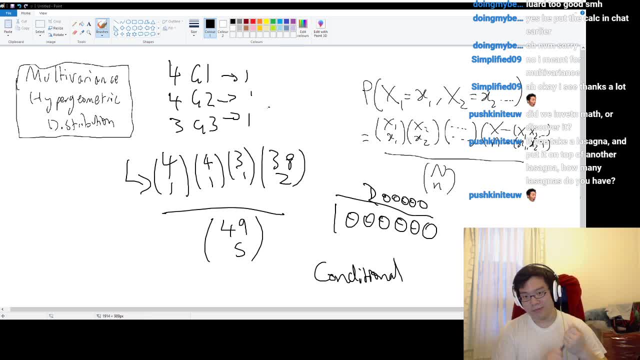 But yeah, This is basic statistics for card games, especially opening. you know, top X, whatever opening hands, whatever things like that. And again, it doesn't account for mulligan, because different games will mulligan in different ways. 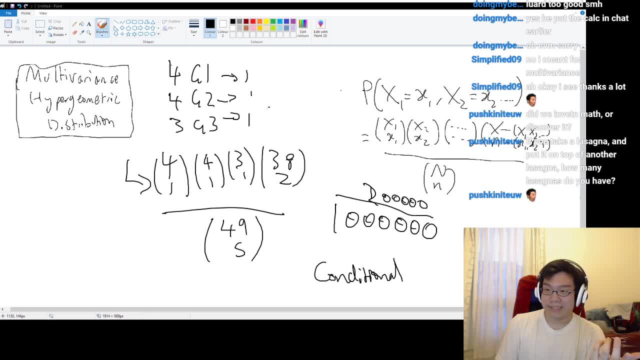 In fact, theoretically, Vanguard has the easiest mulligan to account for because it's You're not arranging the order of the deck in between hands, It's that you're looking at five, analyzing the quality of it, and then determine from there. 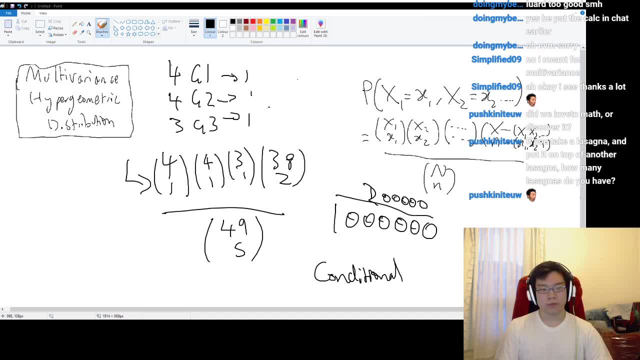 So, for example, if you want to open a domain of which you have, say, four domains and then 13 other grade ones, you could either have a domain in the top five but no grade one, in which case you would only look at the top four. 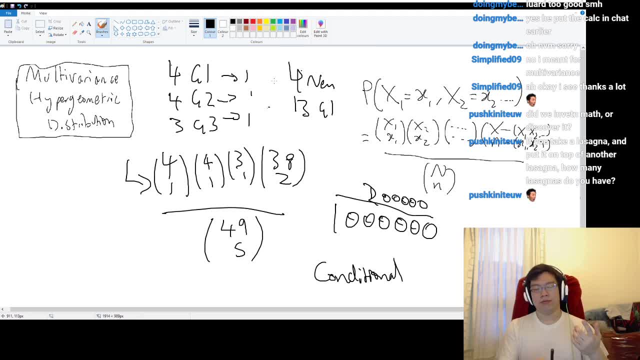 to find the other grade one or the other way around. You would have a grade one in the top five but no domain, in which case you put that in the other four. keep the grade one and then look at the next four for the domain. 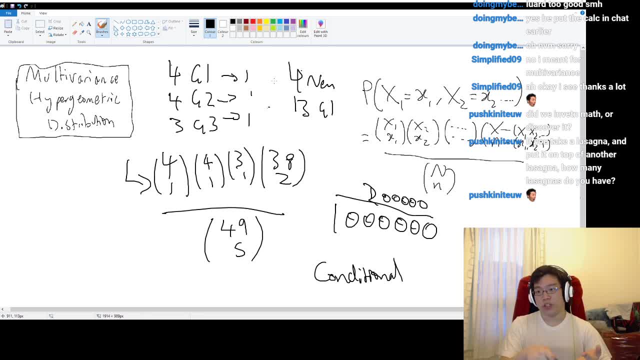 Or you have them both in the top five, in which case you don't need to stop there, you don't need to mulligan. Or you have none of them in the top five, and then you mulligan all five. 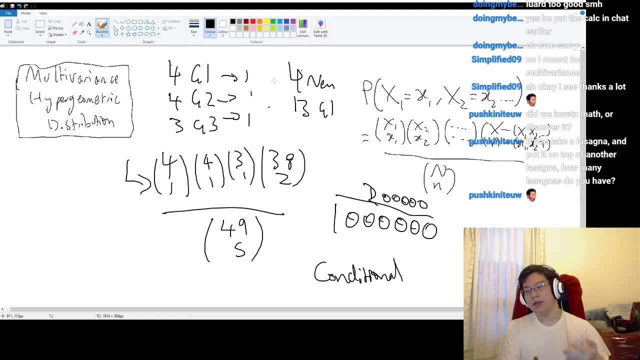 to find the two again in the next top five. So the numbers change a little bit more, especially because you put them on the bottom. so those four or five cards that you took out of the system you technically don't introduce because they literally cannot come up again. 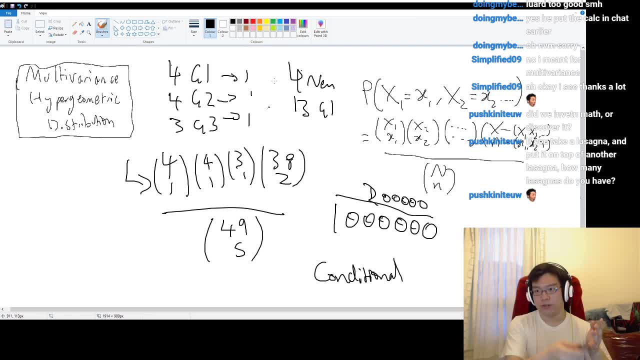 That doesn't mean that you might not draw the same copies or different copies of those same card. it just means that those specific objects are out of the set. in terms of insofar as this 49 by 5 goes, it becomes: 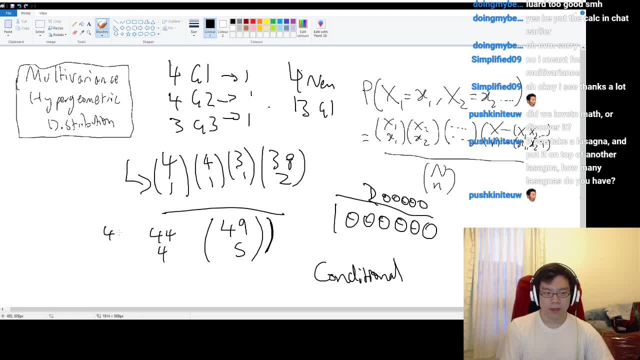 you know 44, 4, or 45, 4, or what have you, And then you know it kind of like draw for turns, start a ride and draw stuff like that top fives. 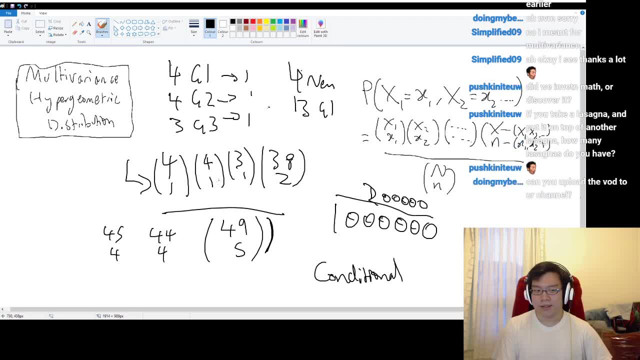 like it changes massively after that, but this is just a very basic sort of simple here and there Can you upload the VOD to your channel. Yes, I will definitely put this VOD on my channel, probably tomorrow morning. 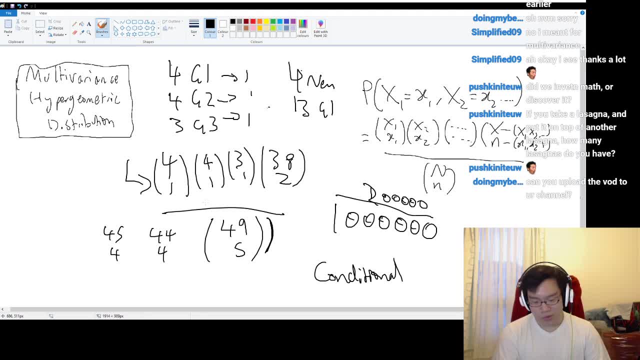 or something along those lines. see, That's the other reason I didn't want to make a video out of it, because if I stream it, then I can just upload the VOD and I don't have to do any editing whatsoever. 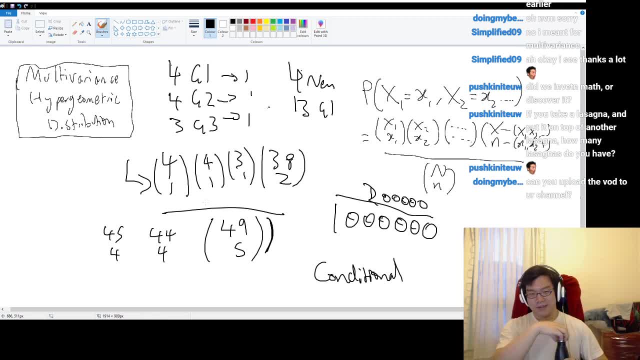 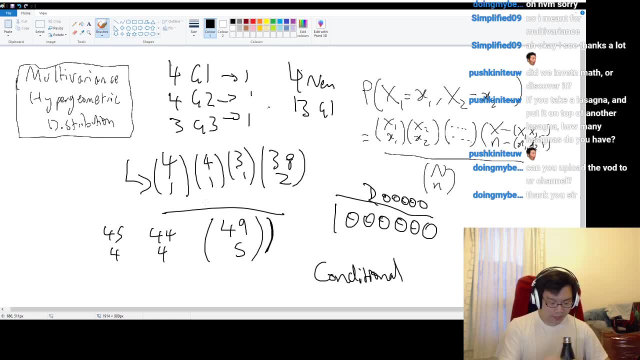 Very good, But yeah, that's been. ooh, how long are we? It's only been an hour. wow, we're ahead of time. I was expecting to take an hour and a half. brilliant, But yeah, that's been that. 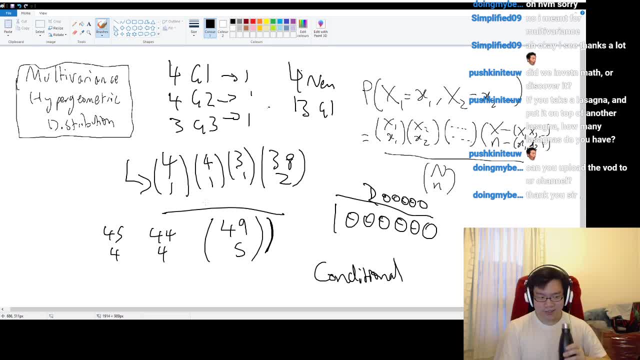 if anyone has any questions relating to this, feel free to drop them and I'll see if I can answer them otherwise, and that will pretty much be it. thanks for watching. Let me know if you did find this useful, like. 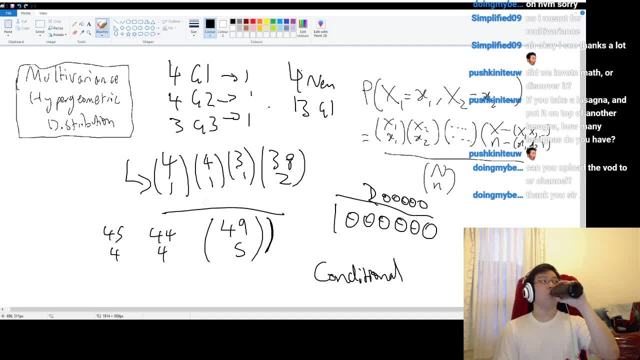 I've very much enjoyed it and I'll see you in the next one. bye, I've very much enjoyed doing these sorts of teaching sort of materials. the weird thing is that there's not very much other high level theoretical stuff that you can apply to card games. 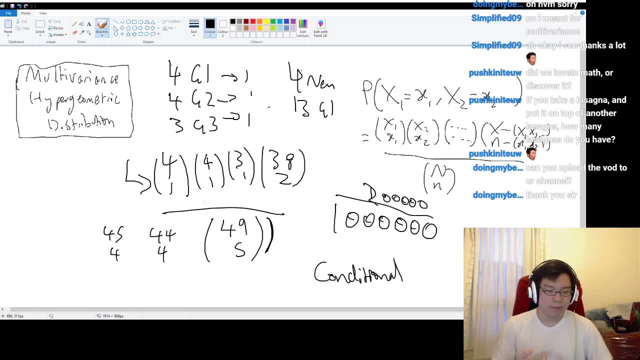 like things like evaluating cards, deck building theory, meta analysis, things like that. they're all very specific topics, like it's all very card game specific things, so it's hard to really account, it's hard to explain. 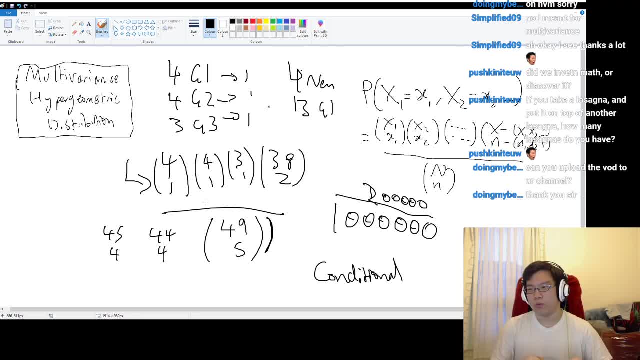 unless you already know a lot about the card game in question, which is why I kind of want to avoid stuff like that. but you know, if there's any other like abstract-ish concepts, concepts or theories that you'd like to, 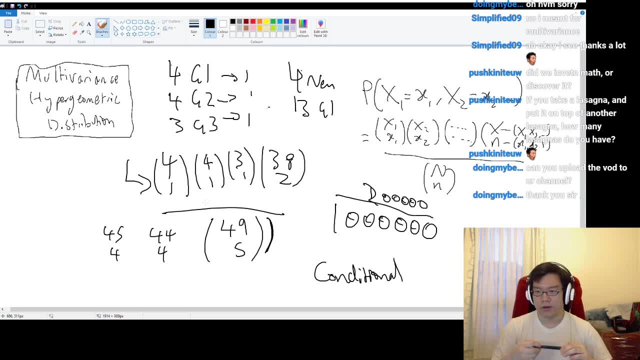 you know, see me cover, let me know. you know, drop me a line on Twitter, drop me a line on Discord or whatever. send us, you know, leave a comment on YouTube or whatever, and you know, we'll see if we can get around to it. 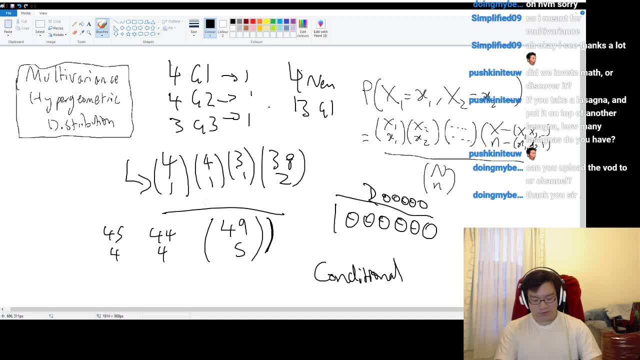 That's pretty much been it, but yeah, this was actually quite fun to do. got to plan a lesson and got to dig out my tablet. after you know years of osu abuse, Yeah, this was actually pretty fun to do. 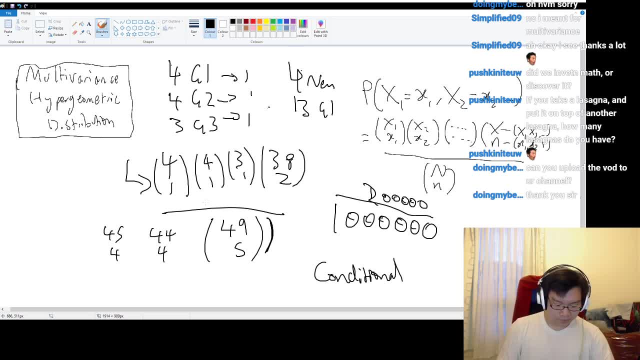 so again, hopefully you guys found that useful. uh, you'll understand now why you play Superior Raiden in Luard: because you're so likely to hit it and it offers you so much things like that. So, okay, yeah. 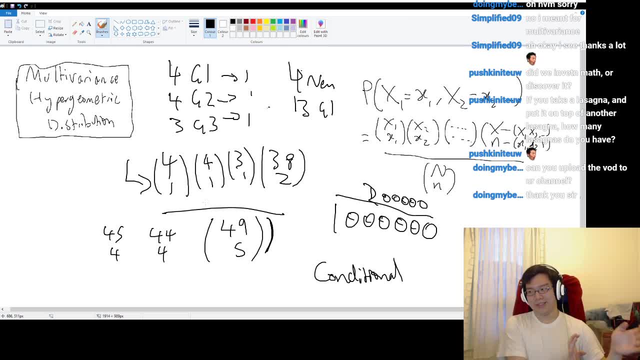 to talk back about Luard for a second. this is only half the argument, right? The consistency is only half the argument. The- how good is it really like? how game-winning is it? That is much harder to quantify, for obvious reasons. 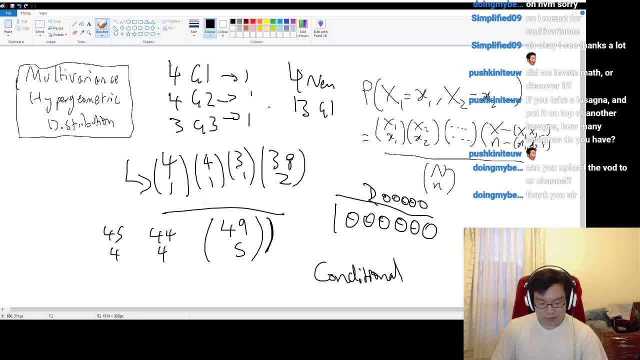 but you know it is. that is something else I think we could probably teach, but I'm probably not gonna plan to put something out like that for a while. So sorry, but you know it's. it's a much more abstract concept. 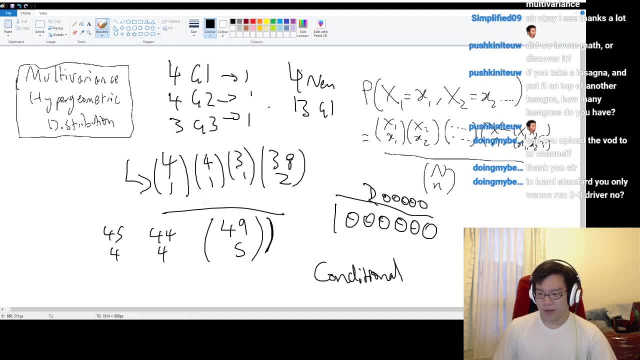 and I had to have a hard time conceptualizing it. In Luard's land you only want to run two or three driver. Yeah so, but that's another. that's a separate story. I meant the Phantom Blaster Superior Raid. 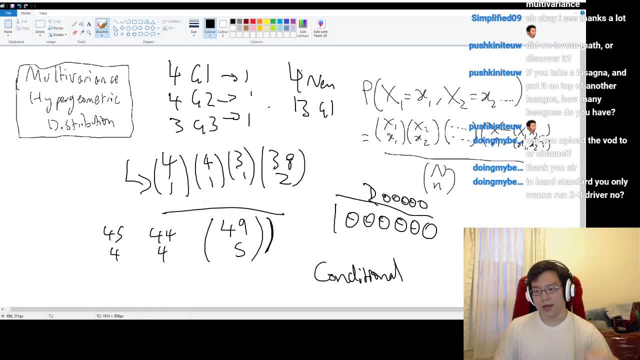 like you know, the chance of opening a Blaster Dark and in the main, or whatever, or the chance of opening Grade 1 Blaster Dark or Grade 1 Domain. there's a lot of ways of doing it. It's. 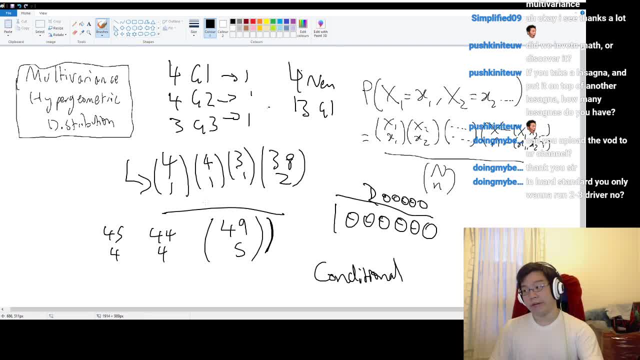 the Superior Raid in Luard means Superior Raiding to Phantom Blaster Dragon from Blaster Dark and then rewriting Luard after that. But that is a separate video altogether. I'm I'm still working on Luard in Standard and Premium. 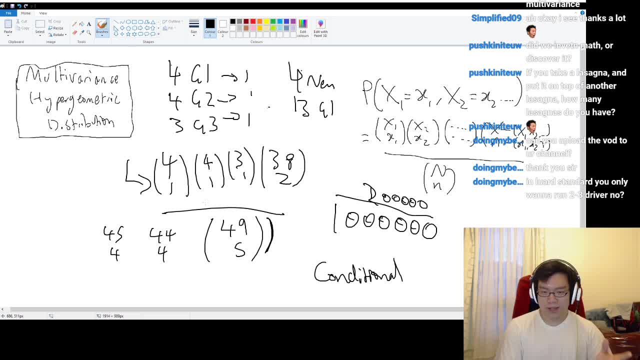 I'm still doing a bit of testing, trying to figure out what the list is. that is like. I know I haven't uploaded a video to the channel in like a month at this point after doing Bang Dream stuff, but I want to make sure that. 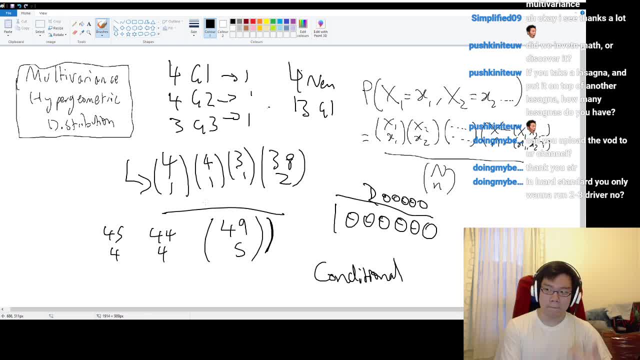 I want to make sure that what I'm presenting for Luard is A good and B correct before I do any further, but so I'm still working on like actually having a base level. I don't want to like. 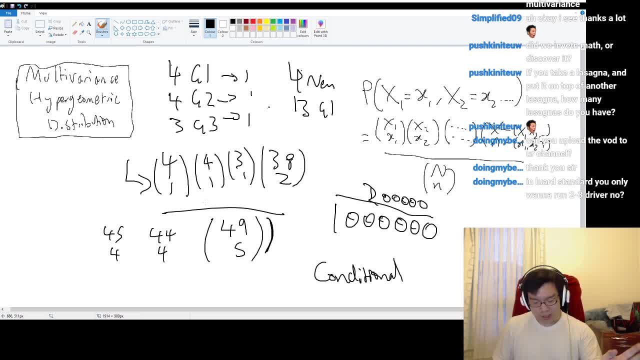 make a. I don't want to, like you know, I make lists and tweet them. like as soon as I make them, just like you know, tell people like: here's the idea I had, here's the rough idea. 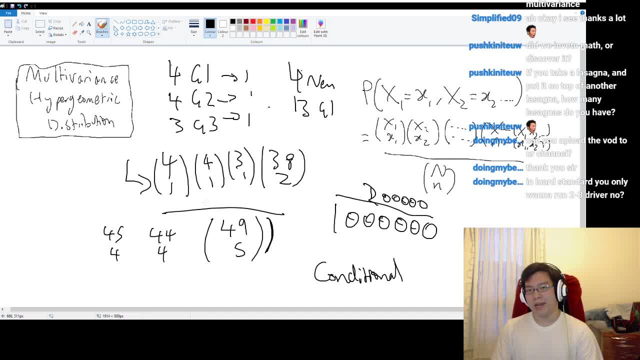 like this is where you can kind of go with it, But for stuff like videos, I really want to make sure that I have a good list before I go any further. It's actually I'm a video talking about every individual card. 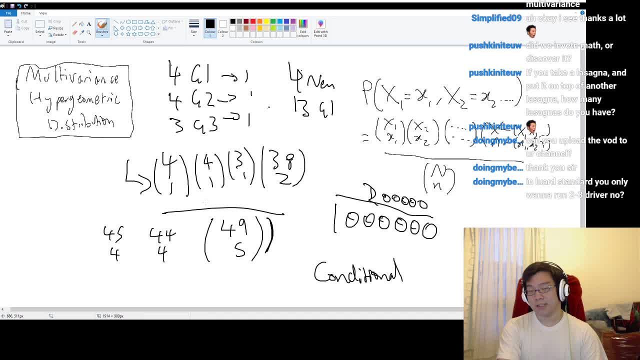 and why I think it's good or bad. Obviously, some cards have become better and some cards have become worse as the meta shifted since that video came out, but the idea is that, rather than just presenting a list and being like 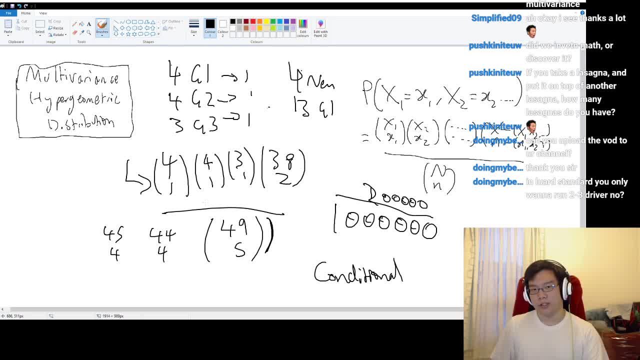 here's the list. I wanted to run like the deeper theory as to why cards are good, But with something like Luard I would much rather present a list, because I think the list, especially for Luard's case, where tech options matter a lot. 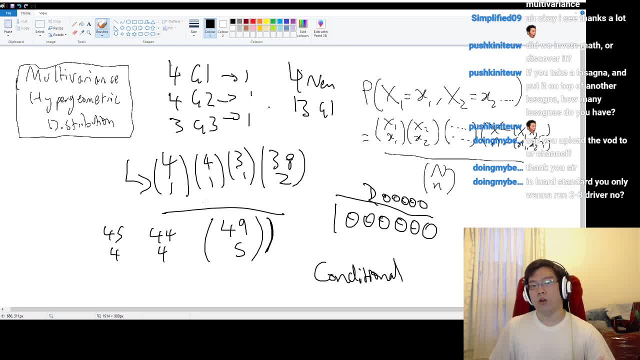 the individual choices you make make a factor in a lot more into what it does and compared to the overall concept of what the clan or the deck is trying to do. So when I make a Luard video, I really want to make sure that the list is. 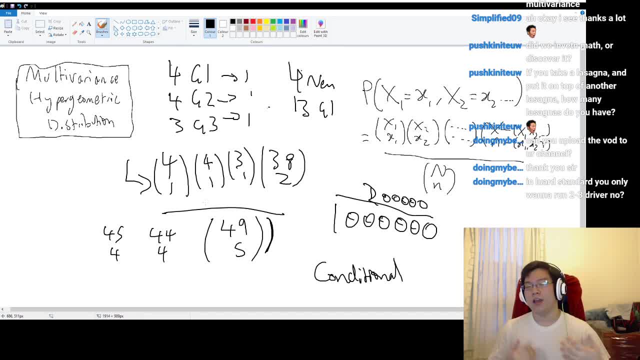 not the best, but as good as I could have made it before I present it, And I think that's probably going to take me another week or two at least, until I find something I'm happy with, like things like the number of Morphesser. 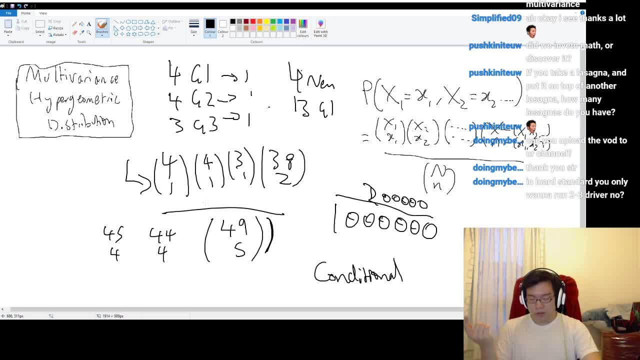 whether or not to play the one of Swordbreaker, which I do credit Nuno for talking to me about, like he has some pretty good arguments, which is why I'm experimenting with it. Things like playing the Grade 1- that gives you all the Grade 1's intercepts. 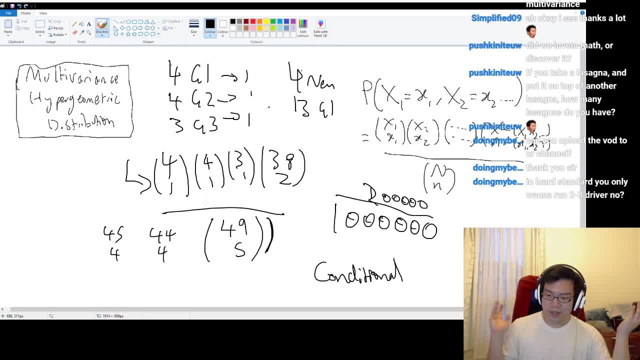 a lot of people are playing that. I don't like it, but you know, it apparently is decent. Like all this stuff, I still need to really, like you know, run through an experiment. And while we're on the topic of statistics, 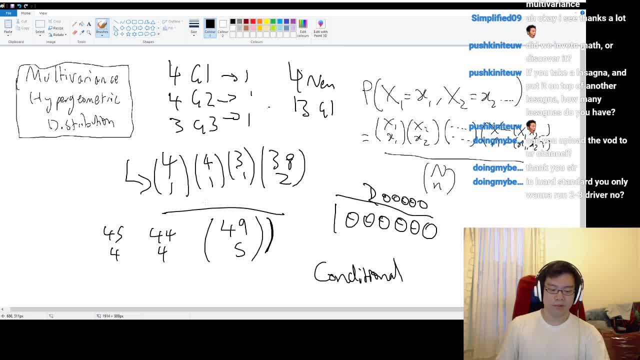 one of the other things I want to mention very quickly before I end the stream. when I when me, or StrictlyBroke or any of the guys that I experiment with, test stuff, we don't just play two or three games. 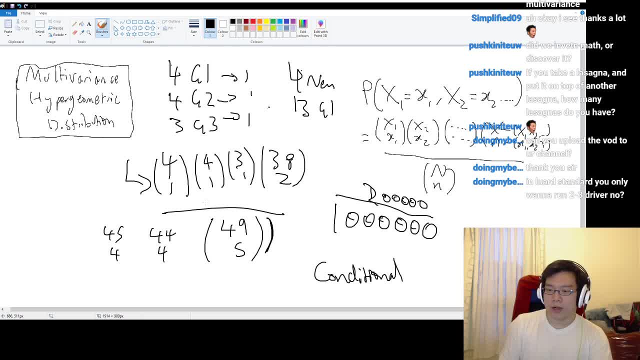 we're playing. like you know, we only stream like an hour at a time or two or three hours, which is only like four or five games, but we're playing a lot more than that Like. we're playing, like you know. 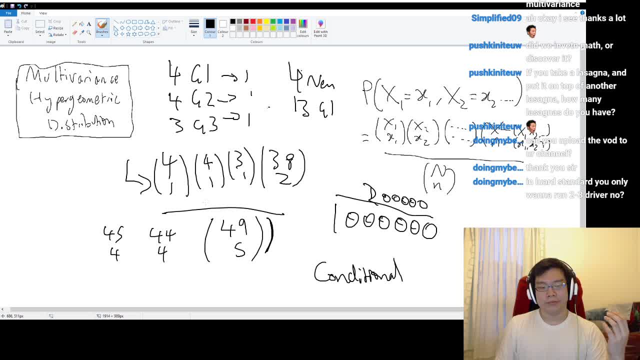 ten games a day, like across two or three days a week, because it's all about statistical significance. Like you saw that, the numbers tell you that you're 80% favoured to ride in the main or to open in the main. 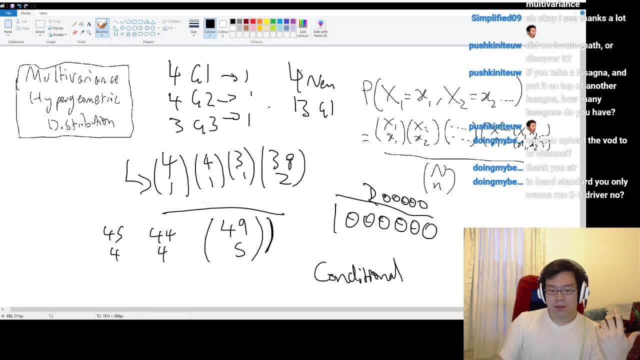 and have a Grade 1 ride on turn one, But they'll be, you know. so 80% chance is four out of five games or eight out of ten games, And sometimes you'll play three games in a row where you don't see any in the mains. 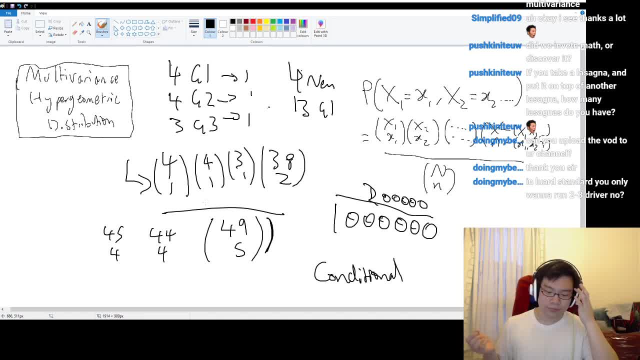 or you'll play, you know, six games in a row where you don't see any in the mains. And just because that small subset you got unlucky doesn't detract from the statistical significance of being correct, And so that's why you want to play as many games. 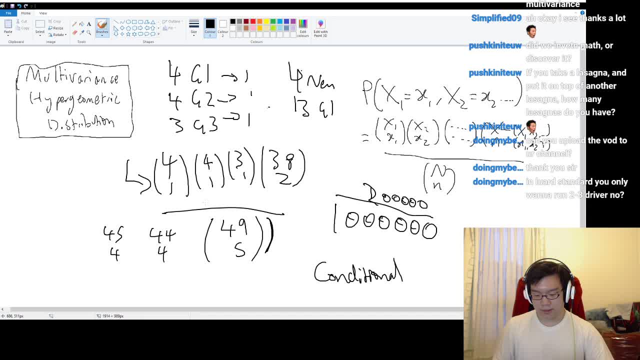 as physically possible to ensure that it's statistically significant. Like you know, if you say it's 50-50 to flip a heads or tails and you flip three heads in a row, that was only a 12% chance to hit it. 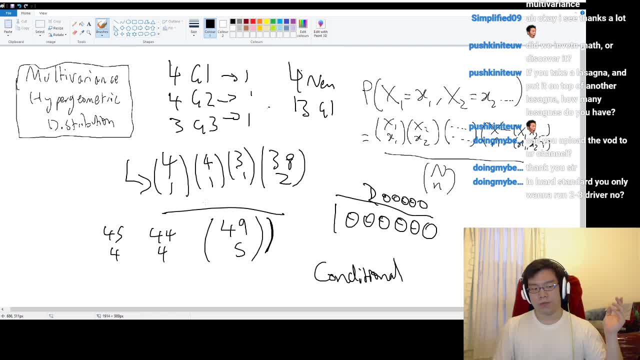 But that's still, you know, probability. Like you can't just say: oh, it's 100% chance to always flip heads. You need to flip a 30% chance to flip 1,000 coins and see, you know. 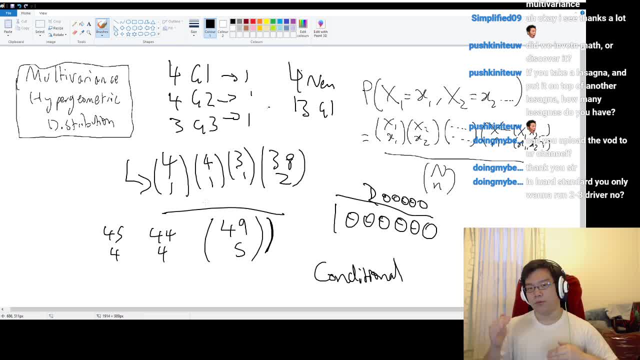 And after flipping 1,000 coins will you get you know, like 450, 500-ish heads or tails either way, And even then there'll still be some wiggle room. So, yeah, that's the final disclaimer for this video. 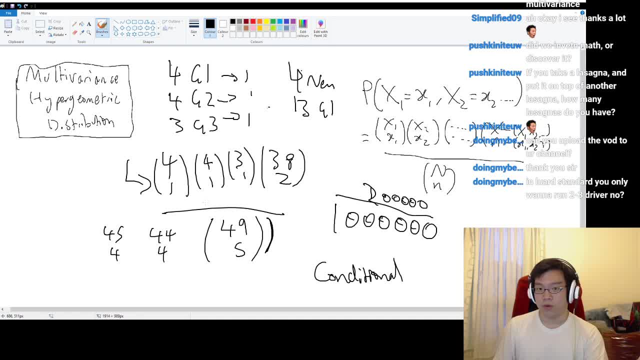 if you're watching this on YouTube, or your final disclaimer for the stream if you're watching it on stream, that everything here, all of everything regarding theoretical statistics and probability and all that, is all theory. It's not reality. You're never gonna be exactly on percent. 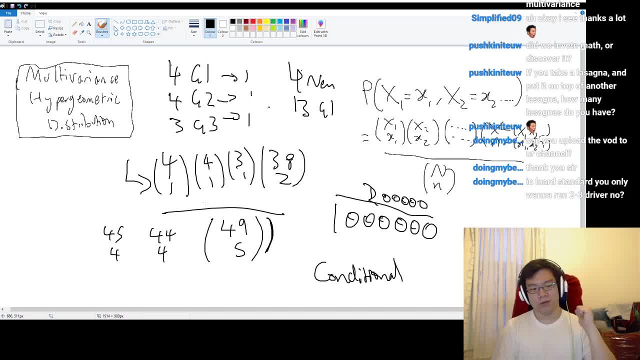 You're never gonna be exactly on expectations Numbers. numbers are only a guide and an estimation to what reality is. So take everything here today with a pinch of salt. So that's been it for me for today. Yellowcard Vanguard. Thank you very much for watching. 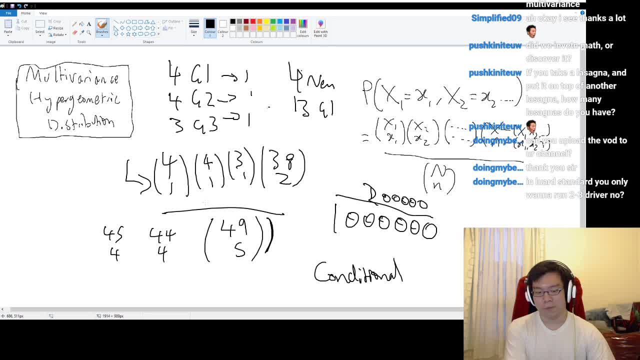 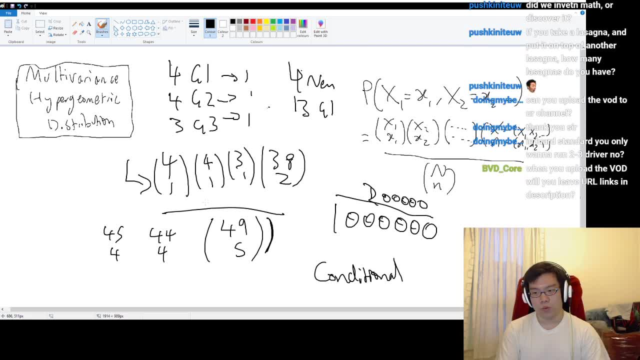 And, as I said, as always, hopefully someone finds this useful. More content coming very soon, hopefully, more like this. As always, feel free to leave a like, subscribe to the channel, leave comments, see what you wanna like, what you wanna see more of. 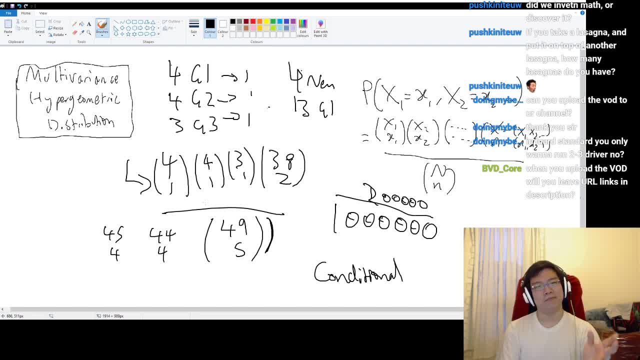 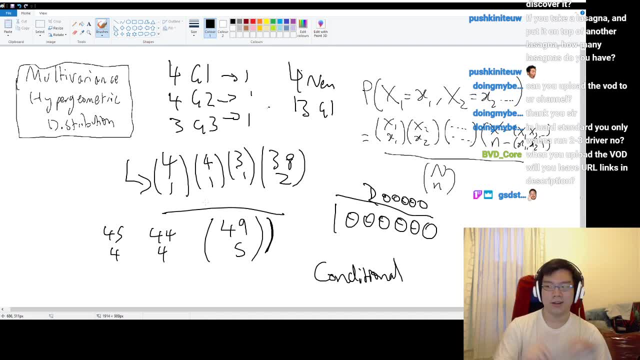 And, yeah, hopefully we'll see you guys next time. Buh-bye, Will you upload the VOD and leave your? I definitely will. Thank you for reminding me. Yes, So links to StatTrak, links to Wikipedia and all this stuff. 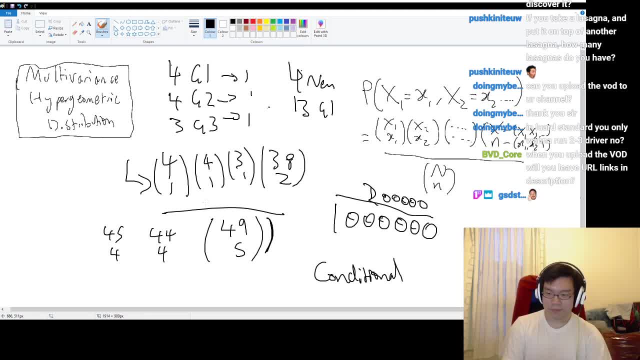 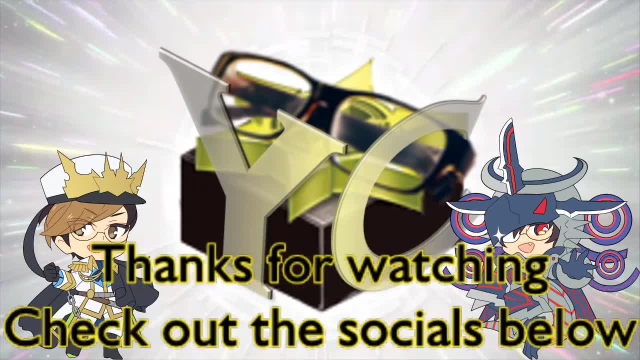 they'll be in the video description as well. But yeah, thanks for watching, guys, and hopefully we'll see you all next week. Buh-bye, Bye. 4.